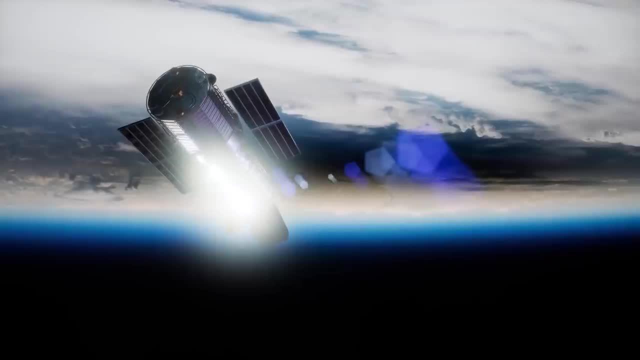 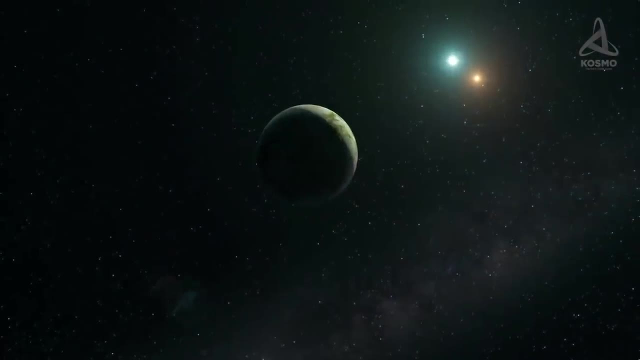 The first exoplanet in outer space. The first exoplanet in outer space. The first exoplanets were discovered back in the late 1980s. Since then, the number of detected ones has increased hundredfold. According to statistics, from January 2021, over 4,000 planets. 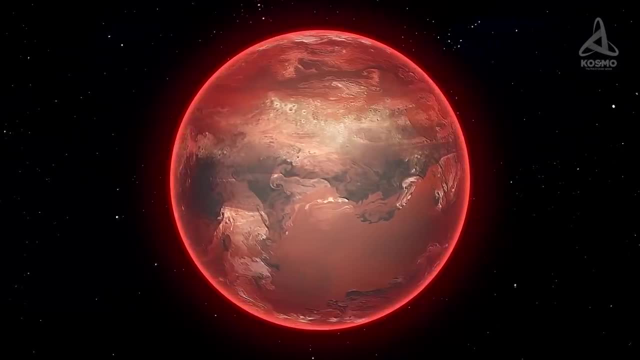 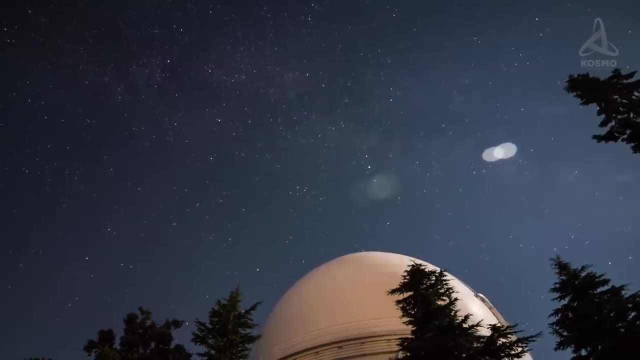 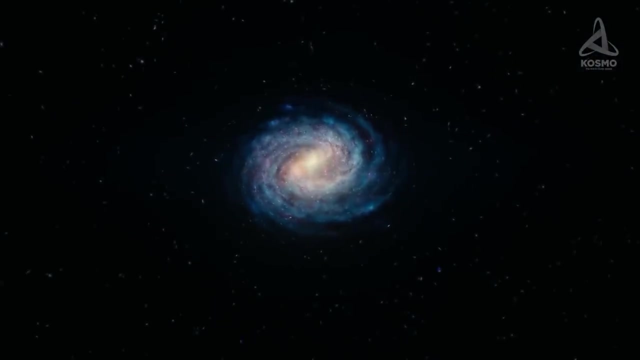 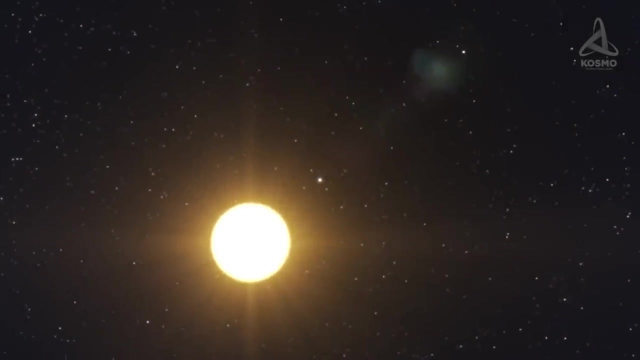 in other systems have already been discovered. Apart from these, several thousand candidates likely to be given this status have been registered With sufficient evidence from Earth-based observatories. most of them are going to become officially confirmed exoplanets. The overall number of planets in our galaxy may supposedly be over one trillion, From 5% to 20% of. 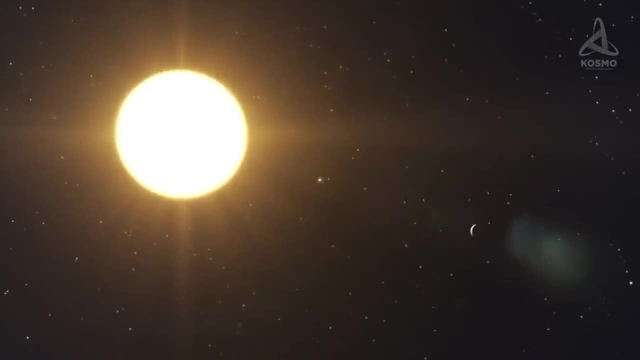 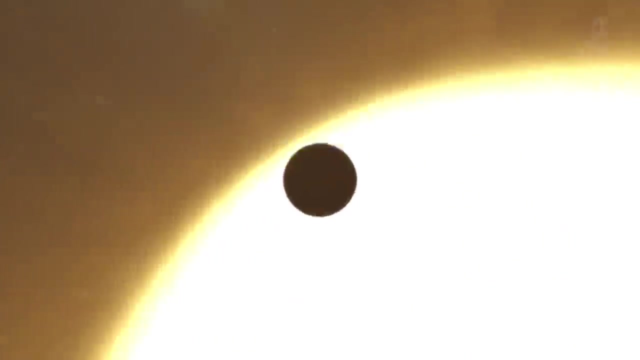 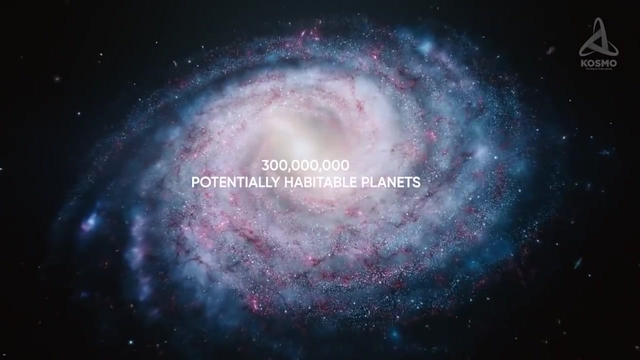 these are close to our Earth in terms of their size and composition. Not all of them are in their host star's godelock zones, that is, not all of them are habitable. Still, according to scientific estimates, there are not less than 300,000,000 potentially habitable planets in the Milky Way. 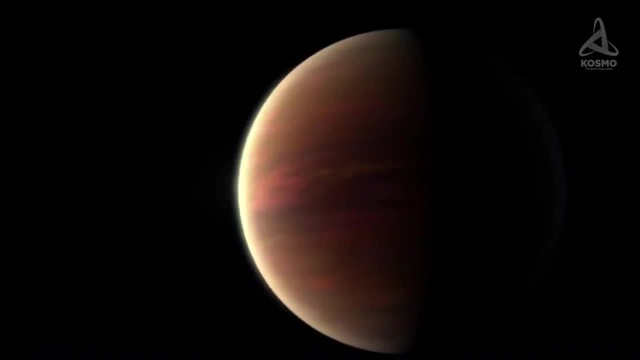 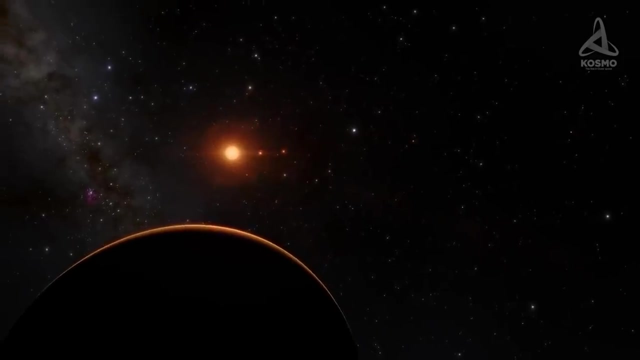 Exoplanets differ in their own own size and composition. The exoplanets have different differ very much in terms of their environment. Their dimensions may be enormous, some even beating Jupiter, but there are also comparatively smaller ones, close to our Earth in size. 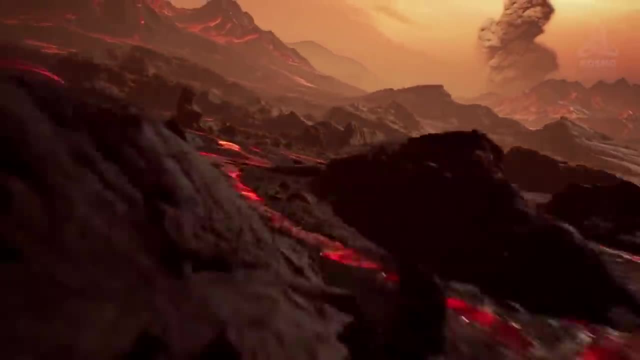 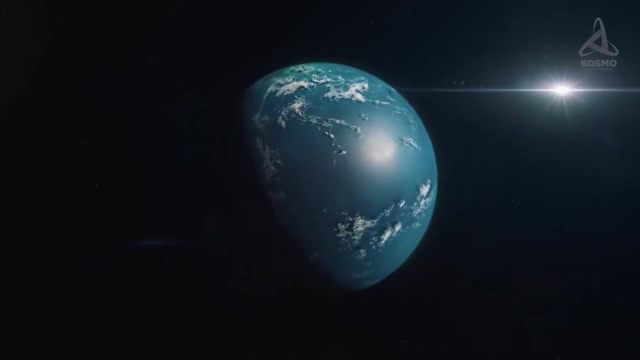 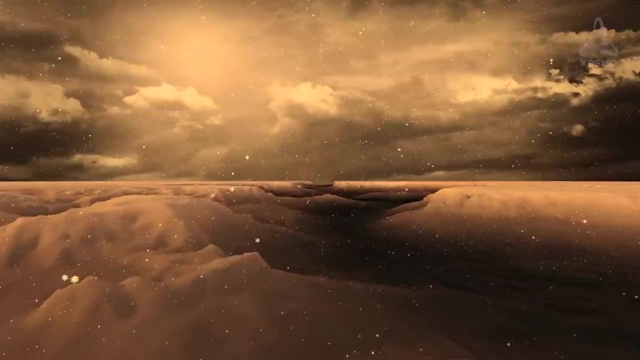 Some of these bodies are hot, consumed with oceans of molten lava, whereas others are encased in a shell of permanent ice. There are planets out there made entirely of oceans, with not a bit of dry land on them, while on others, sulfuric acid rains or diamond snow are a regular occurrence. 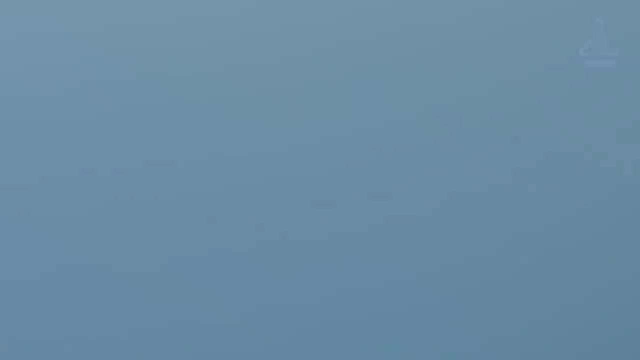 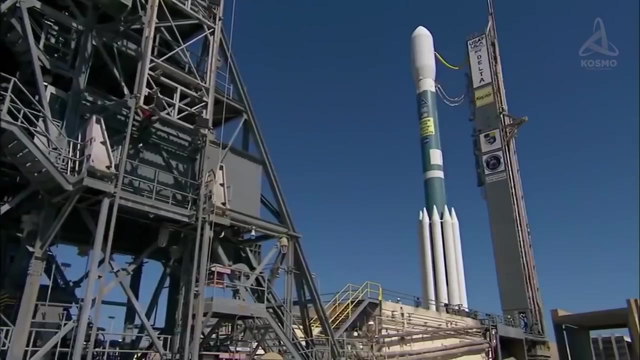 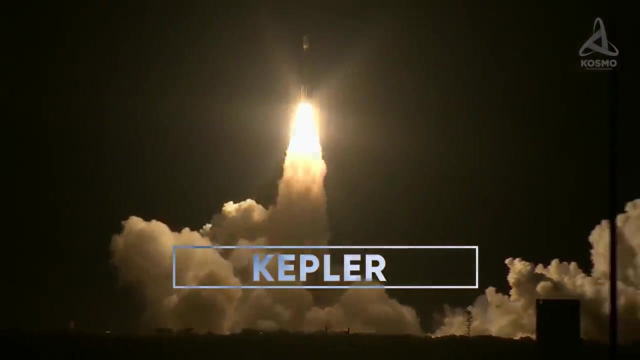 Various techniques are used for discovering other worlds. As a rule, it is next to impossible to spot an exoplanet by simply looking through a telescope. That is why, in 2009,, Kepler was launched, the first space telescope designed for searching for planets beyond the boundaries of the Solar System. 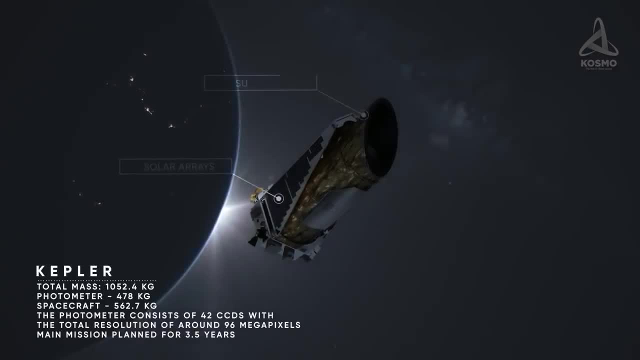 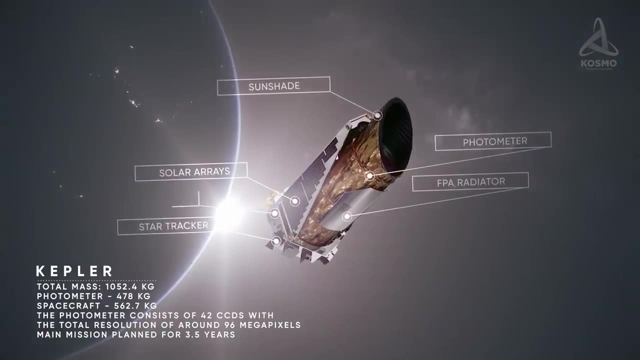 The telescope's cameras had 42 charge-coupled devices, Or CCDs, with a total resolution of around 96 megapixels, With a field of view covering about 25% of the sky, and coupled with a 1.5-meter mirror. 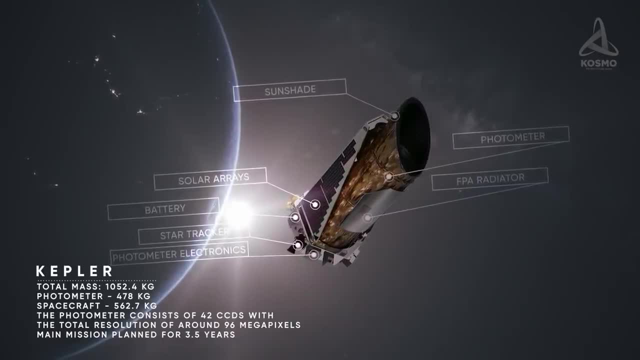 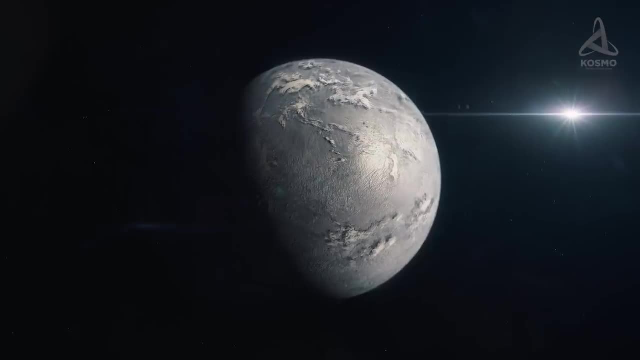 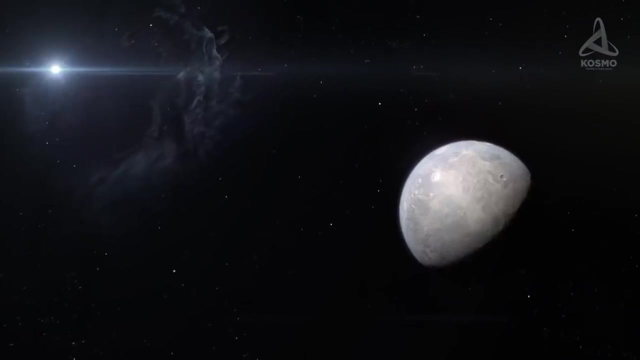 of the telescope, it was able to detect astronomical bodies within 3,000 light-years from the Earth. In the 3.5 years of productive operations, Kepler managed to spot over 3.5 thousand exoplanet candidates. The status of over 2,000 of these exoplanets is unknown. 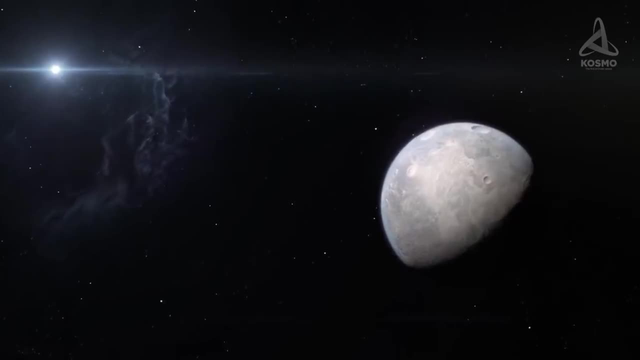 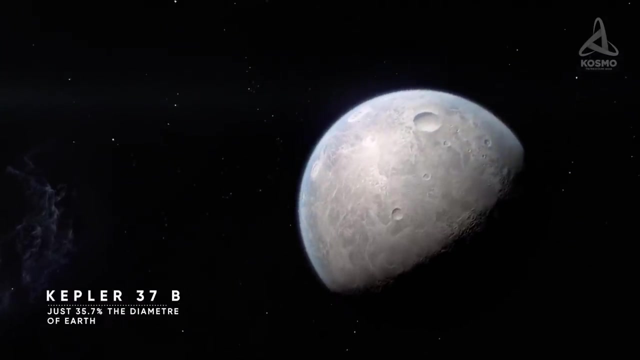 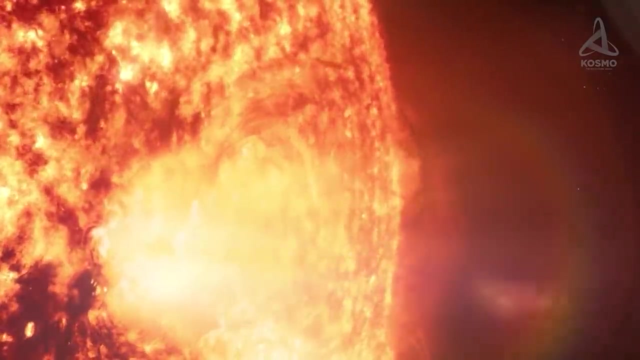 One of these has already been confirmed by repeated observations. It was in this period that the smallest of known exoplanets today was detected. The diameter of Kepler-37b is just 35.7% that of the Earth. The telescope was also instrumental in registering several stars and brown dwarfs. 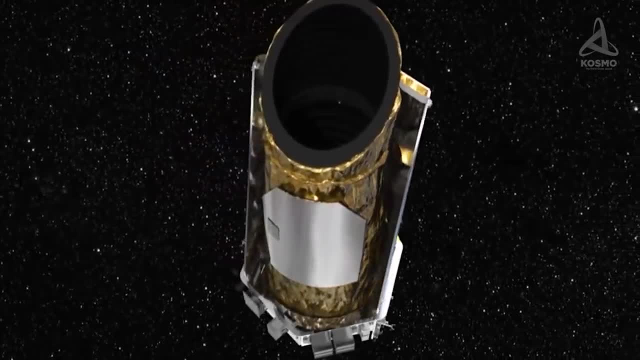 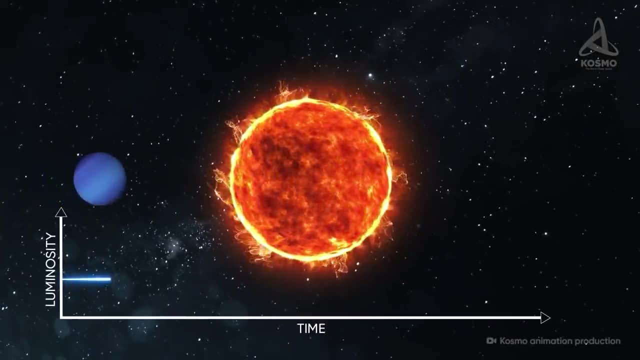 The transit method was used by Kepler in the search for exoplanets. This method is based on observing the star's luminosity. The telescope is based on observing the star's luminosity. If the supposed planet passes between the parent star and the observer, this will be: 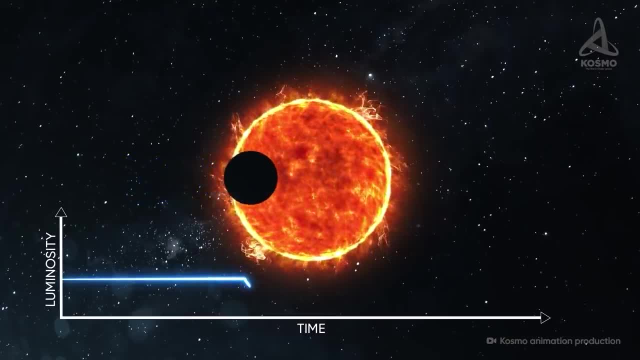 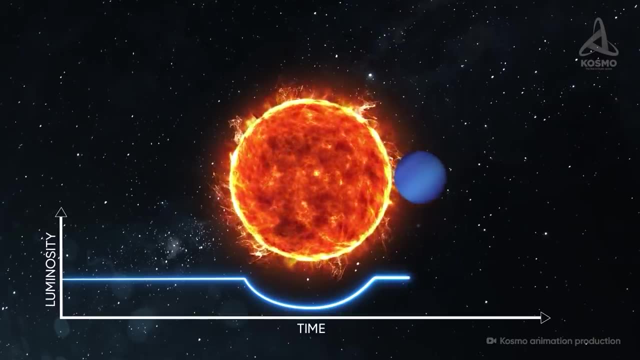 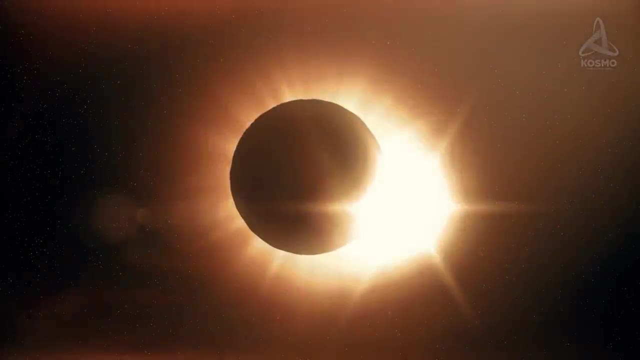 noticed in the telltale decrease in the star's luminosity. The extent of these fluctuations in luminosity directly depends on the ratio of the star's and planet's dimensions. while their regularity allows one to estimate the object's orbital period, The transit method requires accuracy in measurements. 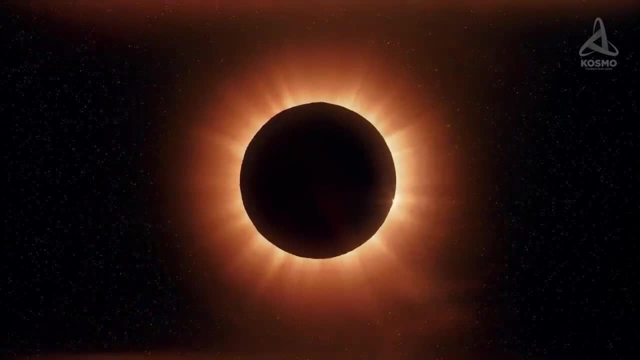 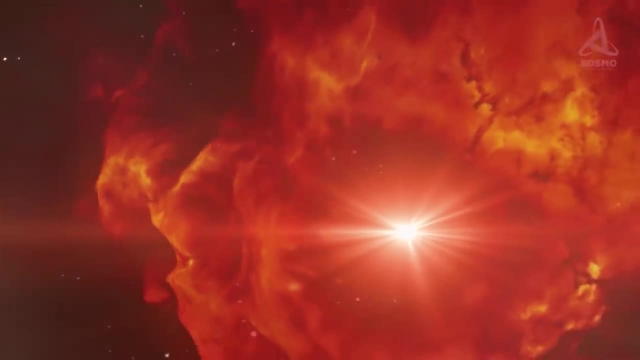 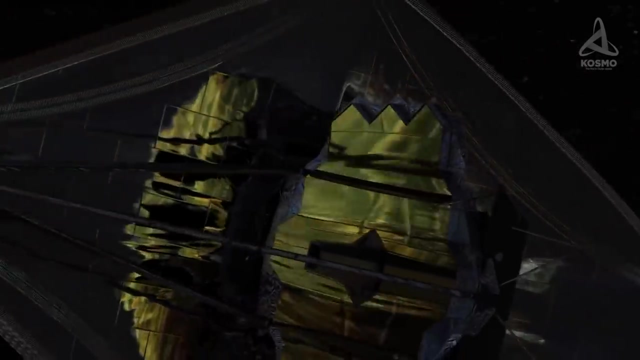 Changes in a star's spectrum account for less than 2 percent and are usually tenths or even hundredths of one percent. Ripples in the atmosphere, dust and precipitations negatively affect results produced by Earth-based telescopes. That is the reason why telescopes based on automatic space stations are used for searching. 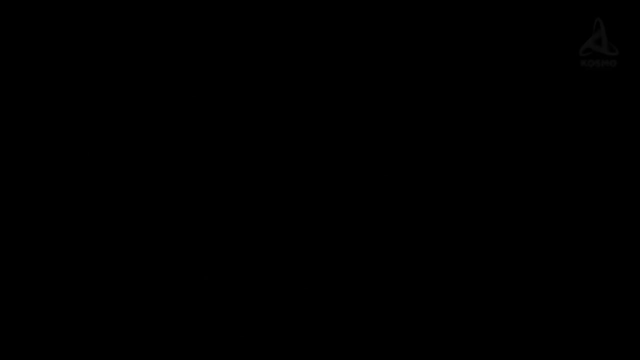 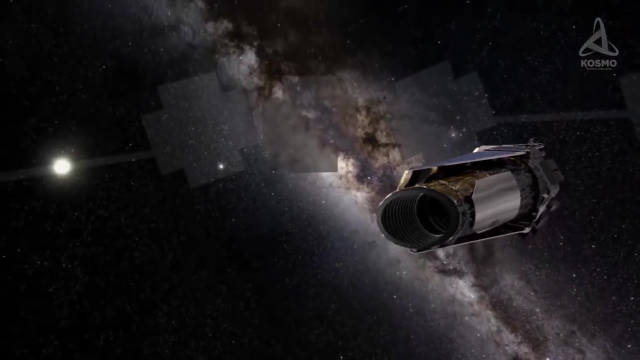 for objects beyond the boundaries of the solar system. Unfortunately, in 2013,, three and a half years into the mission, the Kepler Space Telescope had several major equipment failures. In 2018,, the Kepler Space Telescope was the first telescope to be used in the space space. 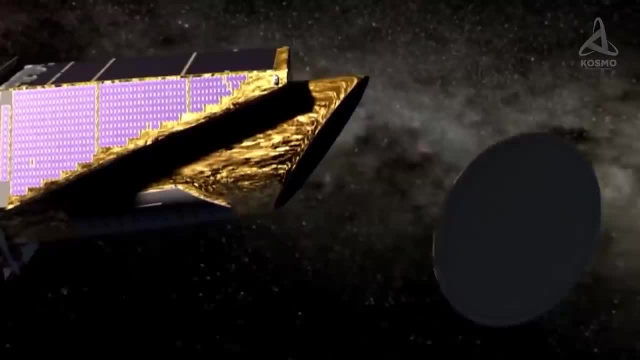 In 2018, the Kepler Space Telescope was the first telescope to be used in the space space. In 2018, the Kepler Space Telescope was the first telescope to be used in the space space. In 2018, the spacecraft ended science operations completely. 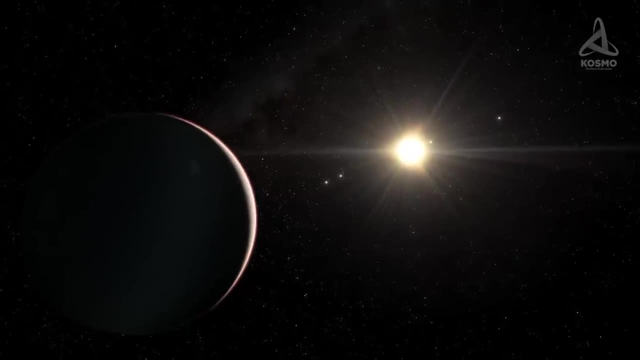 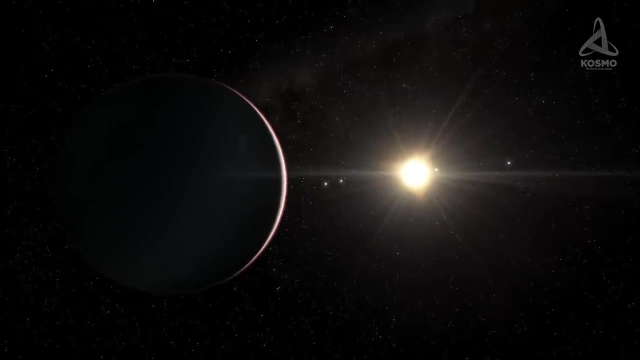 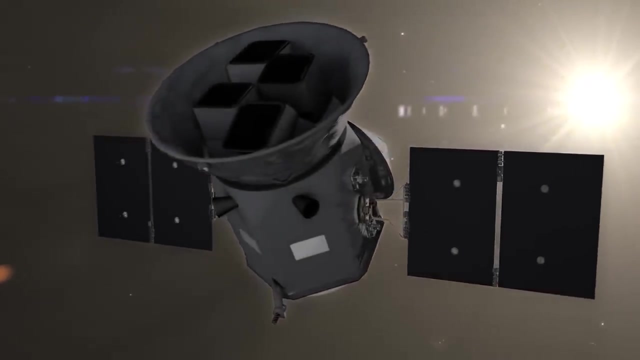 Kepler was the first spacecraft to be created specifically for looking for exoplanets. However, most of the objects it managed to spot happened to be too remote and dim to study them in any satisfying detail. That is why the next space research complex had slightly different parameters. 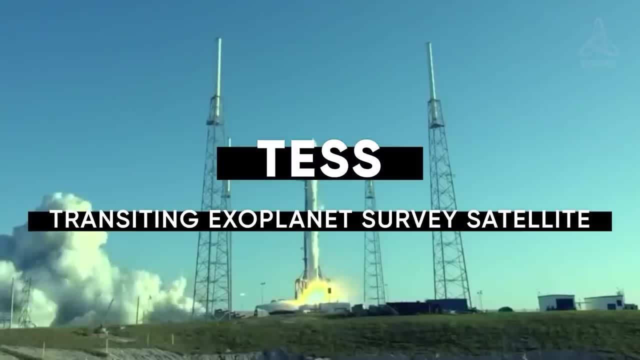 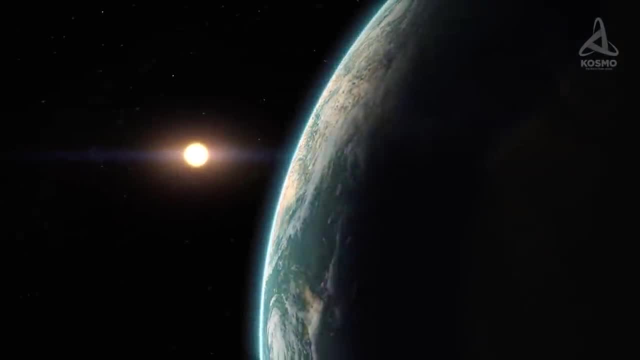 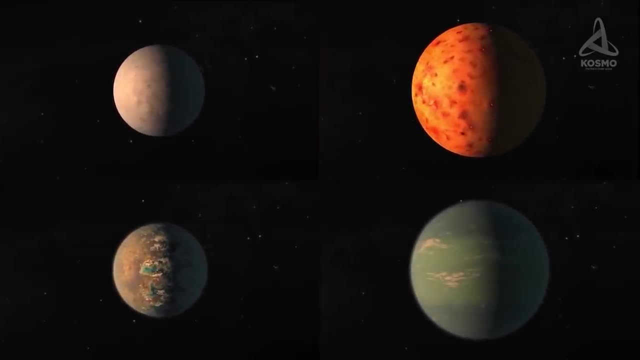 Kepler was succeeded by the TESS telescope launched by NASA on the 18th of April 2018.. Its main object was searching for rocky exoplanets orbiting the brightest stars within 200 light years from the Sun. This telescope also used the transit method. 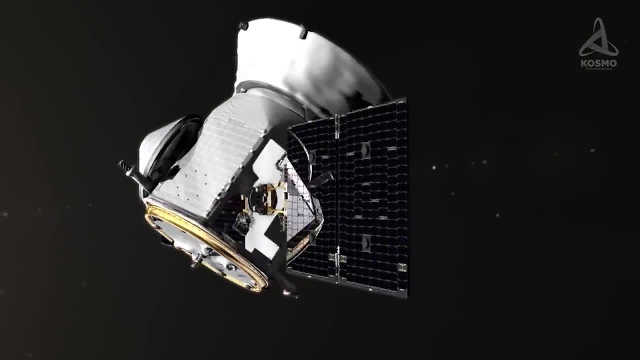 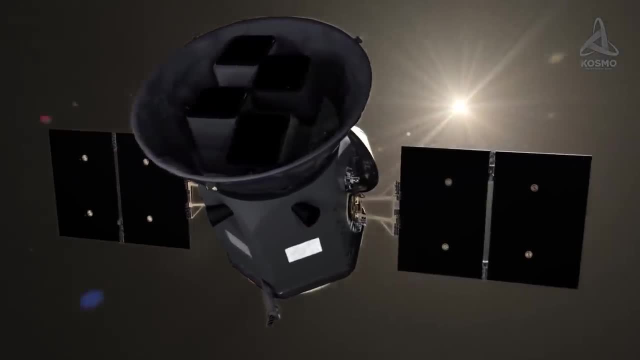 And here is the spacecraft's brief profile. TESS is equipped with four refractors with a 24 by 24 degree field of view and a 10 centimeter aperture. The spacecraft's peculiar orbit allows it to cover both the northern and the southern. 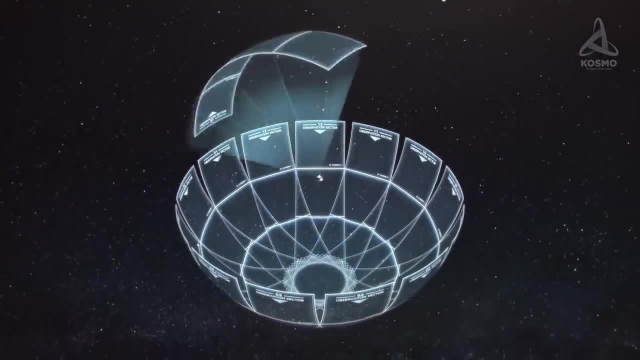 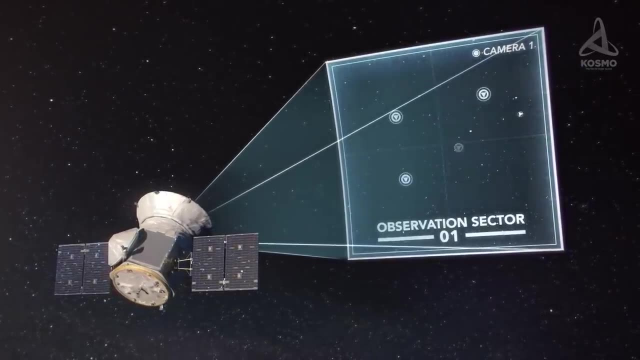 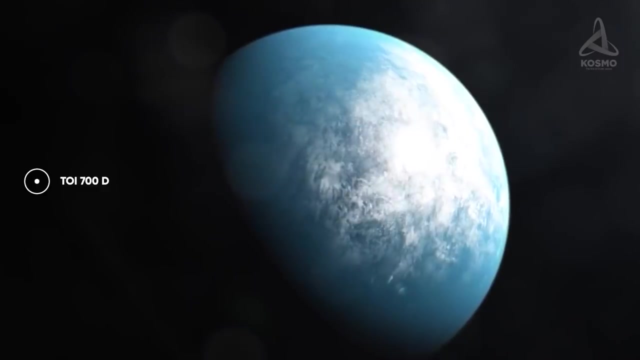 parts of the sky which is approximately 8 meters. TESS is capable of covering 85% of the entire sky. Photos are taken by four cameras and the resolution of each camera's CCD is 16.8 megapixels. TOI 700d is one of the most notable objects discovered by TESS. 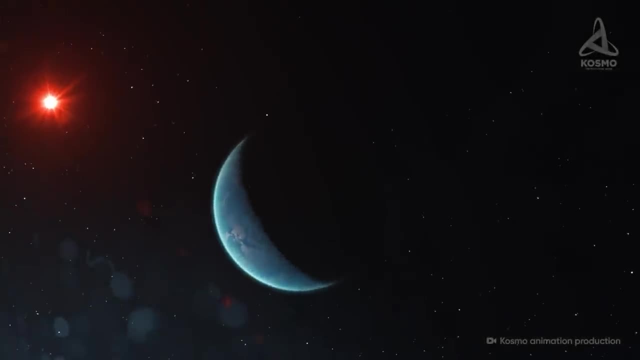 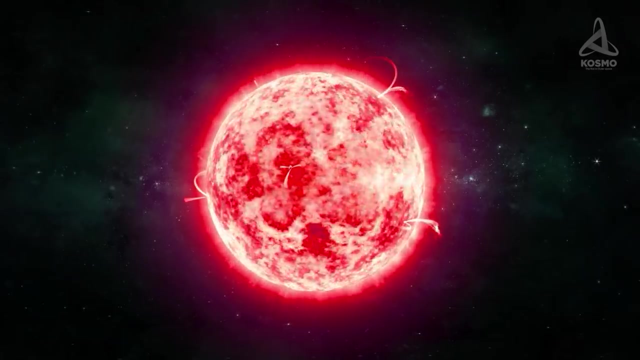 This exoplanet became the first object of the kind comparable to the Earth in size and which found itself in the habitable zone of its star. It orbits TOI 700d, A red dwarf lying slightly over a hundred light years away from the Sun. 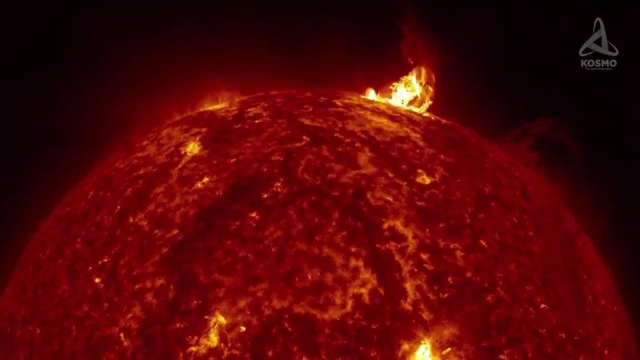 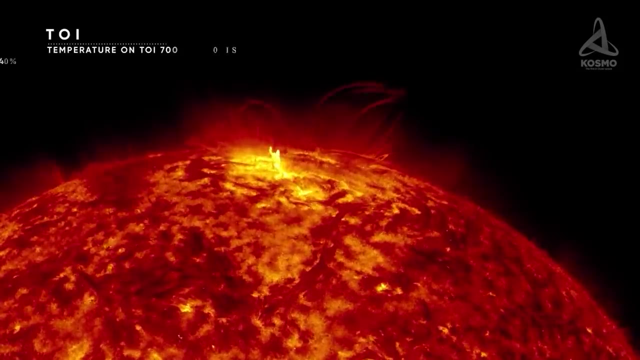 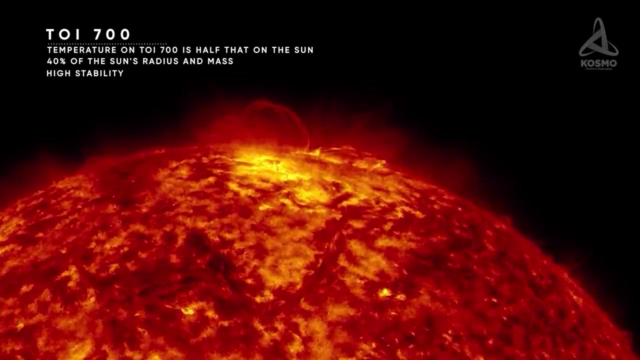 It is a small and rather cold star. Its temperature is half that of the Sun and its mass and radius are just 40% those of the Sun. TOI 700d is peculiar for its high stability. Not a single flare has been registered on it since the beginning of observations. 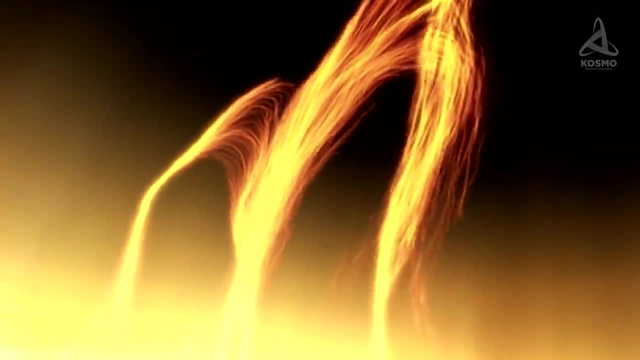 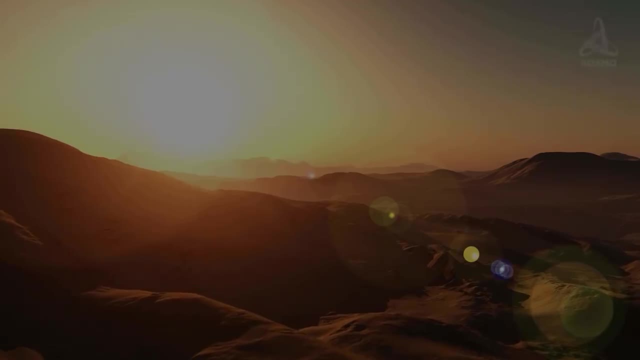 A star's stability is a positive feature. This is because bursts of activity are able to be observed. This is because bursts of activity are able to be observed. The bursts of activity are able to divert its planets of their atmospheres and be generally pernicious for potential life on planet's surfaces. 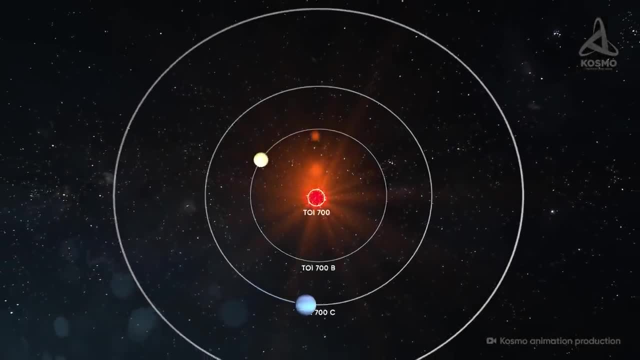 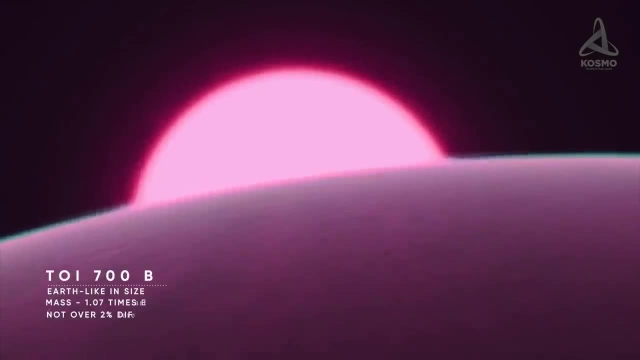 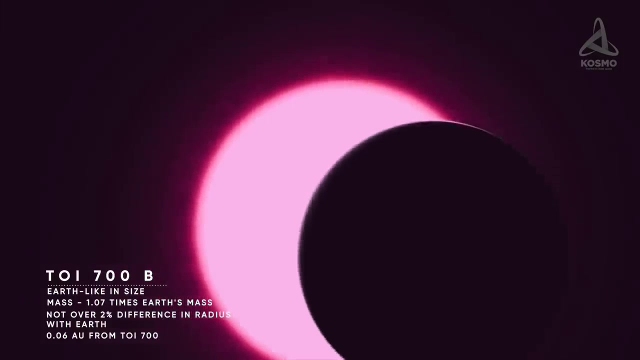 There are at least three planets orbiting TOI 700d, The one closest to it. TOI 700b is comparable to the Earth in size. Its mass is approximately 1.07 times that of our planet, and its radius differs from. 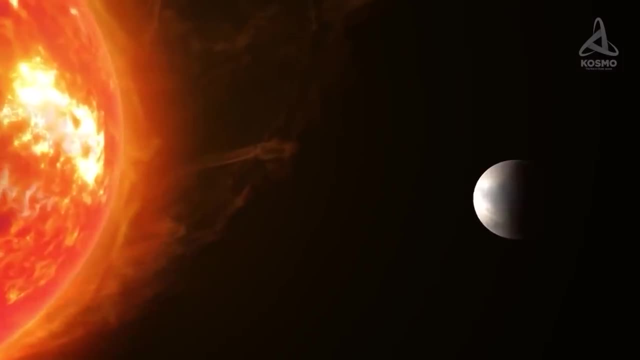 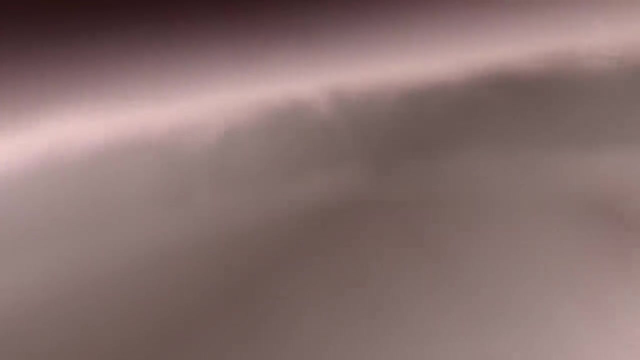 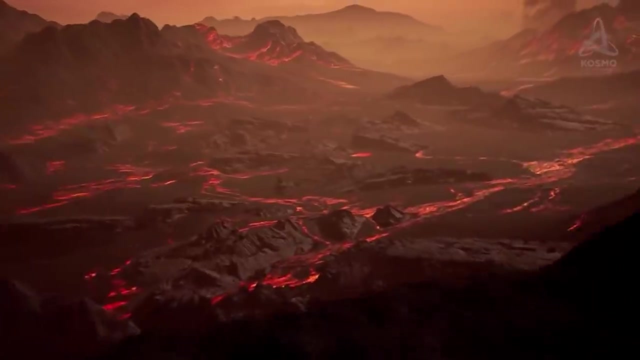 that of the Earth by not more than 2%. Unfortunately, TOI 700d is not a star. TOI 700 b is too close to its host star. It is within about 0.06 astronomical units, and a year on the planet lasts just 10 days. In addition to that, chances are it is tidally locked, that is. 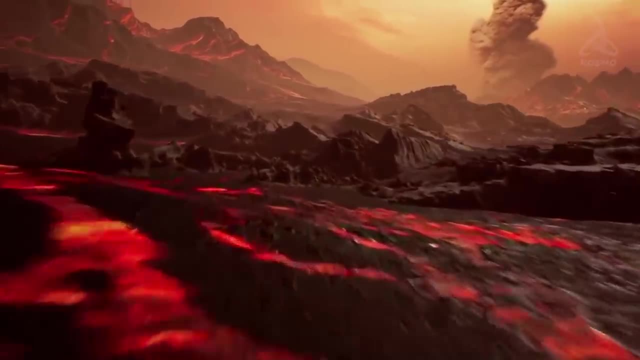 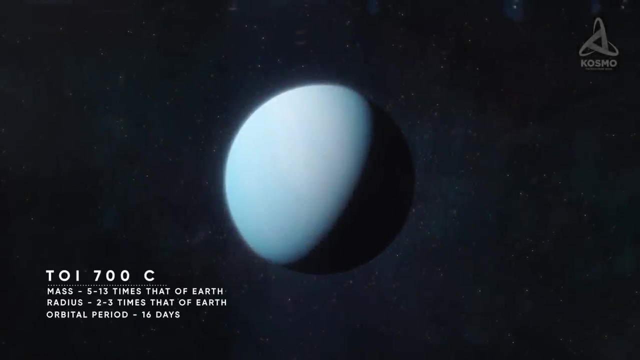 it faces the star with one in the same side. This means that the planet is likely to be scorching hot. The planet lying further from its star, TOI 700 c, is thought to be a mini-Neptune. Its mass 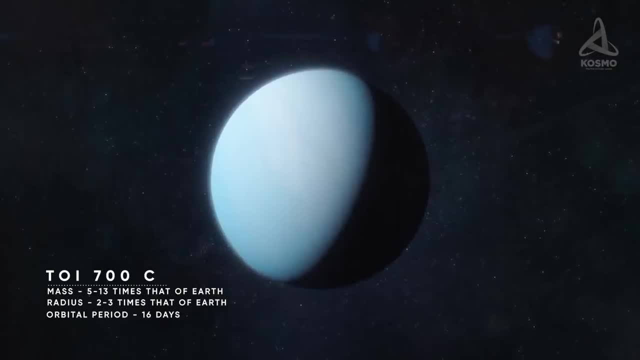 may be from 5 to 13 times that of our Earth and its radius is 2 or 3 times that of the Earth. It takes TOI 700 c 16 days to complete one orbit around its host star Located closer to the star. 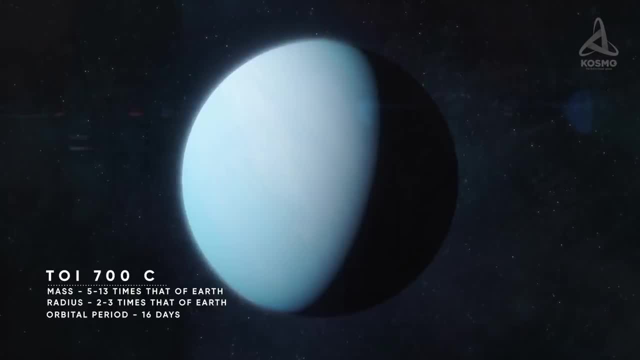 than the inner border of the habitable zone. it must be too hot for life to originate and evolve there. The planet is likely to be scorching hot. The planet lying further from its star, TOI 700 c, is thought to be a mini-Neptune. Its mass may be from 5 to 13 times that of our Earth and its radius. 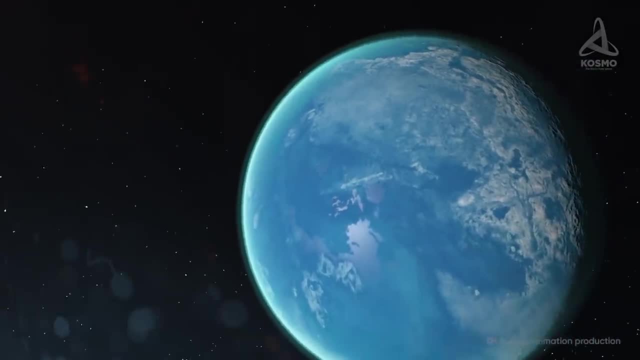 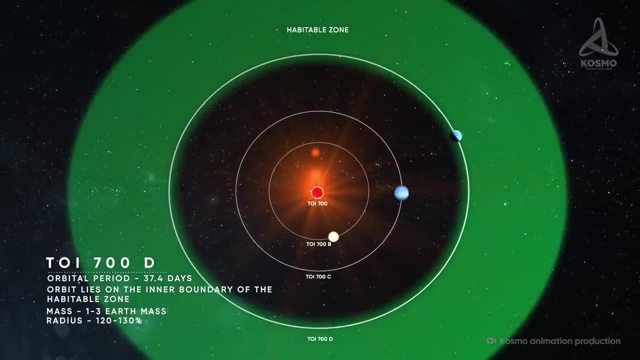 may be from 5 to 13 times that of our Earth, and its radius may be too hot for life to originate there. TOI 700 d is the third and, at this point, the remotest planet in the system discovered by now. It takes 37.4 days to complete a full orbit which, by the way, lies along the inner edge of the. 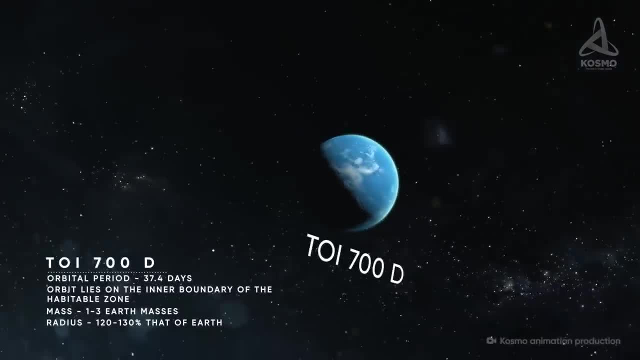 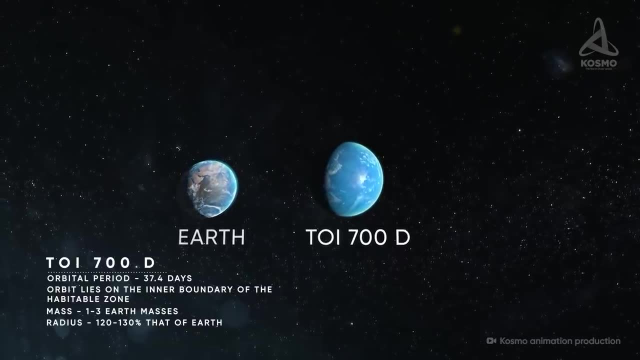 habitable zone. The mass of TOI 700 d hasn't been gauged precisely and may be anything from 1 to 3 times that of the Earth. At the same time, the planet's radius is just 20 to 30% bigger than that. of the Earth. The mass of TOI 700 d hasn't been gauged precisely and may be anything from 1 to 3 times that of the Earth. At the same time, the planet's radius is just 20 to 30% bigger than that. of the Earth. At the same time, the mass of TOI 700 d hasn't been gauged precisely and may be anything from 1 to 3 times that of the Earth. At the same time, the mass of TOI 700 d hasn't been gauged precisely and may be anything from 1 to 3. 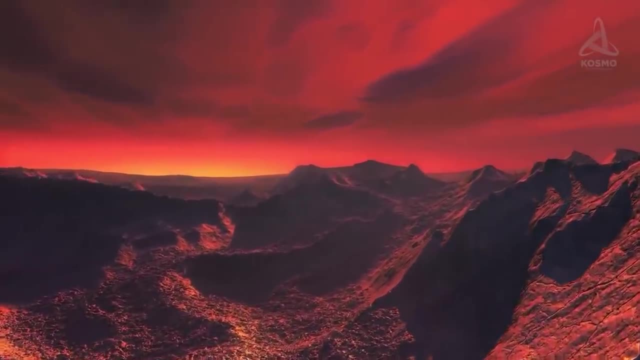 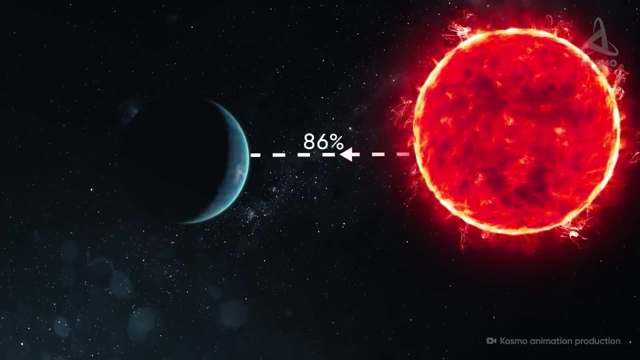 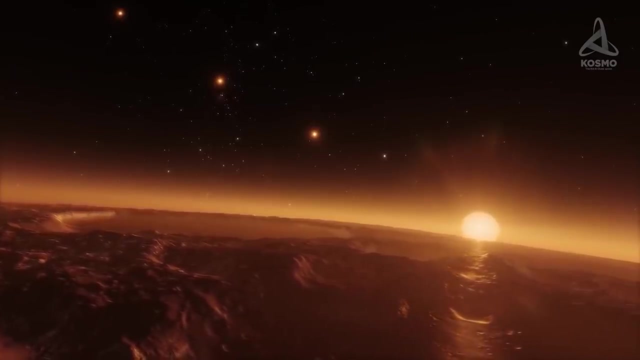 times that of the Earth. TOI 700 d is thought to be a rocky world, but its exact composition is not yet known. The amount of energy received by the planet from its star is 86% that of the amount we receive from the Sun. Assuming the planet's atmosphere is similar to ours, the steady-state temperature on 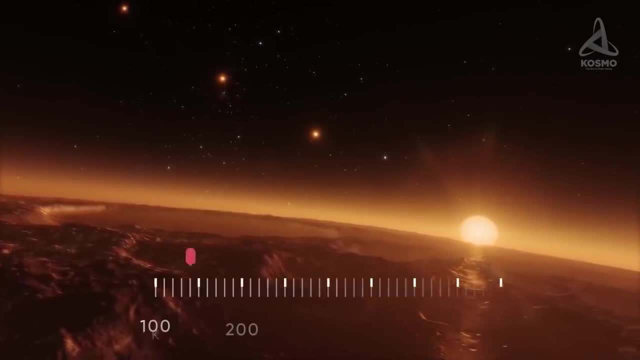 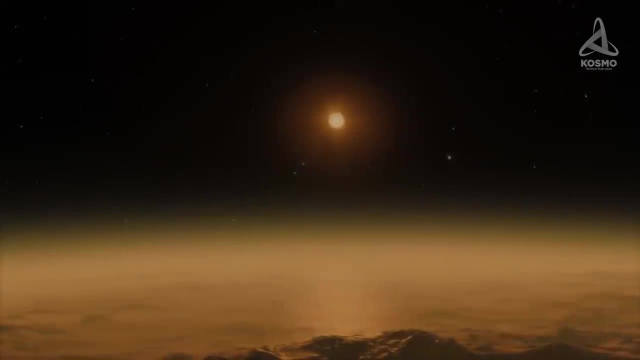 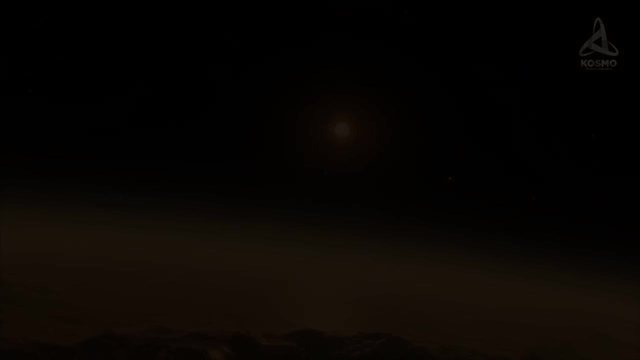 the surface of TOI 700 d is estimated at 268.8 Kelvin, or 4.3 degrees Celsius below zero. However, due to the greenhouse effect or other features of the atmosphere, we may not know yet- this figure may shift either up or down. There is no precise data on the eccentricity of TOI 700 d, but it is. 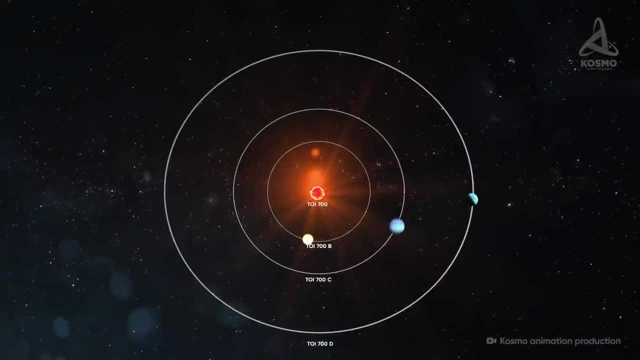 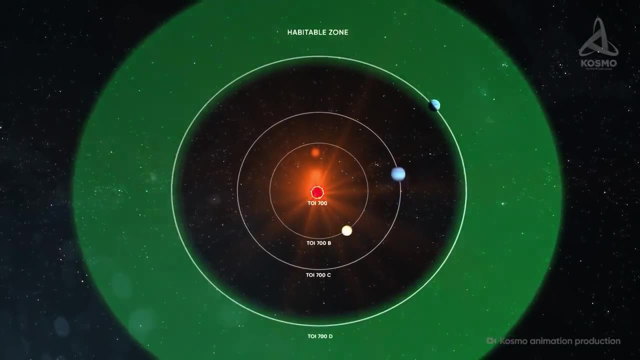 thought to be small at around 0.11.. As the planet's orbit finds itself at the inner edge of the Goldilocks zone, the planet's eccentricity, however small, may incidentally turn out to be perceptible when the planet comes too close to its star from time to time. 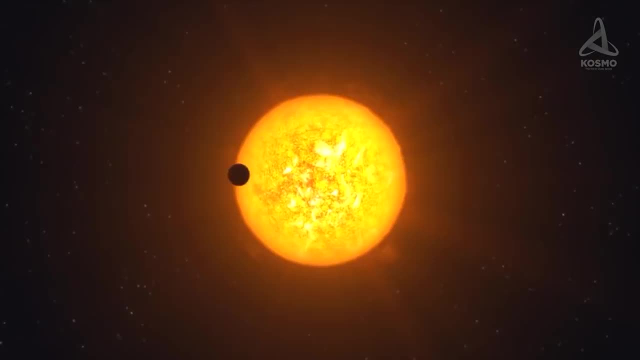 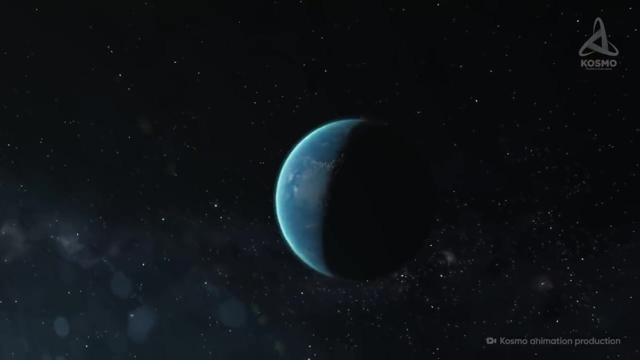 Thus actually leaving the habitable zone Still. with a year on the planet lasting slightly over one Earth month, such unfavorable periods are expected to be rather short. If there are living creatures on TOI 700 d, then they might be able to weather the harsh spells in a state of anabiosis. 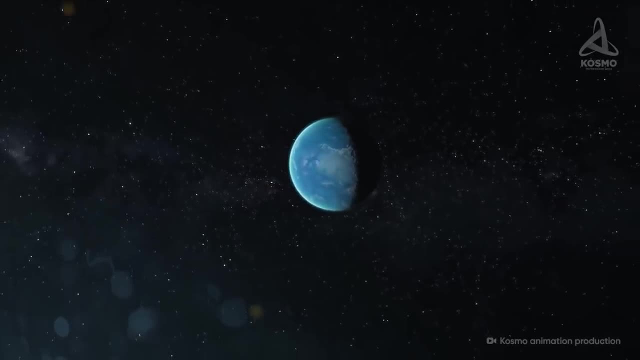 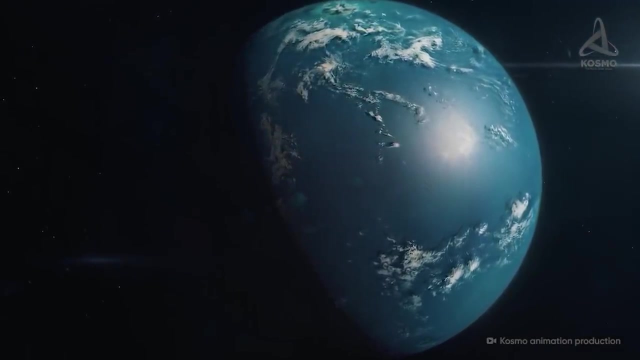 Alternatively, they could adapt or migrate to less inclement areas. Even though the data acquired by spectral analysis of TOI 700 d is not yet clear, the data is still available. To be sure, the data from TOI 700 d can't be enough for making conclusions. There is a chance that there is liquid water. 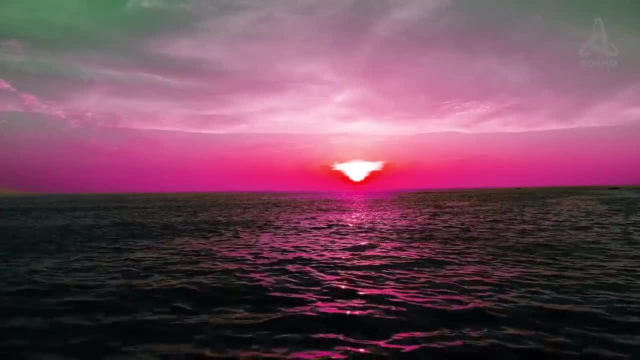 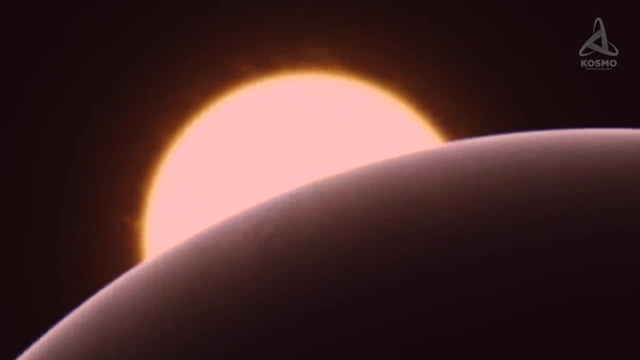 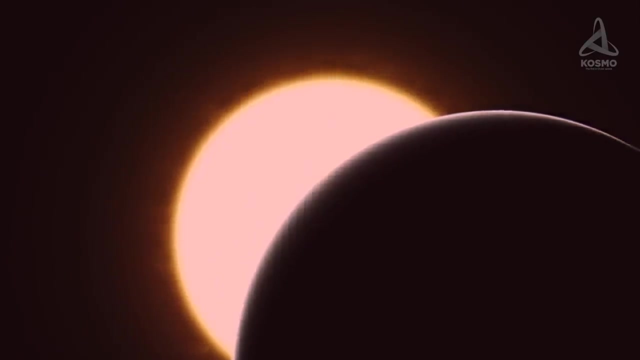 on the planet's surface, Then there is bound to be the greenhouse effect too, which will help the surface temperature to reach favorable values. As I've already mentioned, TOI 700 d, along with the other known planets in the system, is highly likely to be tidally locked to its star. If this is the 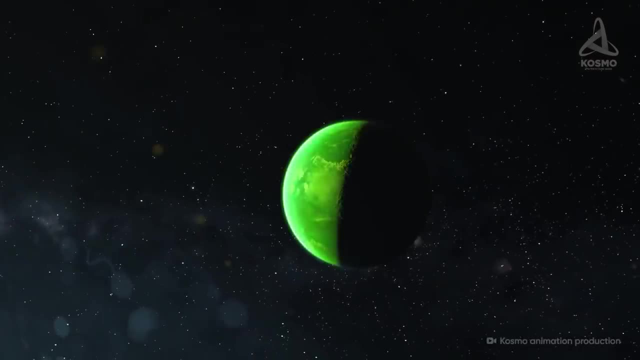 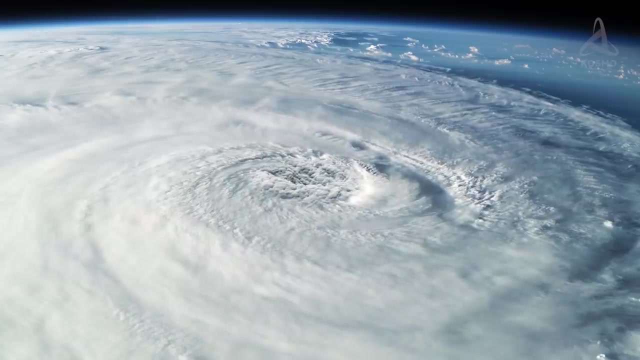 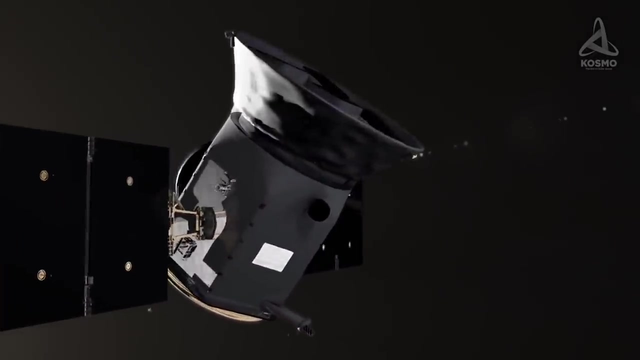 case, there should be a stark difference in temperatures between the sunny side and the shadow side. This contrast could be leveled off by a dense atmosphere, but that would cause powerful hurricane winds. Although the main mission of TESS has been accomplished by now, it still has enough. 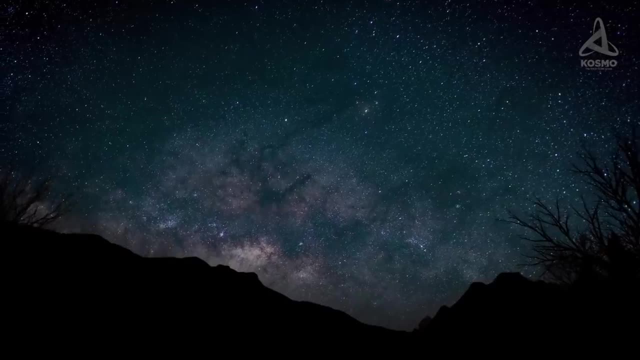 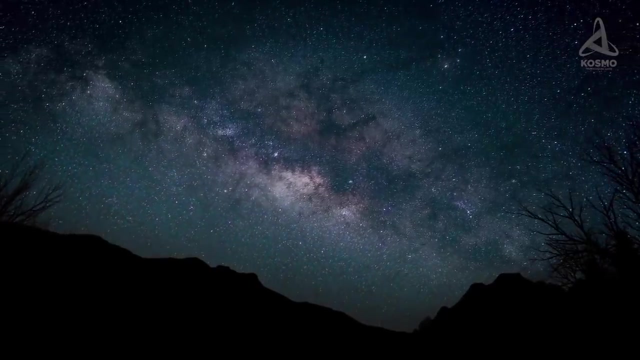 resources to carry on operations. The telescope will continue taking snapshots of the sky, including the Milky Way plane, which is the most challenging direction for observation. Over 2,100 exoplanet candidates have been discovered by TESS. To be sure, there should be a stark difference in temperatures. 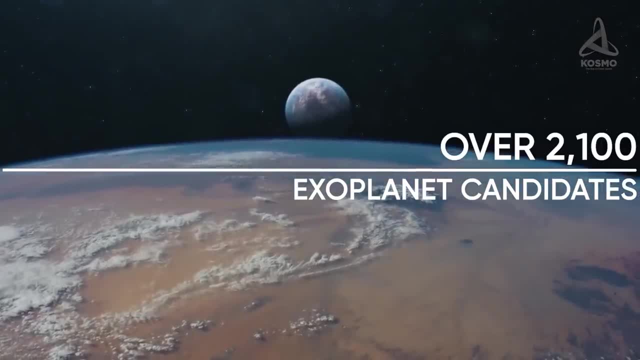 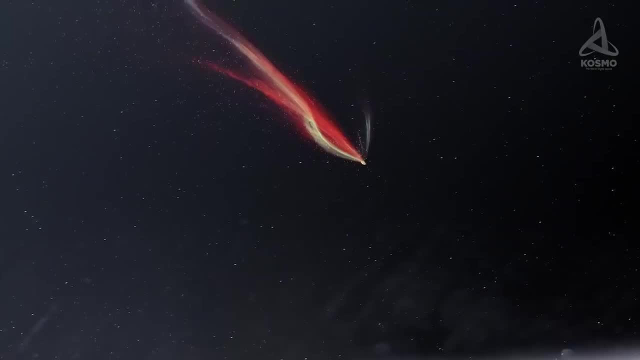 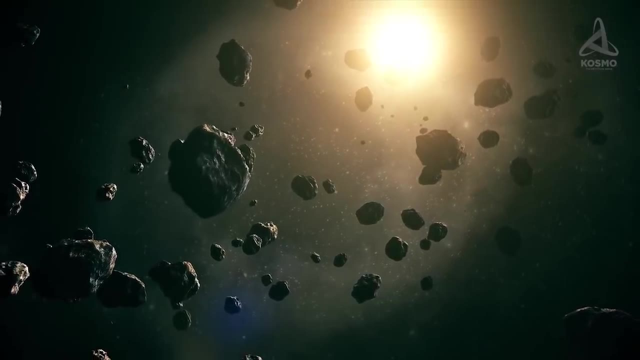 in the course of the main mission. Not less than 66 of them have already been confirmed. Apart from that, six supernovae flares have been registered, three exocomets identified and a great number of photos taken of small bodies in the solar system. The latters were not objects of the main mission. 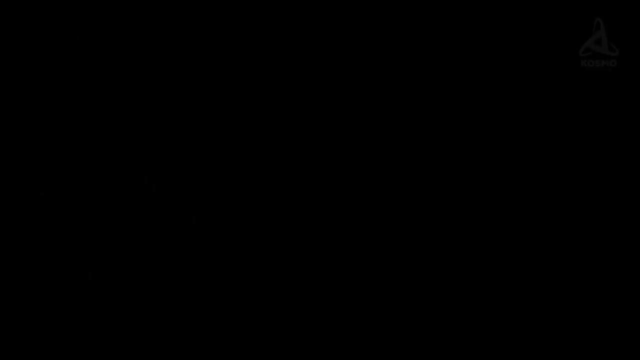 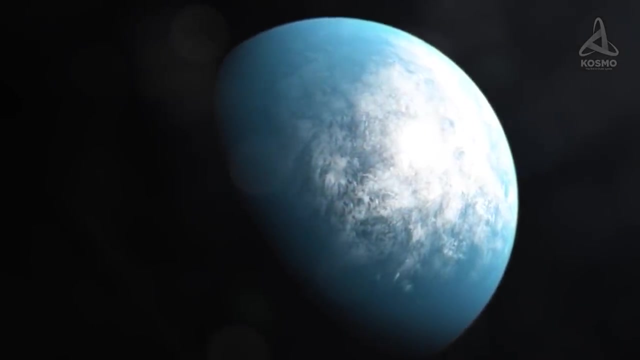 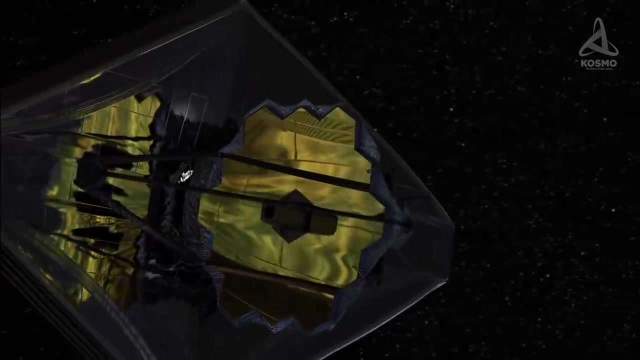 but are of course of scientific interest. TOI 700 d is still guarding its mysteries and waiting for its explorers. Great hopes are placed on the new orbital telescope James Webb, which may help investigate this world and a number of other ones. The new telescope is supposed. 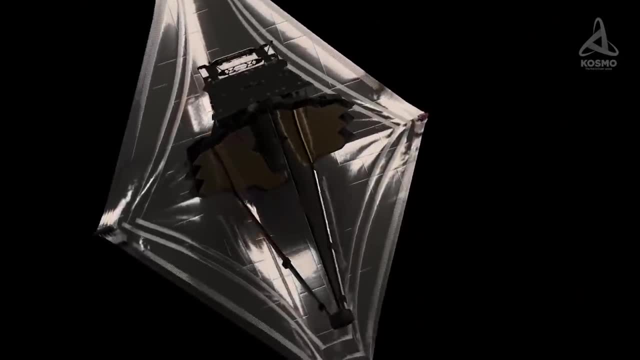 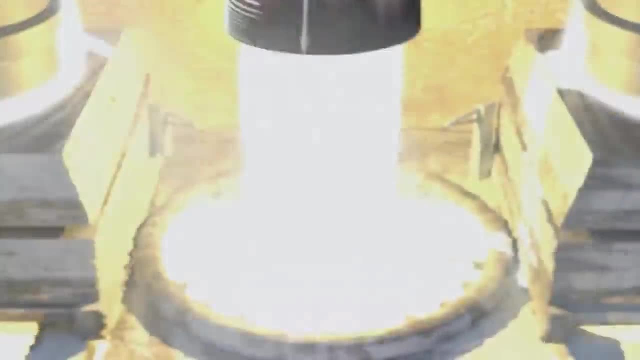 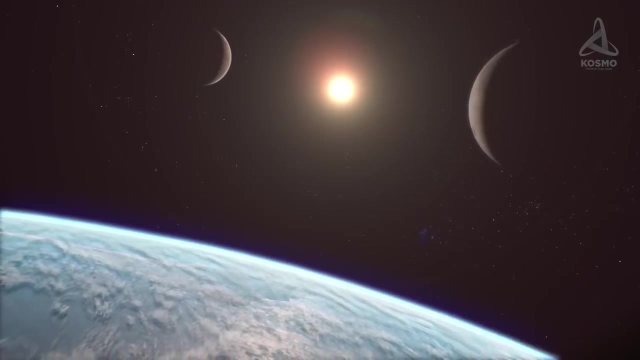 to provide images of not only exoplanets lying closest, but also detect their moons and carry out spectral analysis of their surfaces. The launch of the telescope is planned for 31 October 2021.. If all goes according to plan, first data will 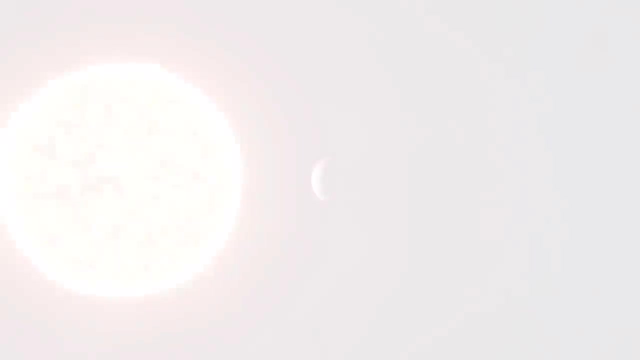 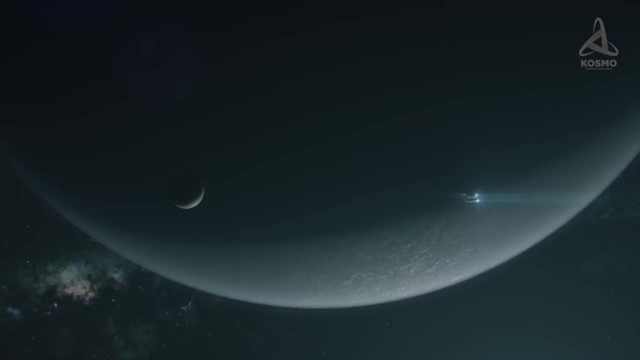 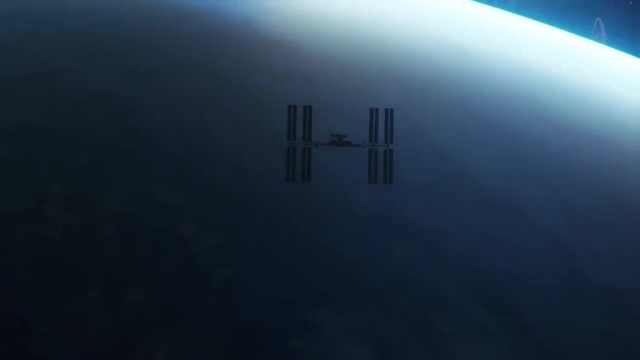 be available as soon as next year. Will we ever discover a world that could rightfully be called the second Earth, And if we do, will we be able to reach it? Distances in space are just too much for humans. Could it be that we are confined to the limits of? 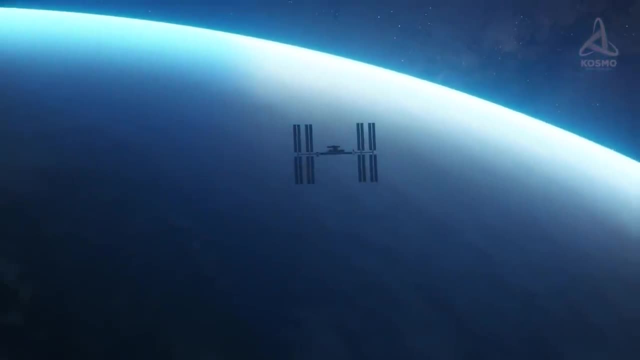 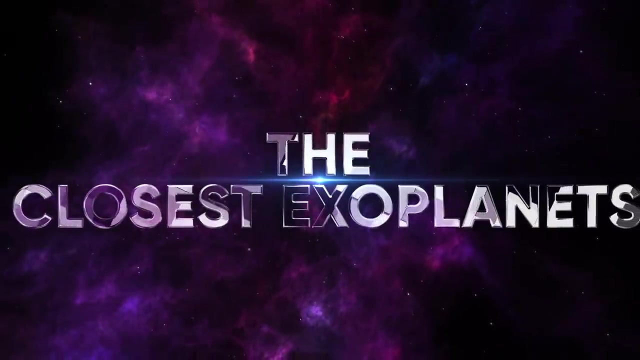 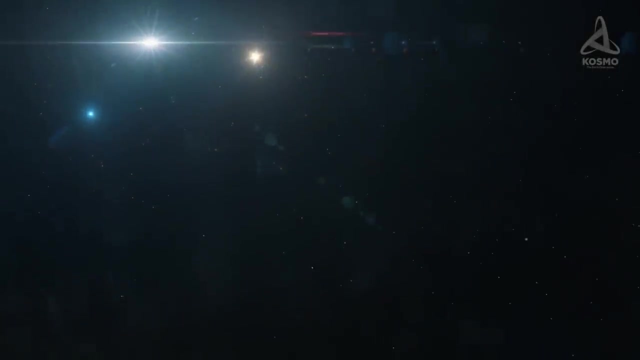 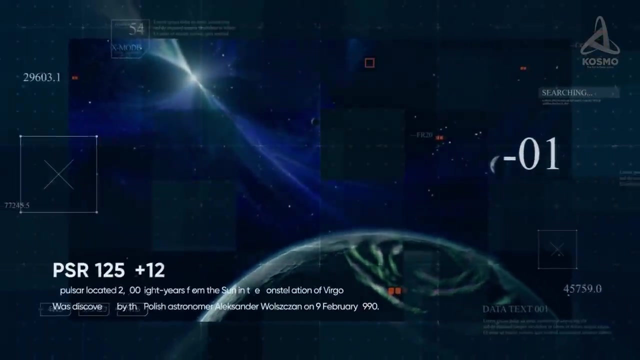 our system forever allowed only to gaze at the vast, infinite universe. Several centuries ago, it was quite unimaginable to admit of discovering exoplanets. However, everything changed In 1992, as the Polish astronomer Alexander Wolszczan was studying. 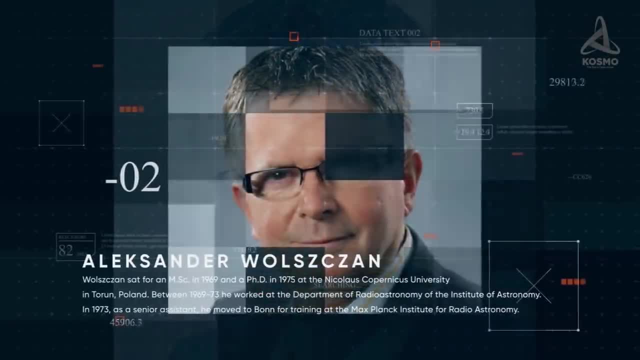 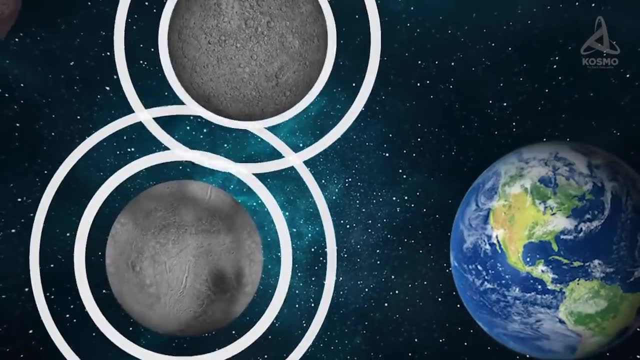 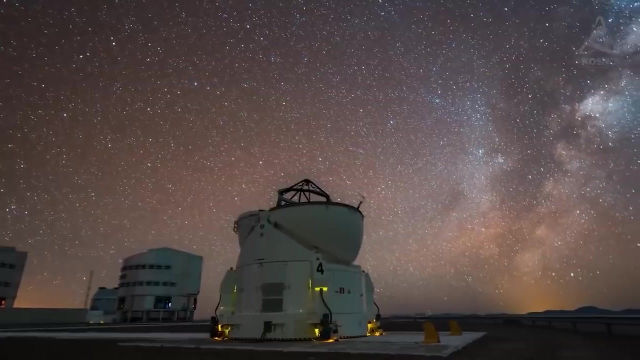 the pulsar PSR 1257-12,, it was noticed that its pulsation period was irregular, which was accounted for by the influence of two planets with a mass four times that of our Earth. This hypothesis was later confirmed, which led to the conclusion that the first planetary system 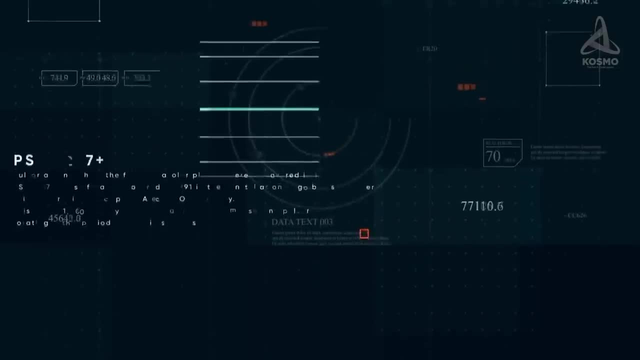 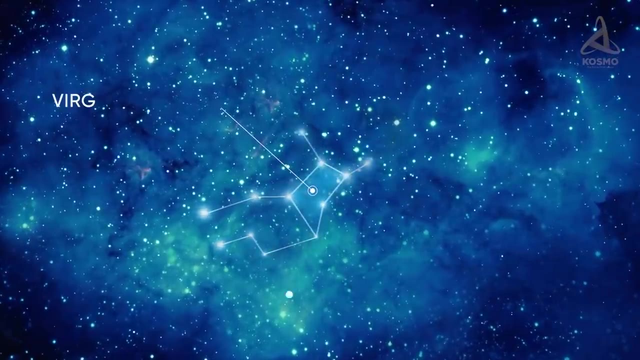 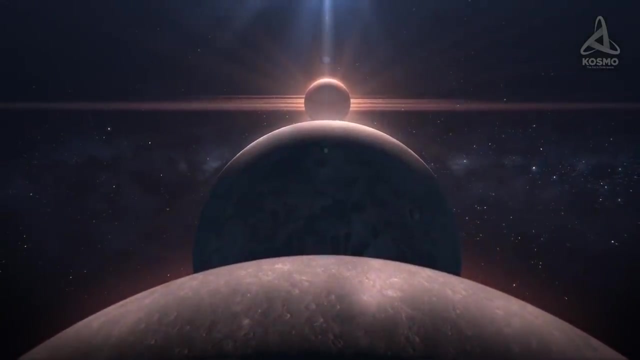 beyond ours had been discovered. There are three objects in that system, two of which have a mass similar to that of the Earth and are comparatively close to their pulsar in the constellation Virgo, Due to the fact that it is rather remote from us and the conditions for sustaining life are poor. 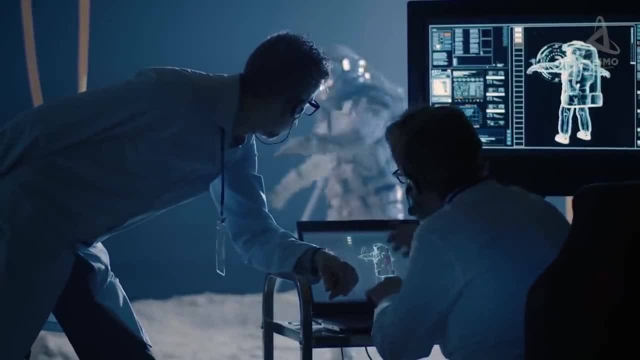 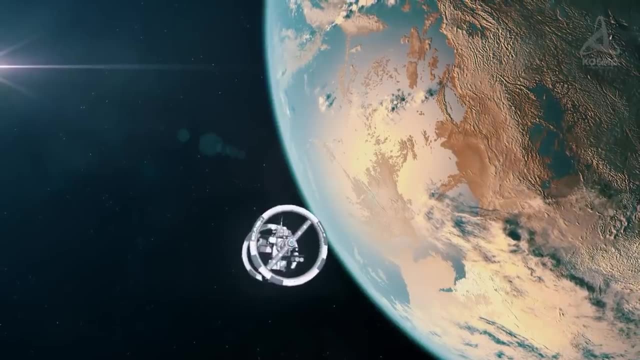 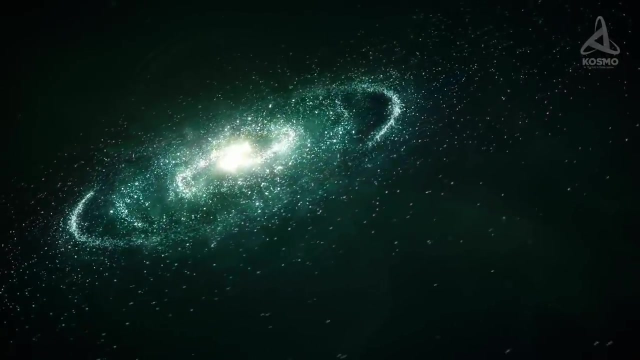 the PSR 1257-12 system is of little interest to scientists, although its discovery led us to believe that the search for Earth-like worlds may eventually be a success. Just three years later, the first exoplanet orbiting a Sun-like 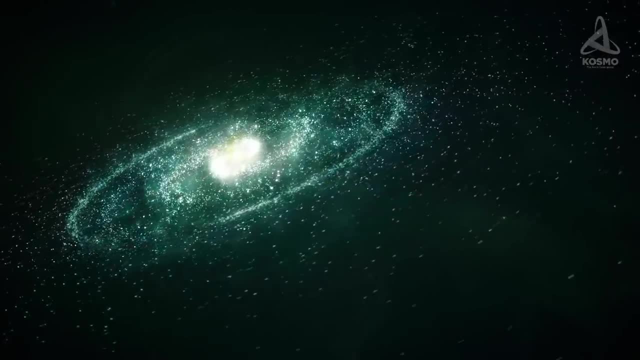 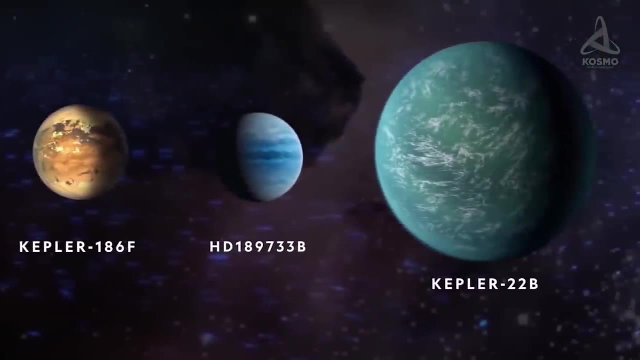 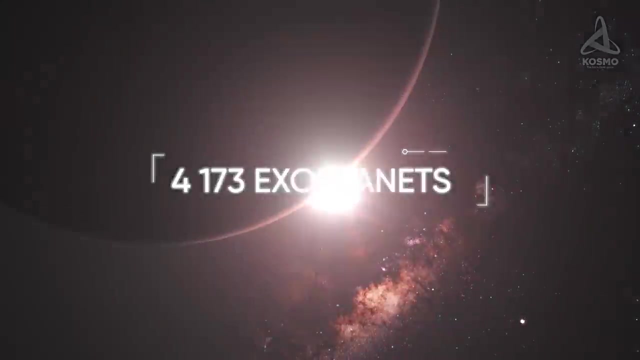 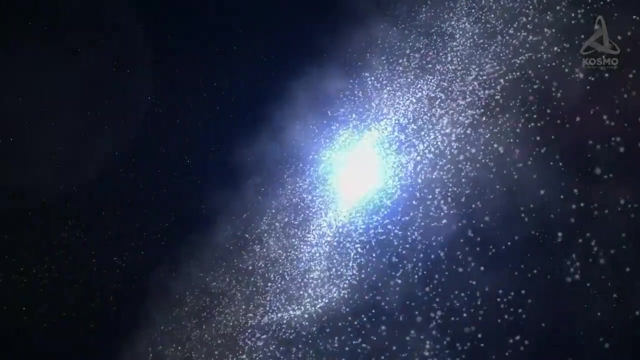 star was discovered 50 light-years away from the Earth and was dubbed 51 Pegasi b. Just several years later, the number of confirmed exoplanets counted dozens, and today there are 3,173 exoplanets in 3,096 different planetary systems unknown to science. 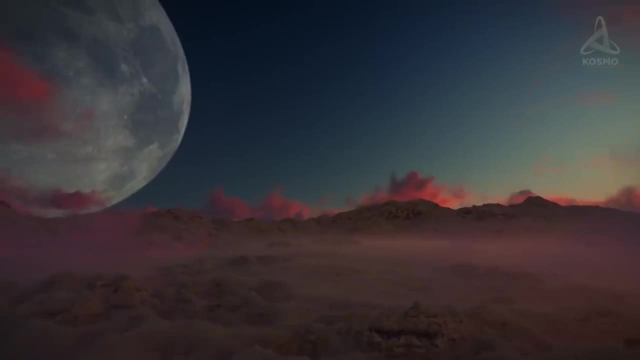 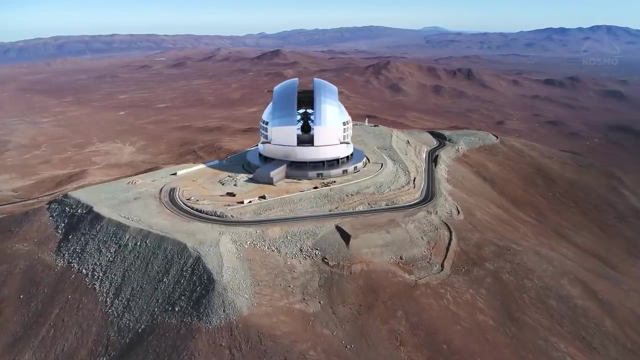 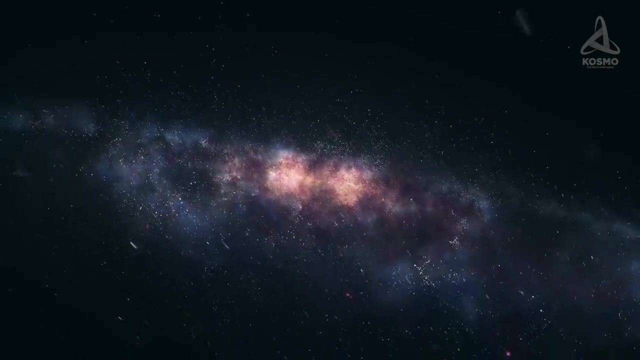 In addition, a great number of Earth-like objects is still awaiting the confirmation of their status, which is possible after a secondary registration with telescopes on Earth. The number of celestial objects of this kind in the entire Milky Way may well be over 100 billion. with about one-fifth of them bearing the name of the planet Earth. The number of celestial objects of this kind in the entire Milky Way may well be over 100 billion, with about one-fifth of them bearing the name of the planet Earth. 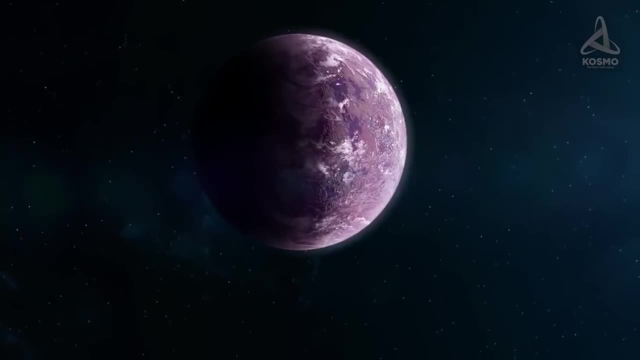 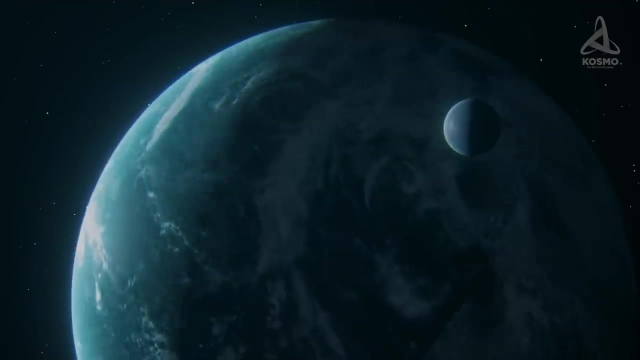 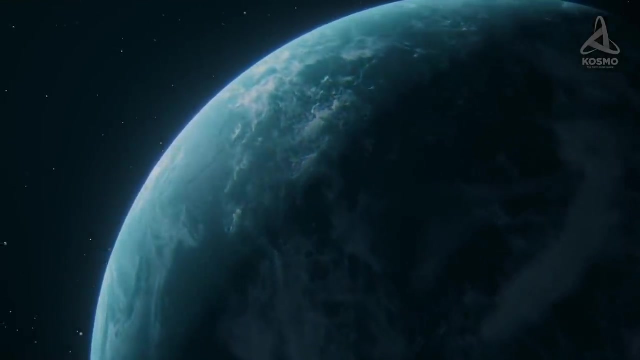 Interestingly, most of the discovered Earth-like exoplanets are located not very far from our system ROS 128 b. This planet was discovered in 2017 by European scientists with the help of the High Accuracy Radial Velocity Planet Searcher, or HARPS, at the observatory in Chile. 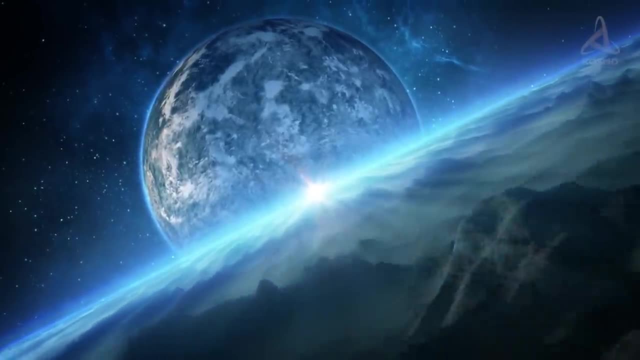 The object is located in the single star system ROS 128b. The object is located in the single star system ROS 128b. The object is located in the single star system ROS 128b 1-8,, which is the 13th closest star to us. 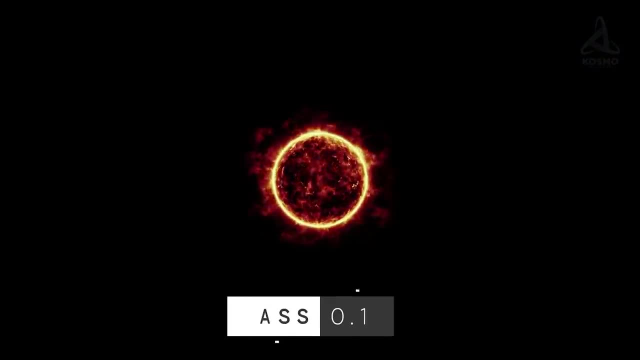 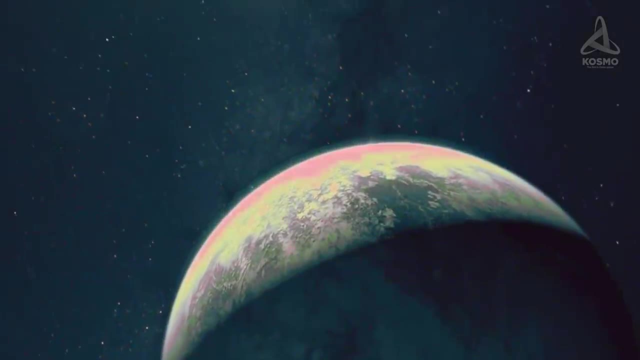 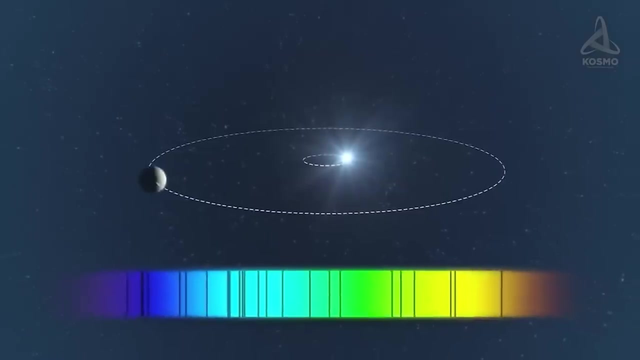 The object is a faint red dwarf with a mass of 0.15 that of the Sun. It was possible to discover this planet thanks to its gravity, which leads to minor variations of the stellar spectrum of its parent star. While observing these variations, HARPS is able to spot planets around stars. 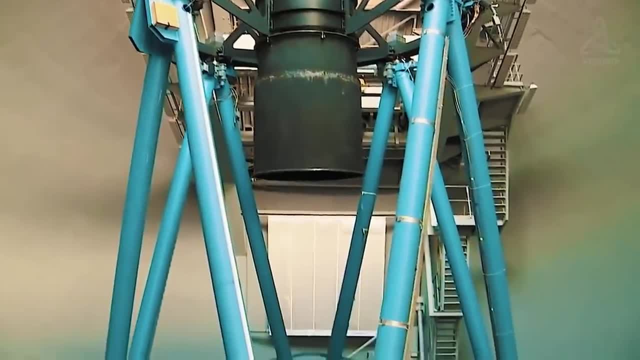 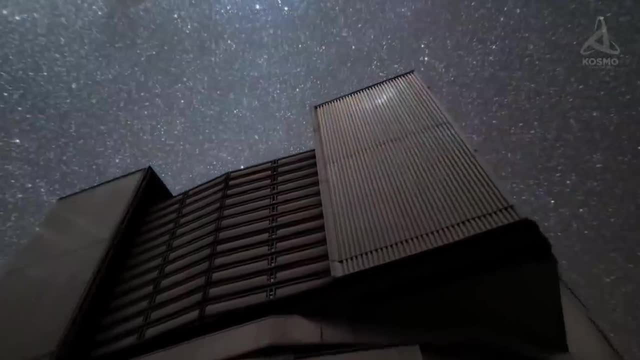 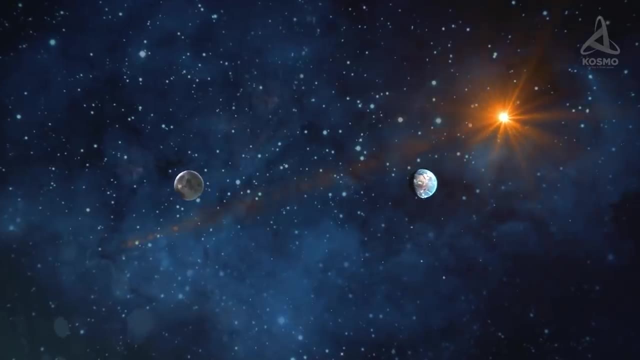 In this particular case, it took the telescope approximately 10 years to collect sufficient data before discovering this planet. This effort paid off. ROS 128 b became the second Earth-like exoplanet lying closest to us. It is located 11 light-years away from the Earth in the constellation Virgo. 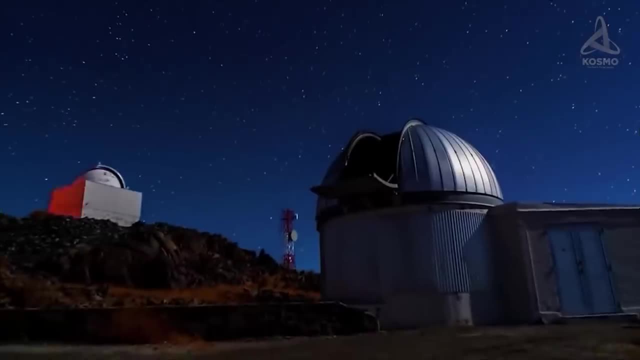 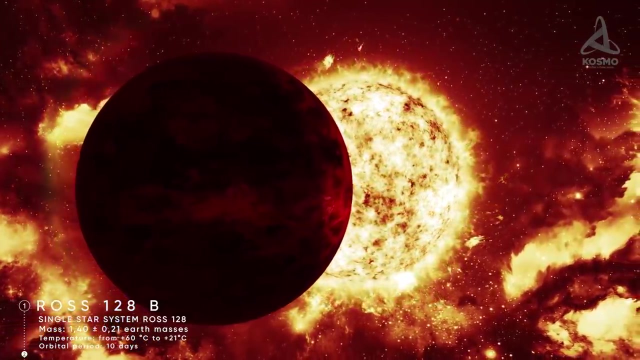 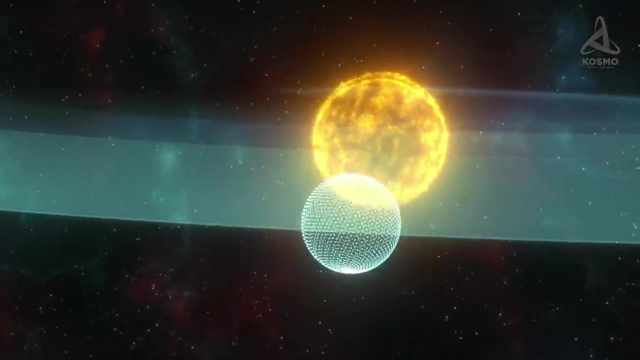 Apart from that, astronomers claim it to be the most moderate of all known exoplanets, due to its mass, its temperature and its rather calm parent star. It takes this planet 10 days to orbit its star. It finds itself in the habitable zone since the temperature of the photosphere and luminosity. 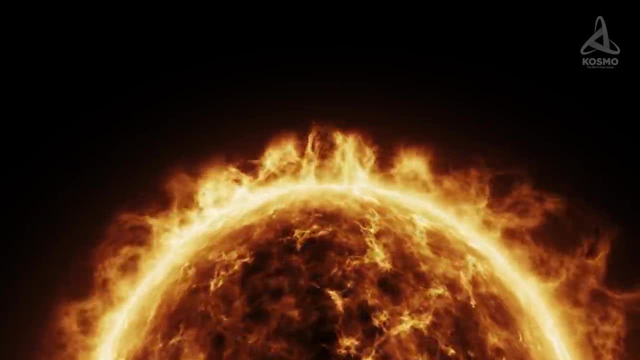 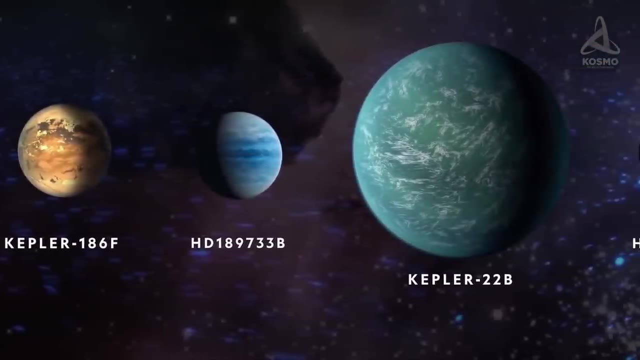 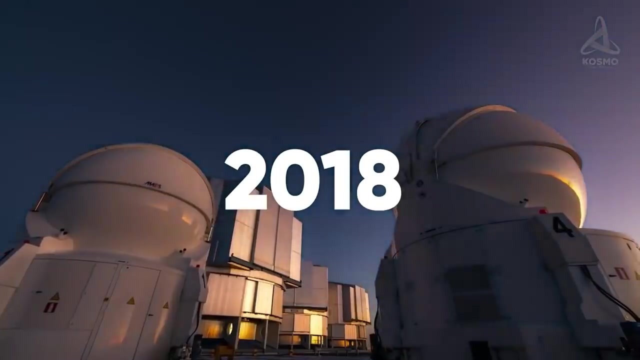 of ROS 128 are low. It is also classified as an Earth-like type of planet and, at the moment, ROS 128 b is one of the most likely candidates to be a potentially habitable exoplanet. Besides, research done in 2018 confirmed that its climate is favourable enough to 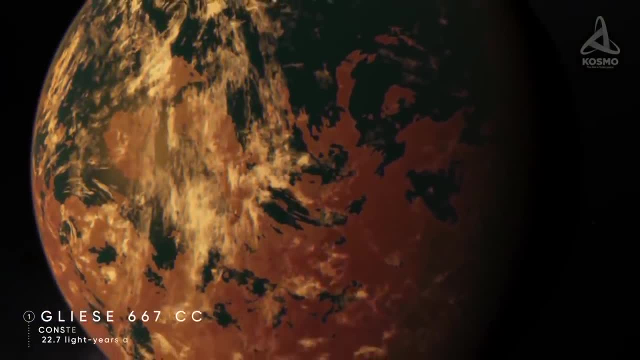 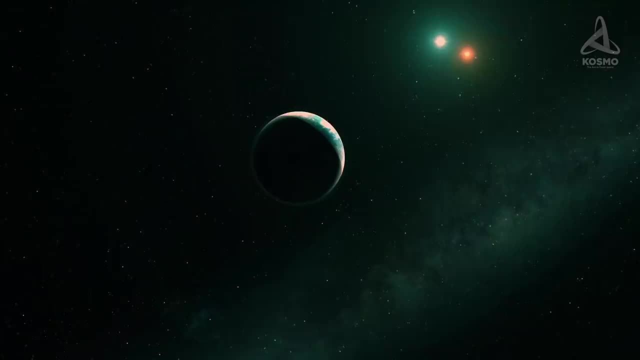 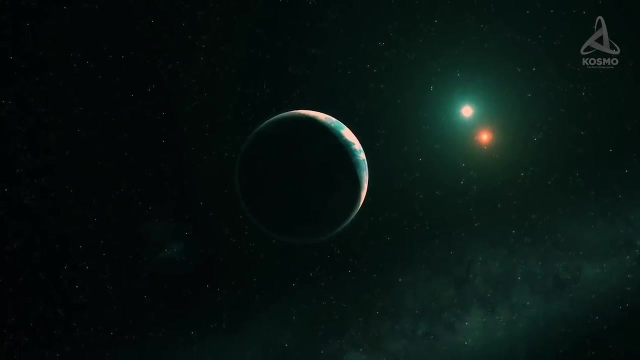 sustain life. Another exoplanet on the list of Earth-like objects located closest to us is Gliese 667 cc. This celestial body is part of the triple-star stellar system Gliese 667 in the constellation Scorpius. It consists of two orange dwarfs and one red dwarf. 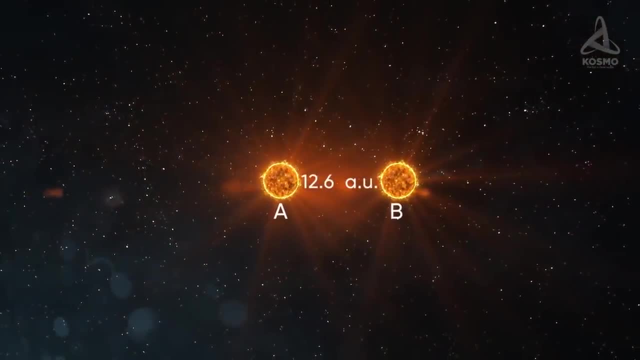 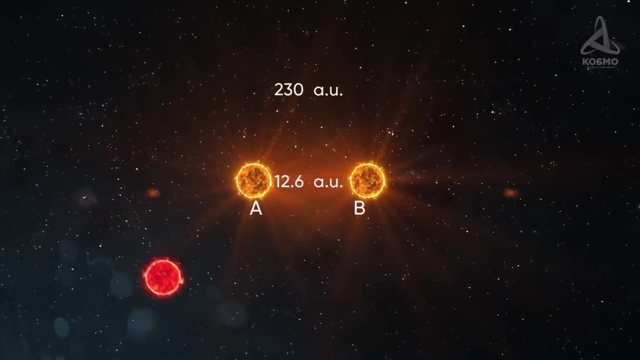 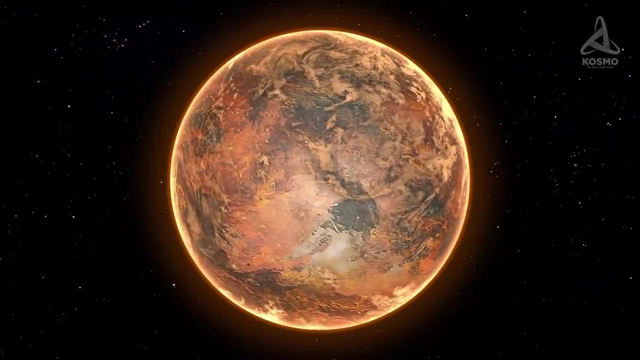 The first two components, A and B, lie 12.6 astronomical units from each other, with the third component orbiting them at a distance of 230 astronomical units. The Earth-like planet in this system was discovered on November 29, 2011, in the Geneva Observatory. 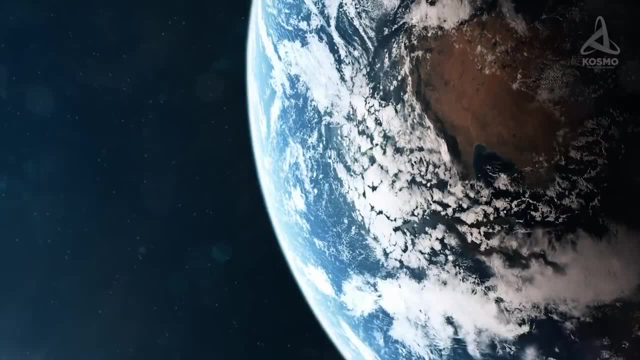 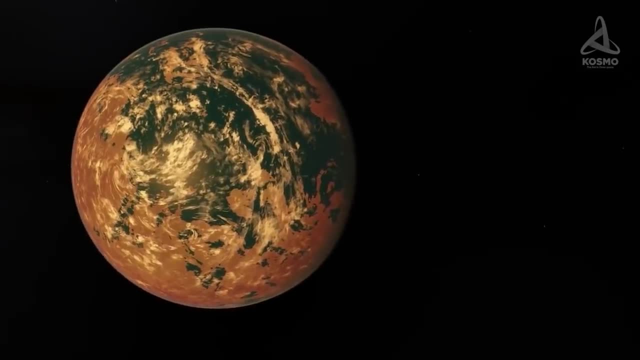 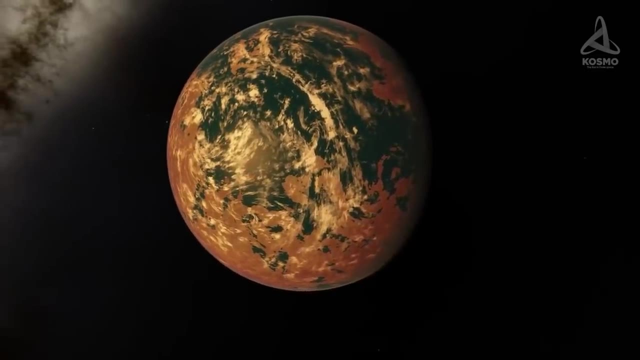 with the help of the Doppler method. The object is 22.7 light-years away from the Earth and is the second exoplanet orbiting the star. The mass of Gliese 667 cc is about 3.8 times that of the Earth, while its temperature range. 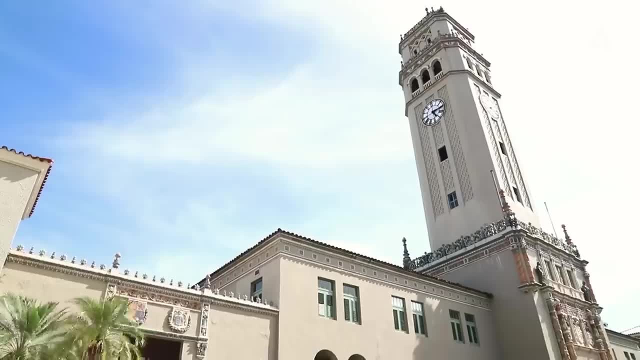 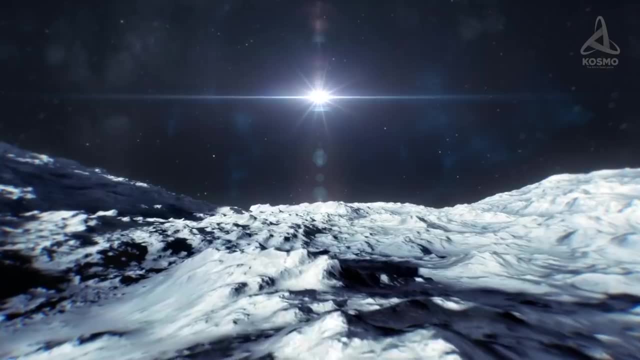 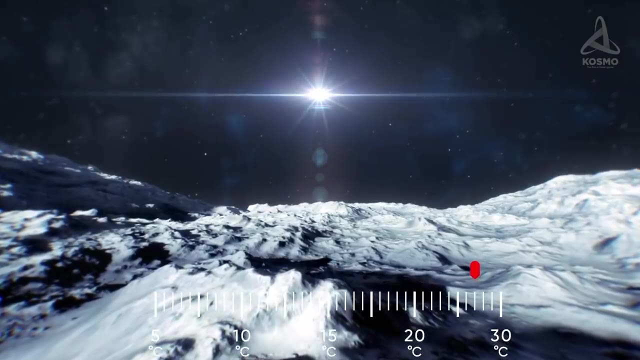 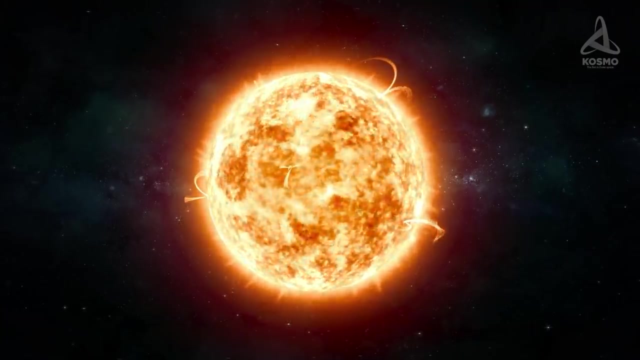 may be rather similar to the terrestrial one. Modelling at the Planetary Habitability Laboratory managed by University of Puerto Rico reveals that the average surface temperature of the atmosphere of Gliese 667 cc must be approximately 27 degrees Celsius. The planet receives about 90% of energy compared to that received by the Earth from the Sun. 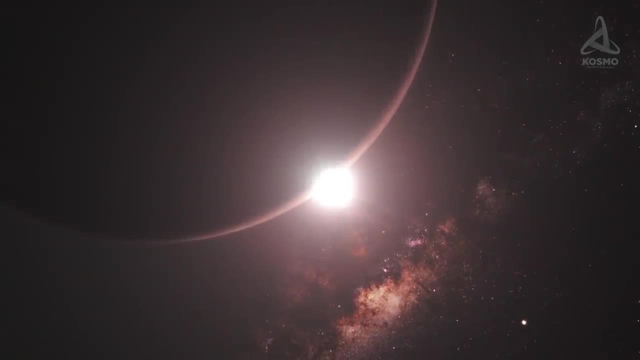 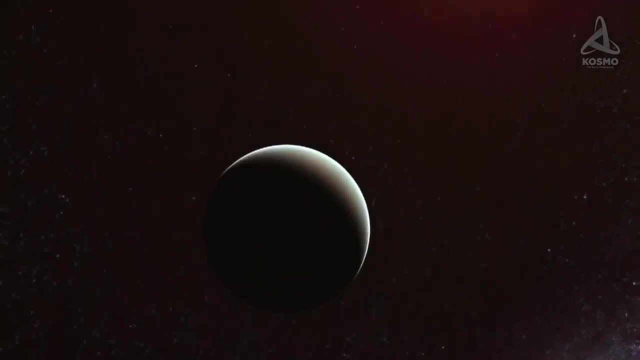 Also Gliese 667 cc is almost certain to be locked in its orbit, that is, it faces its star with one and the same side, If the planet's orbit does not curve too little and if its mass is not too big. the greenhouse. 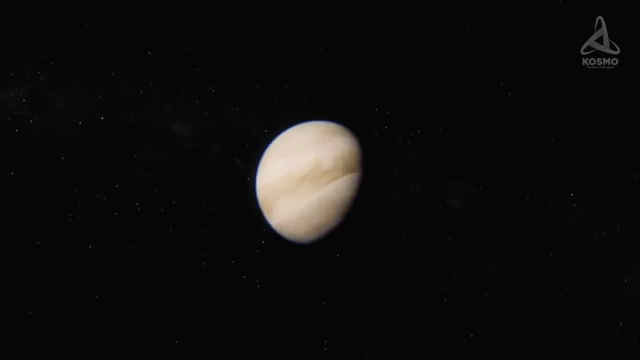 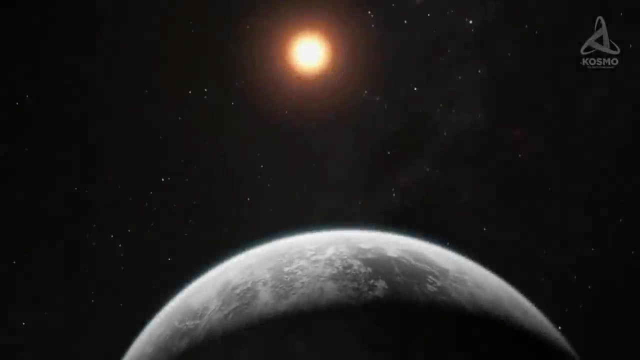 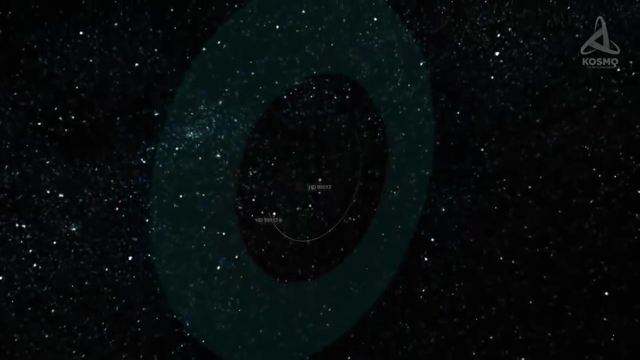 effect produced by the rather dense atmosphere must be quite sufficient to create favourable conditions for primitive life forms. Thank you for your attention. The next deserving object on our list is HD 85512 b, an exoplanet orbiting the orange dwarf. HD 85512 in the constellation Vela. 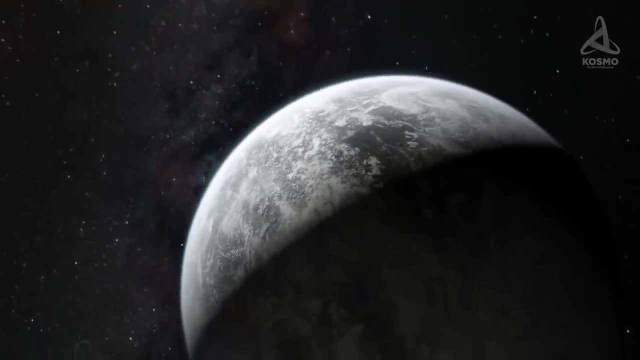 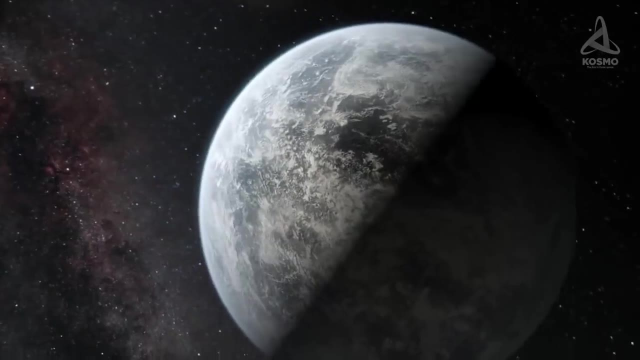 Its star is a single K-type main-sequence star with the mass 0.69 that of our Sun. As for its age, it is more than 5.6 billion years old. The star is a single K-type main-sequence star with the mass 0.69 that of our Sun. 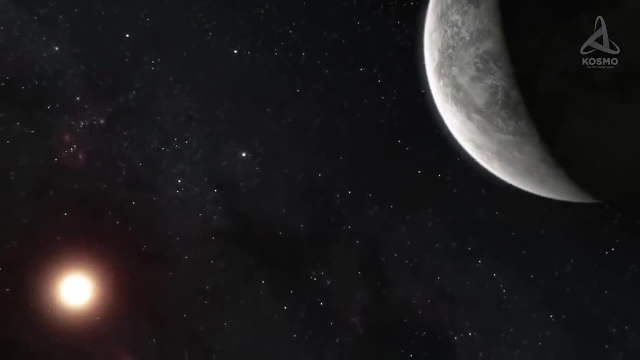 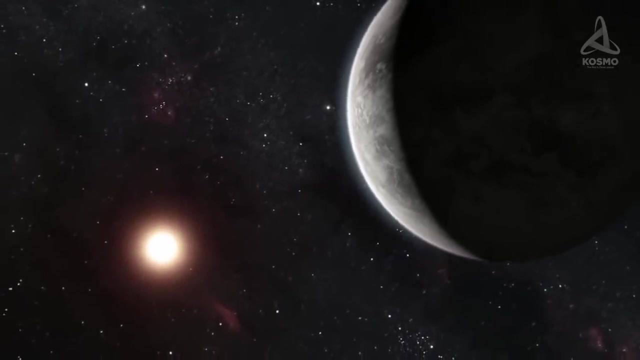 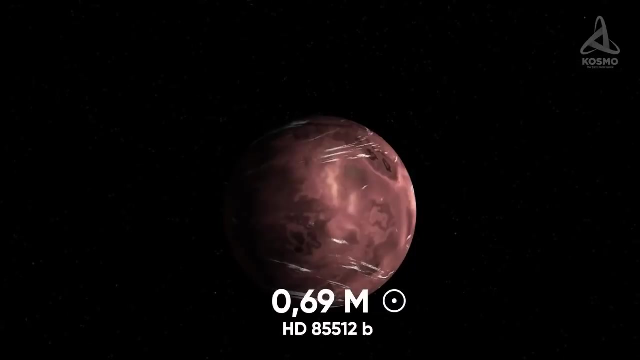 As for its age, it is more than 5.6 billion years old. The exoplanet discovered close to it is located 36 light-years away from the Earth, and its mass is 3.6 times that of our planet. At the same time, HD 85512 b may be one of the smallest planets in the habitable zone. 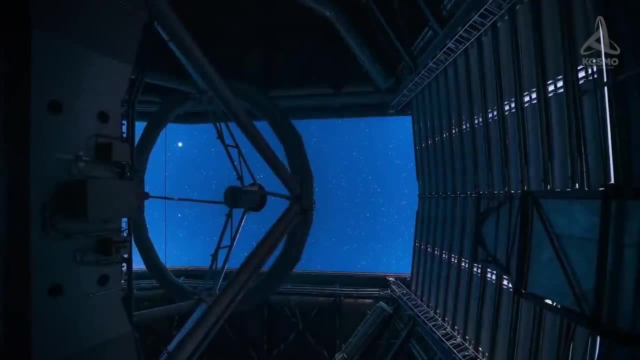 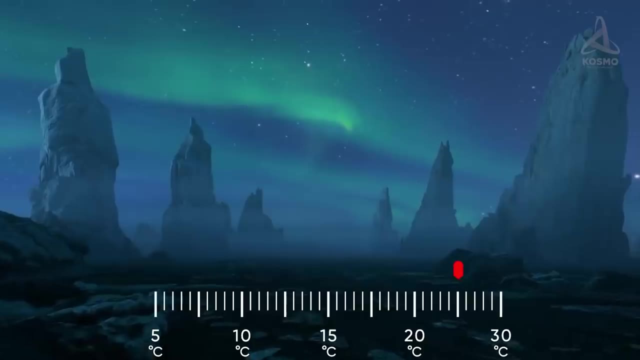 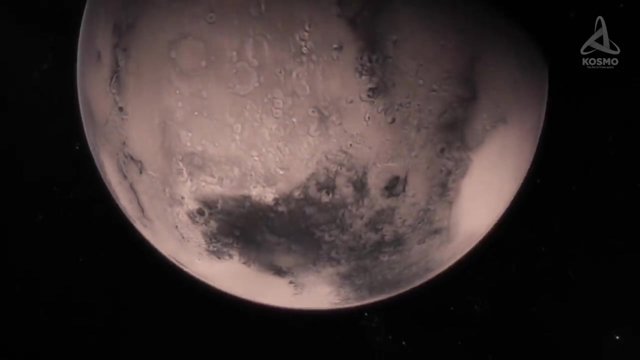 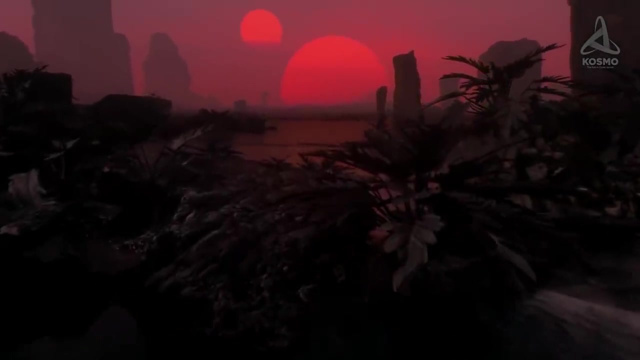 It was spotted in August 2011 with the HARPS telescope. It is about 25 degrees Celsius. If the planet's atmosphere is identical to that of the Earth, its surface temperature should reach 78 degrees Celsius. It is also highly probable that there is liquid water on this celestial body, which is why 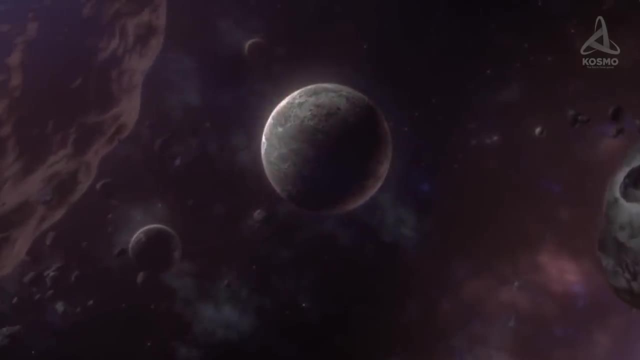 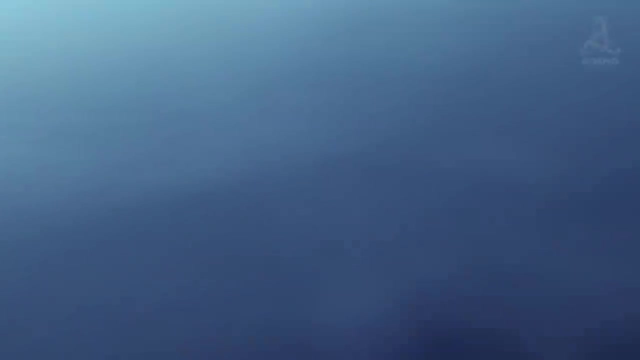 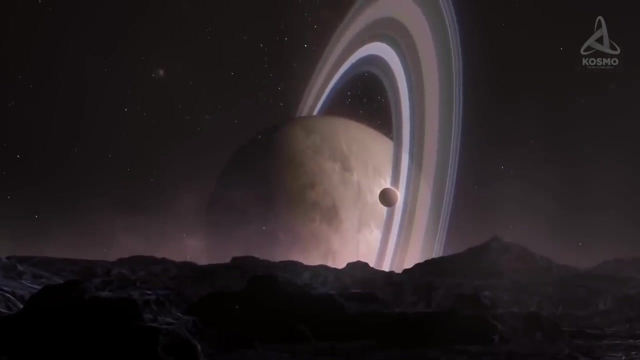 for some time, it was believed to become the most likely place where life would be discovered first. Apart from the objects mentioned, there are a number of other celestial bodies in the space located quite close to us which also boast some unique features. Many of them may well contain various life forms and may be not quite as far from us. 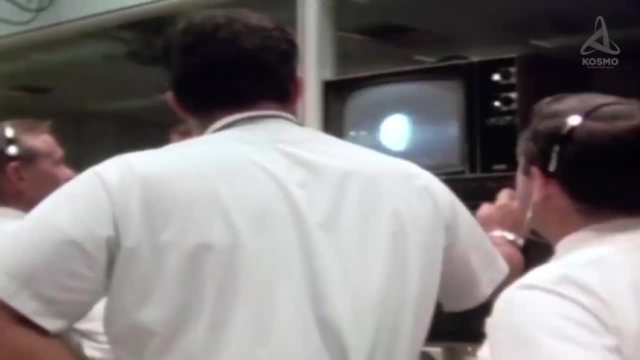 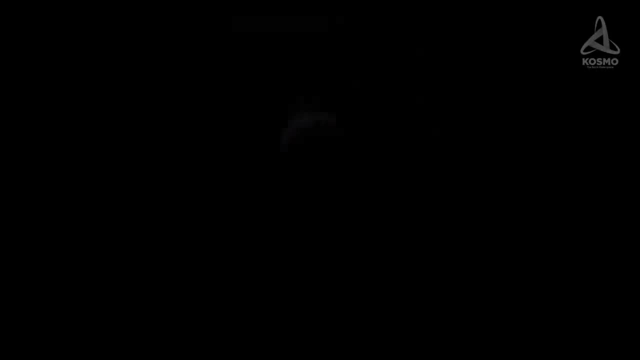 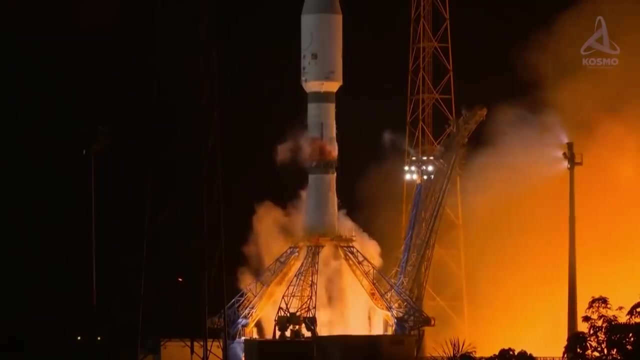 as we would imagine. However, we should bear in mind that some half a century ago, man did not possess a tenth of information known to us. today And in the future, the progress of our discoveries is going to escalate even more dramatically. For example, 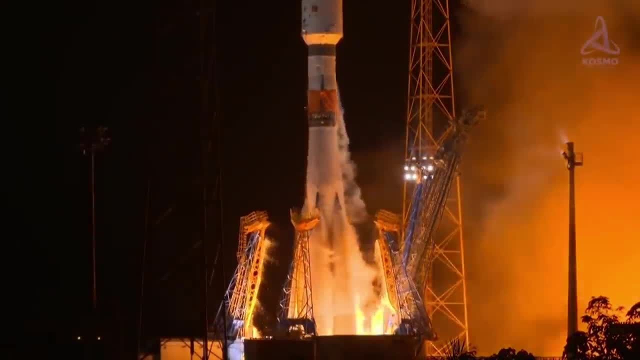 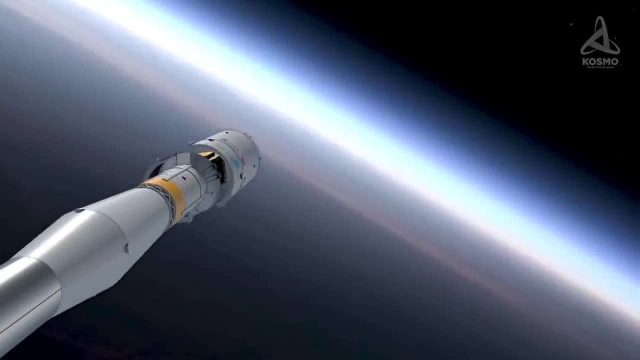 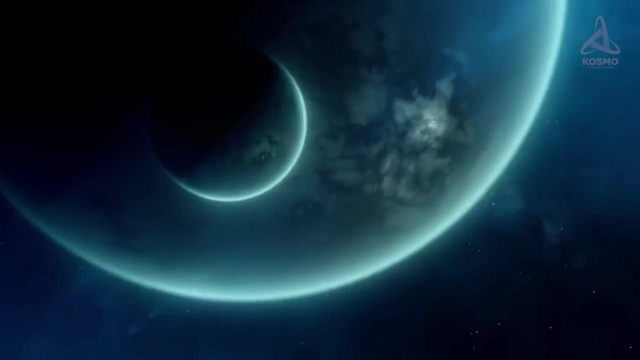 For example, on December 18, 2019, the Cheops Space Telescope was successfully launched in orbit by the European Space Agency. It is specifically aimed at exploring exoplanets using the transit method. It may be. this spacecraft is to contribute to the list of Earth-like exoplanets, and 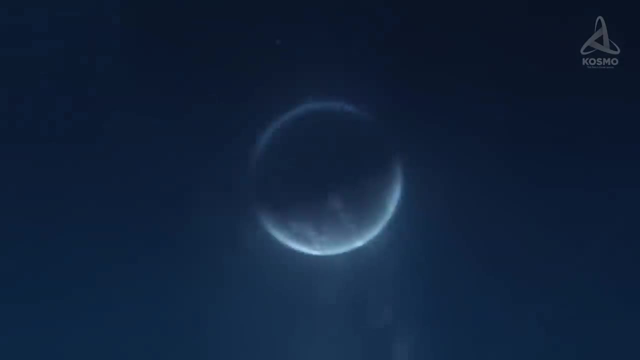 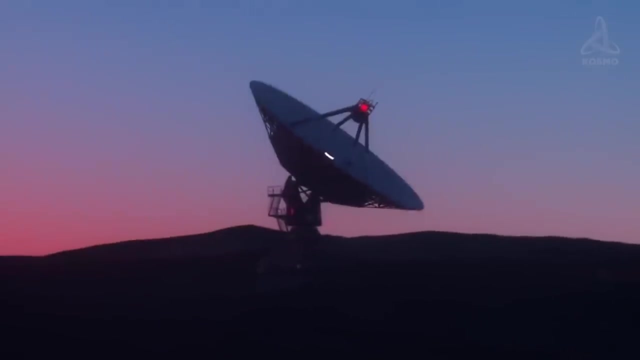 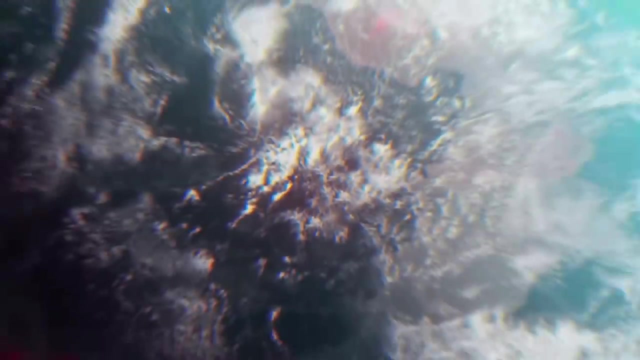 it may become the telescope to first discover alien life forms in the universe. Science does not stand still, and every new day bears witness to the fact that mankind continues to actively stride forward. If this progress does not lose its momentum, sooner or later we are bound to find an answer. 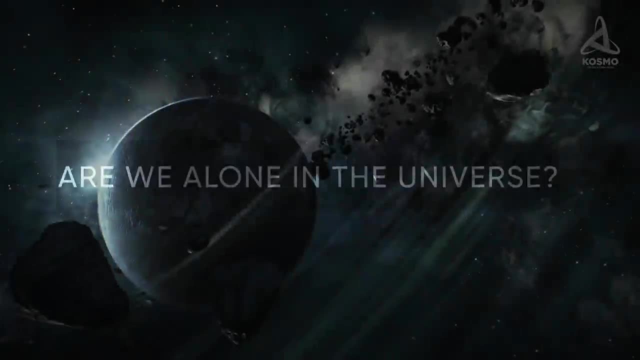 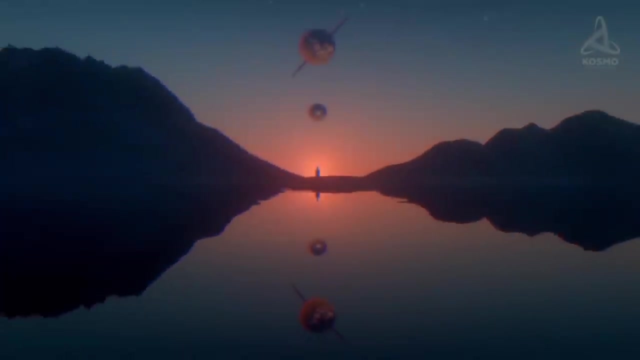 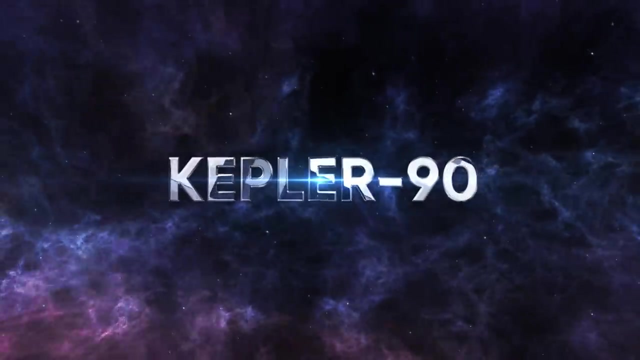 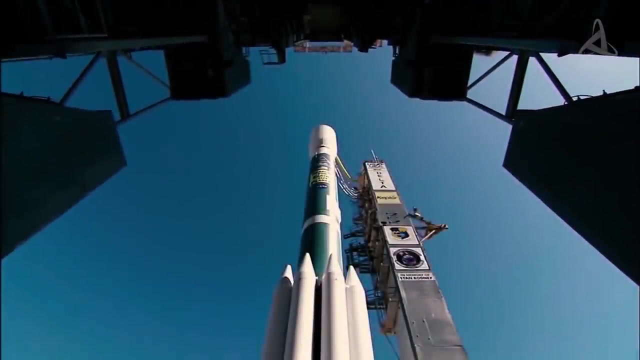 to the eternal, mind-perturbing question: Are we alone in the universe? And I hope the answer we get will prove that life is not a mere accident but a logical consequence of the evolution in our universe. The discovery of this object was made with the Kepler Space Telescope, whose mission 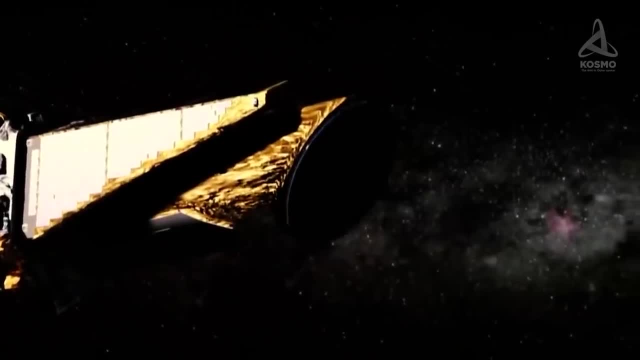 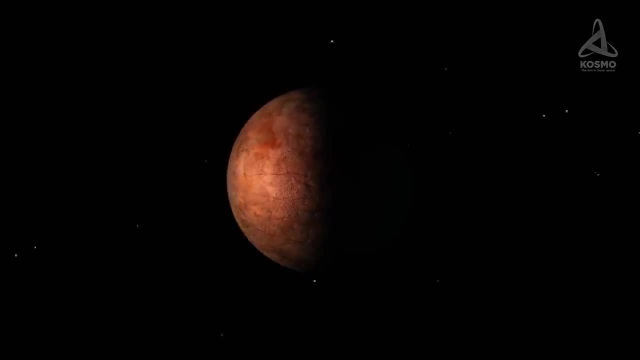 was to look for exoplanets. The Kepler star system became the 90th object spotted by the telescope. That is where the catchy nickname Kepler-90 comes from. Let's take a closer look at it. Kepler-90 is a yellow dwarf of spectral type G0V. 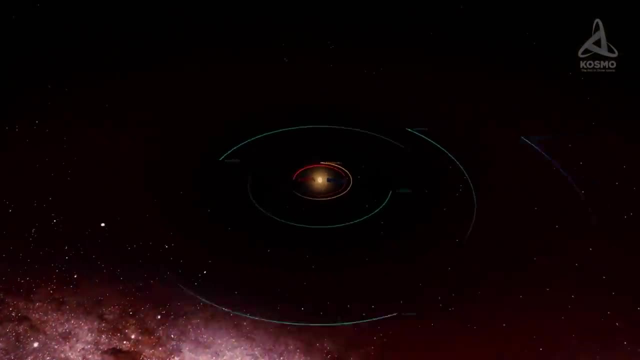 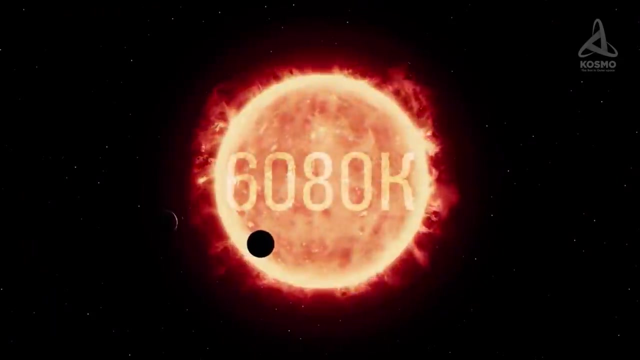 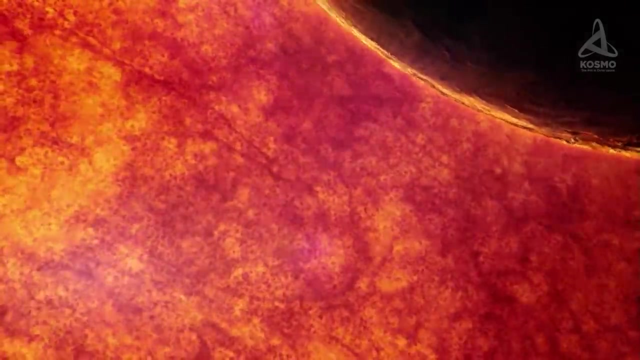 Both its masses are the same. It is a dwarf. Its mass and radius are approximately 1.2 times those of the Sun. As for the surface temperature, it equals 6080 Kelvin or 5800 degrees Celsius. The estimated age of the star is 2 billion years. 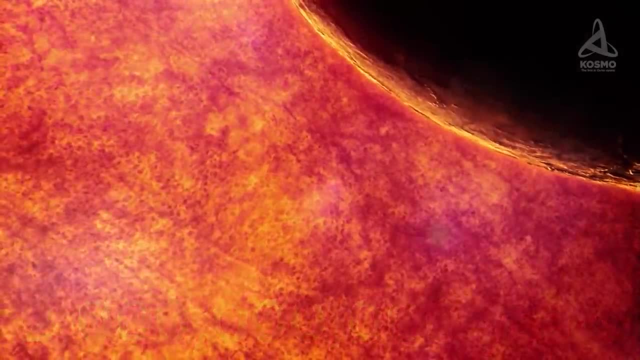 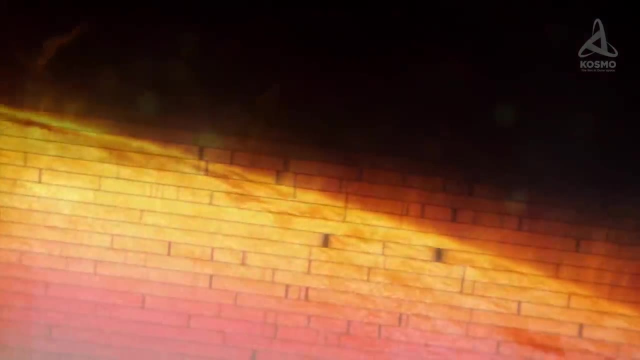 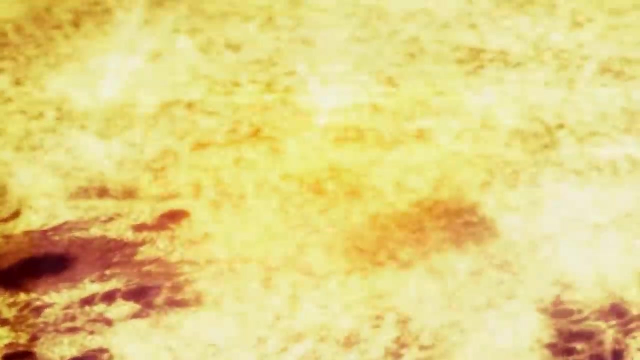 This makes it two times younger than our Sun, which formed about 4.6 billion years ago. It was possible to gauge the star's age by analyzing its spectrum, which helps establish the stage of the star's evolution. Another method instrumental for the purpose is observing stars lying closest to the object. 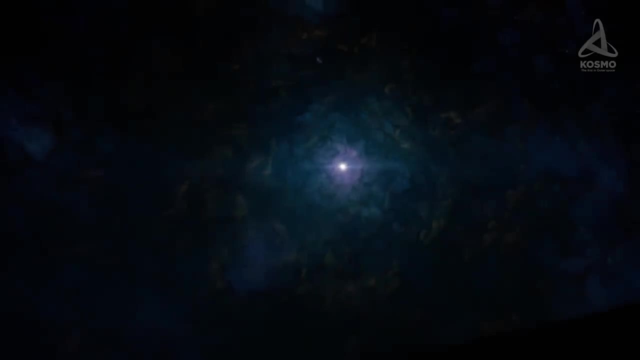 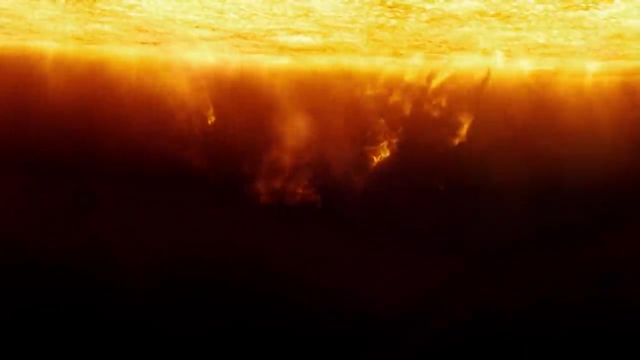 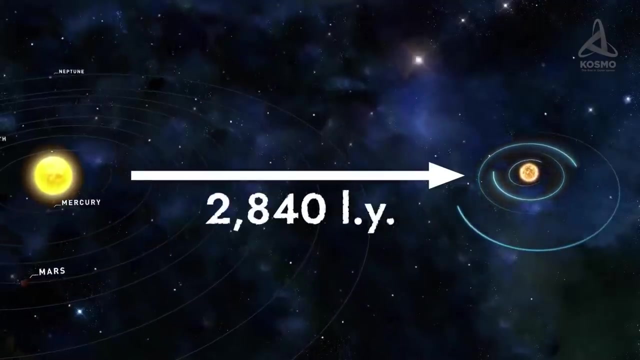 under scrutiny. Incidentally, Kepler-90 is too dim to be seen with the naked eye. Its luminosity, meanwhile, is approximately 1.7 times as intense as that of the Sun Located in the Draco constellation. it is approximately 2840 light-years away from our 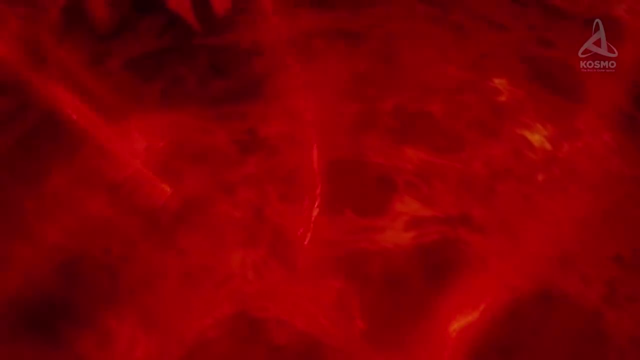 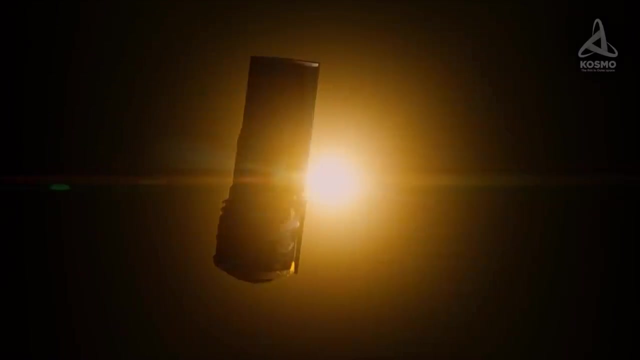 system. The object is a dwarf. Interestingly, the object is hardly notable for its properties. It is quite an ordinary main-sequence star without any particularly exciting features. It's the number of planets discovered in its system so far that makes it really stand out. 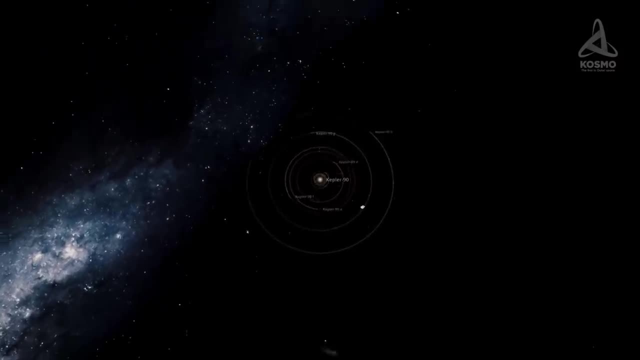 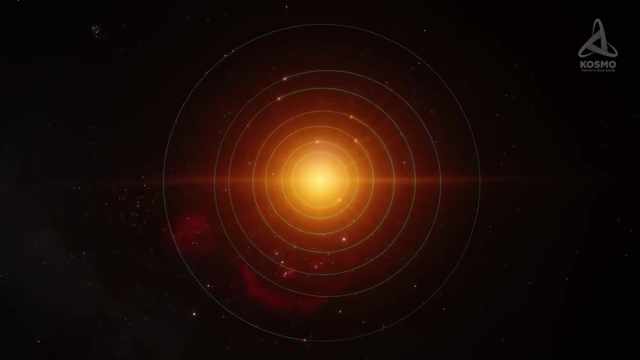 The only other system where we could observe as many as eight planets had been only our solar system. Before Kepler-90 had been spotted, the Sun held the first place in terms of the number of planets, with the following champions as the runners-up: 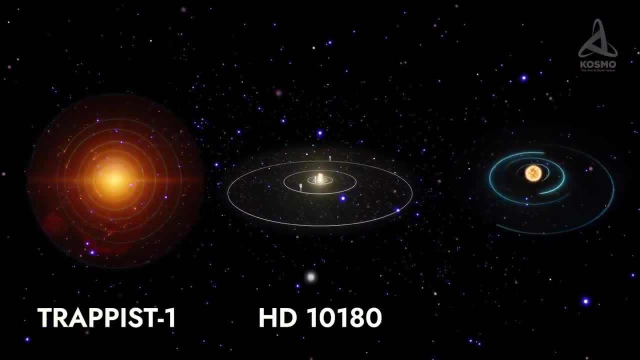 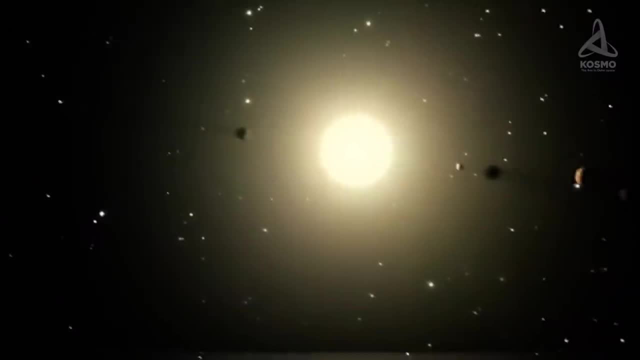 The Sun is the largest planet in the universe: The system's TRAPPIST-1,, HD 10180, and HR 8832.. Each of them has seven detected planets. At first glance, Kepler-90 might probably look like our solar system in miniature. 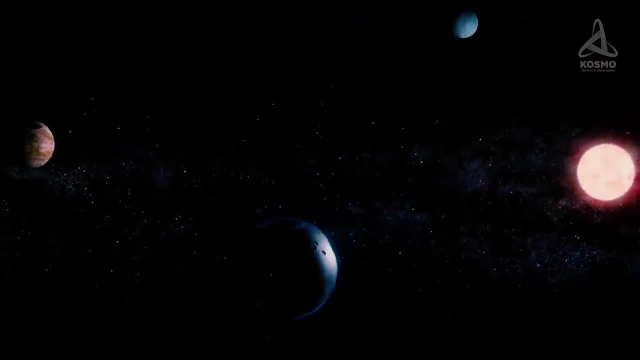 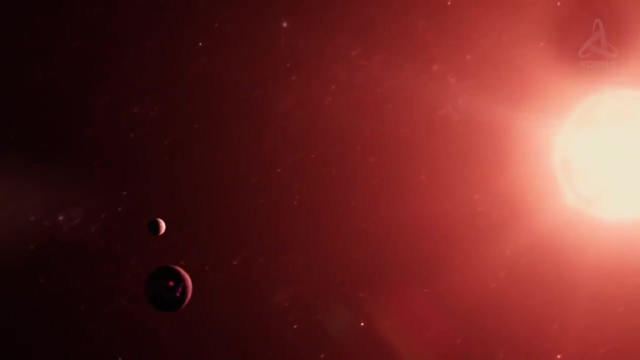 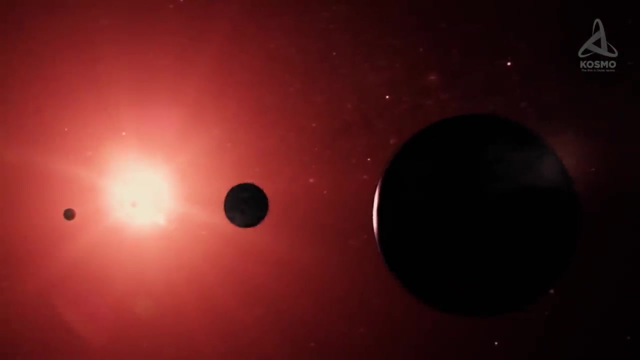 However, on closer inspection, the following principal differences will change the observer's mind about it. For a start, the smaller planets are closer to the star, with the bigger planets lying further and following bigger orbits. As we know, it's quite the other way around in the solar system, with the giants close. 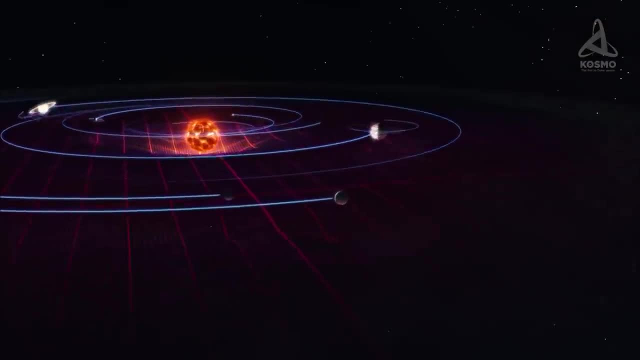 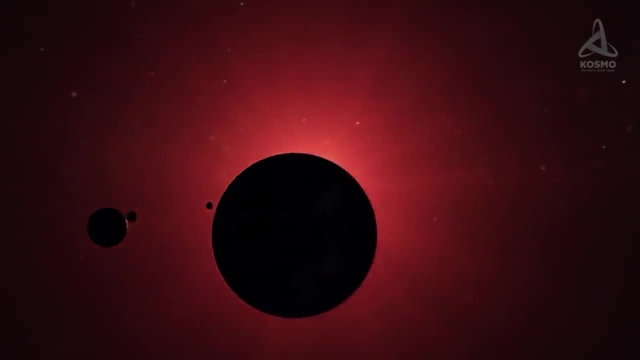 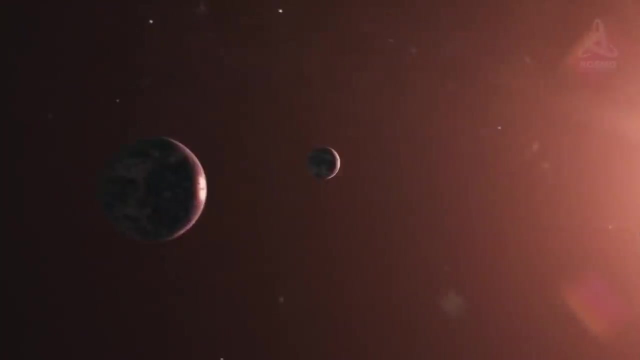 to the star and the smaller planets located further away. Admittedly, it is too early to claim this with absolute certainty, and the number of planets we know of in the Kepler-90 system may increase as scientists make progress in their observations. Another principal difference from our system shows in the planets' mutual proximity. the 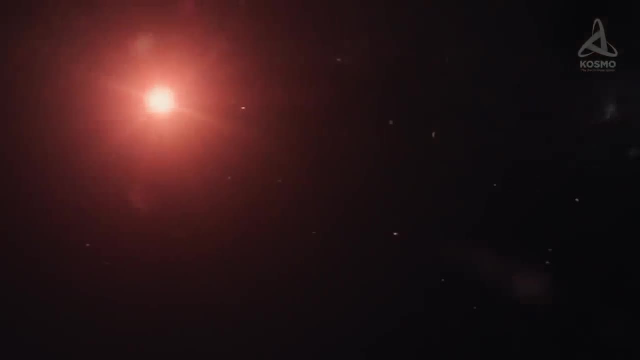 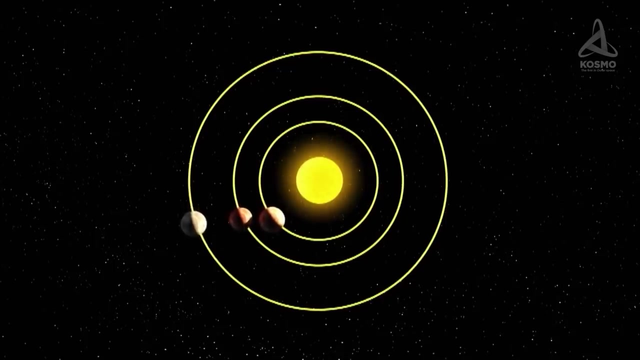 Earth and the other planets. The planets in our system, on the other hand, are located further away from each other, And also all the eight known planets in the Kepler-90 system orbit their star within just one astronomical unit. Another important difference is the fact that six internal planets in the Kepler-90 system 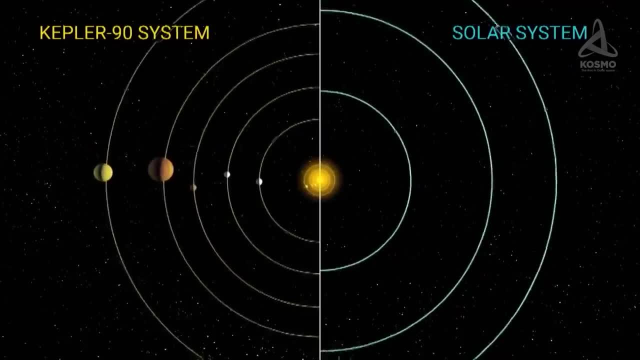 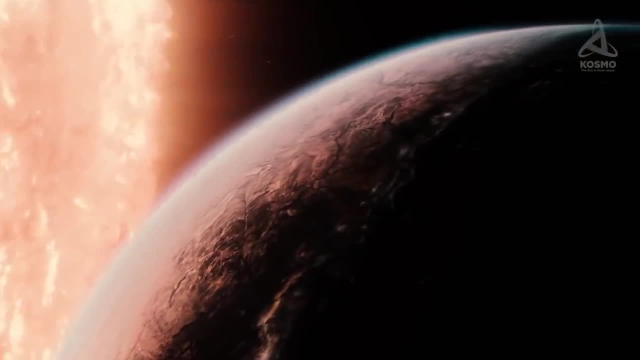 are either super-Earths or mini-Neptunes in size, while its two outer planets are gas giants. The two planets in the system lying closest to their host star, dubbed Kepler-90b and Kepler-90c, may probably be called our Earth's analogues. 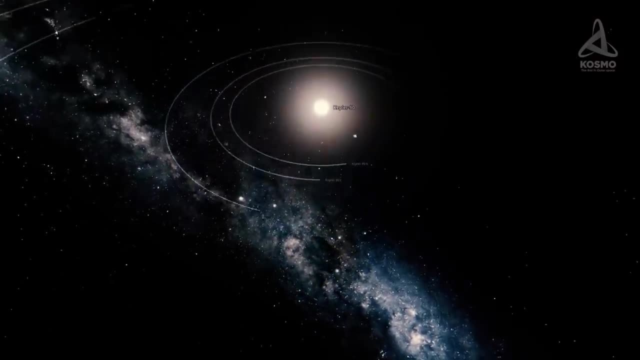 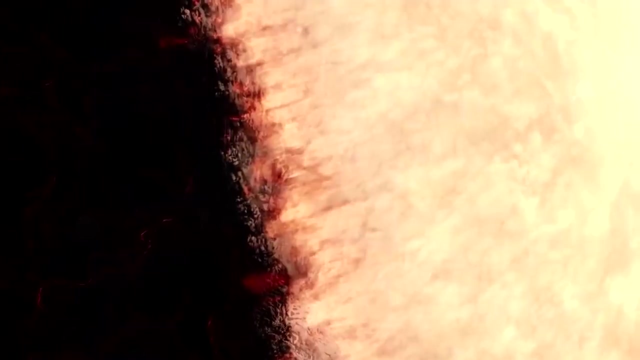 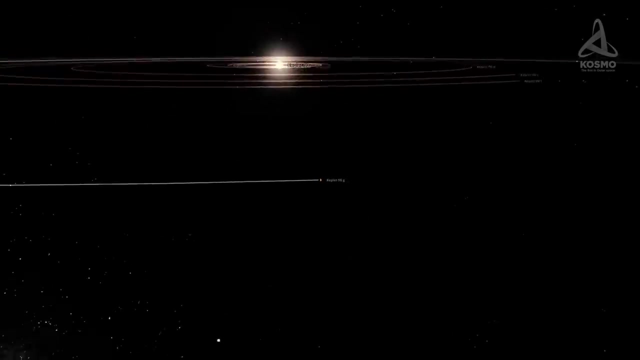 However, their temperatures are considerably higher than on Mercury or Venus, That is, the two planets closest to their host star in our solar system. This is the case on account of their proximity to their system's center. Kepler-90g and Kepler-90h are the objects lying furthest from their parent star. 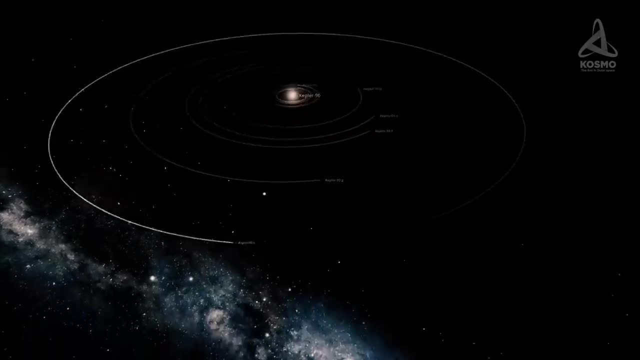 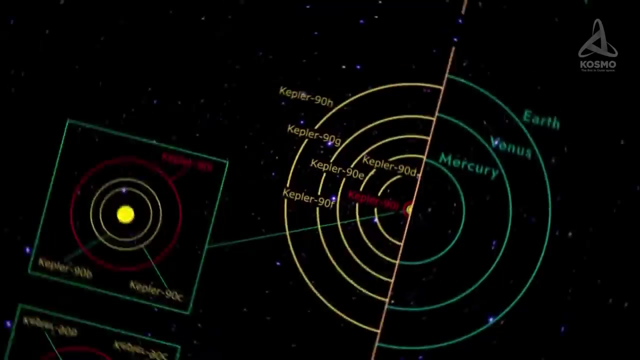 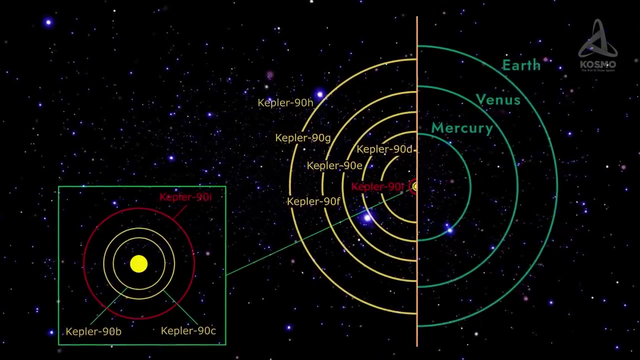 Both of these bodies are gas giants. Their dimensions must be comparable to those of Jupiter. The system leaves the general impression of being extremely compact. Even Kepler-90h, the remotest planet in the system, lies approximately as far as the Earth does from the Sun. 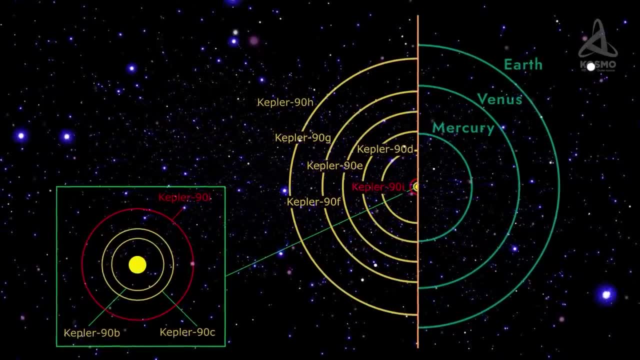 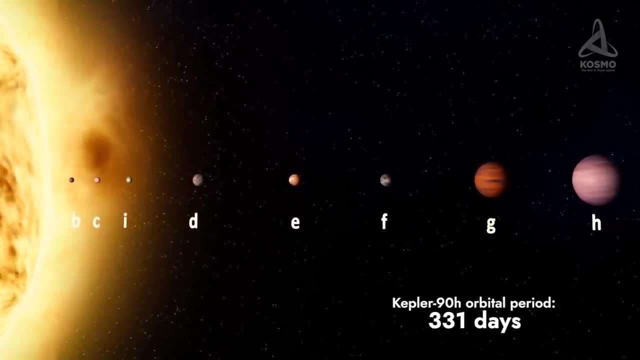 Also, as I have already mentioned, this remotest planet is also the largest in the system And a year on, it is almost as long as a year on our Earth- Three hundred and thirty-one days to be more exact. All these planets are comparatively smaller than the Earth. 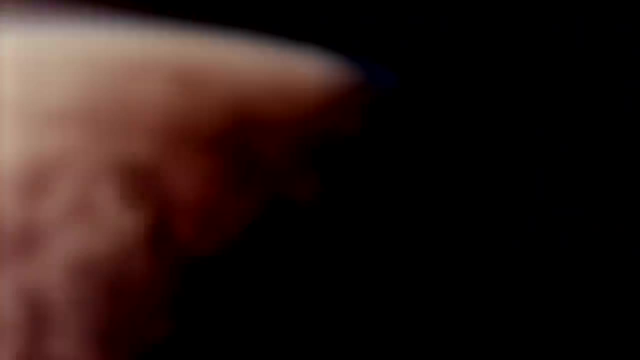 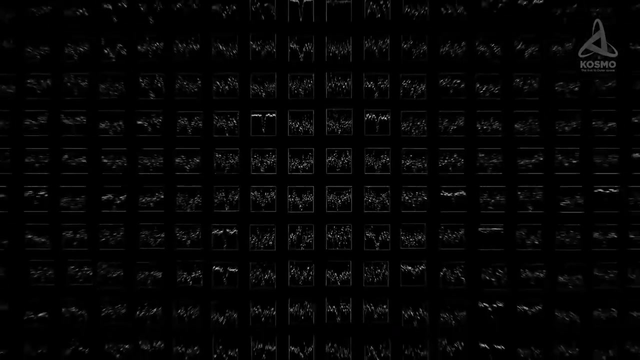 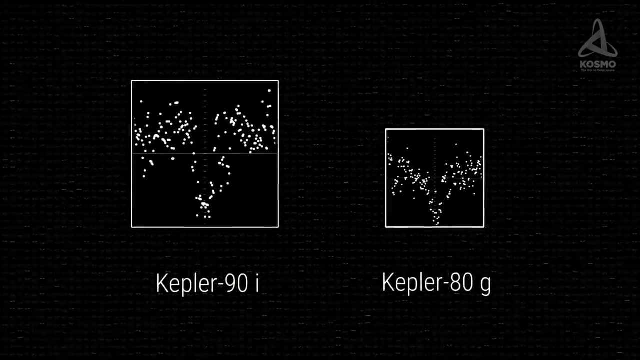 These planets were discovered not so long ago, with the latest of them, Kepler-90i, spotted as recently as in 2017.. It was possible to detect it with the transit method, that is, by observing sharp changes in the host star's luminosity when one or several planets pass across its disk and block. 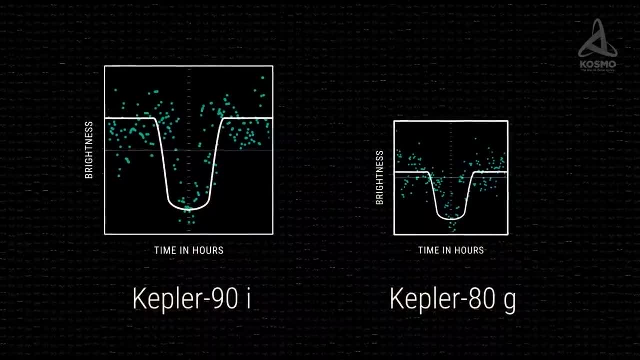 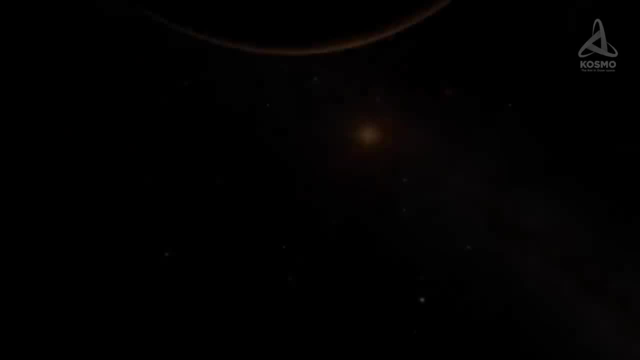 a certain portion of its rays normally visible to us. This method is quite productive for large celestial objects lying close to a star. However, if a planet is not visible to us, then it is possible to detect it with a transit method. However, if a planet is remote from it, fluctuations in the star's luminosity and other incidental 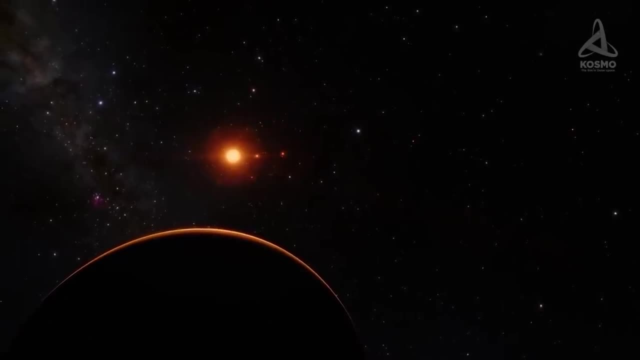 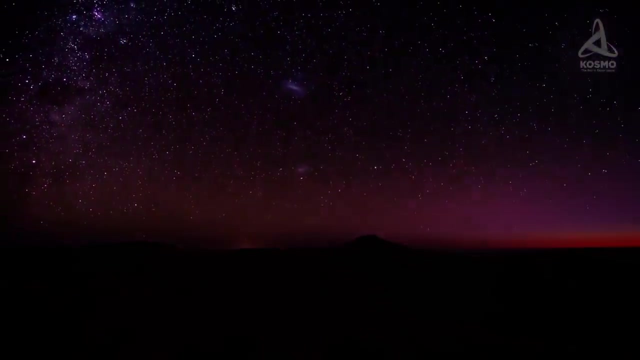 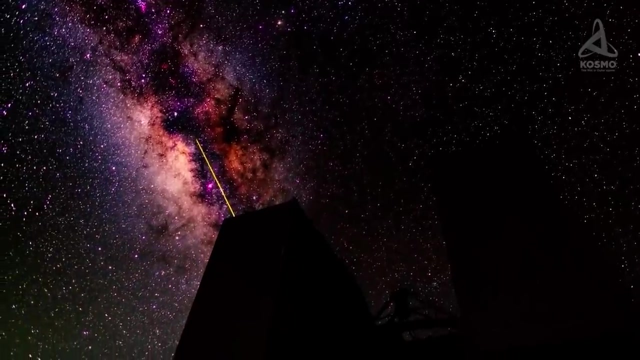 factors interfere with observations. These problems may be dealt with in two ways, namely by prolonging observation periods and by sorting data with the help of statistical algorithms and artificial intelligence systems. In fact, the latter helped the team of scientists studying Kepler-90 in discovering the eighth 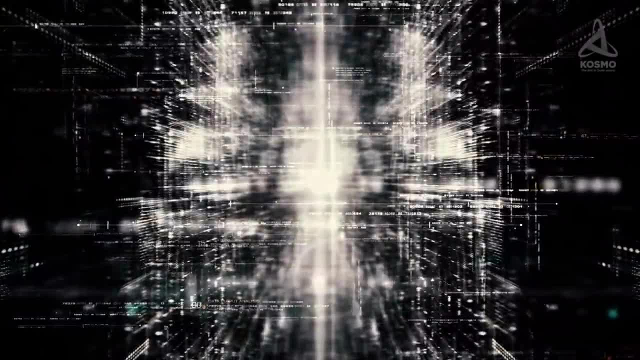 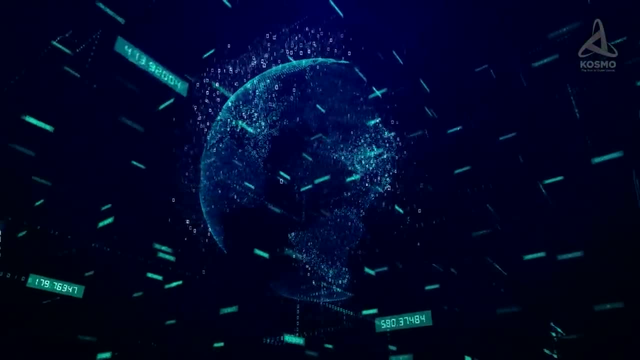 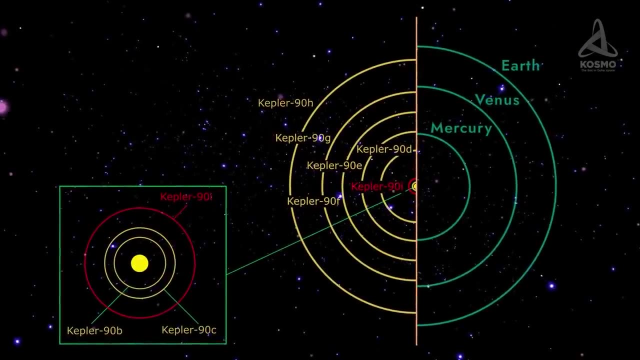 planet in the system Kepler-90i, the eighth planet in the system. This specially trained neural network was instrumental in pinpointing one more planet in the Kepler-90 system and defining its parameters. The newly spotted object was given the temporary designation Kepler-90i. 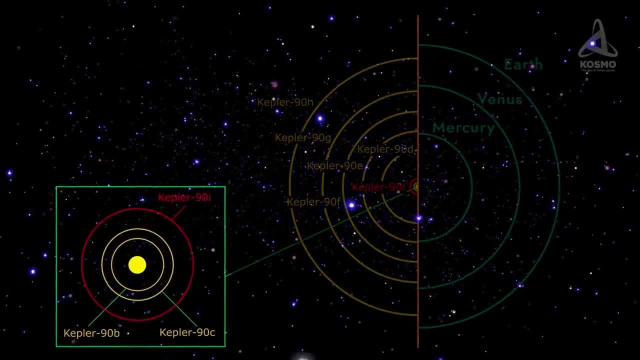 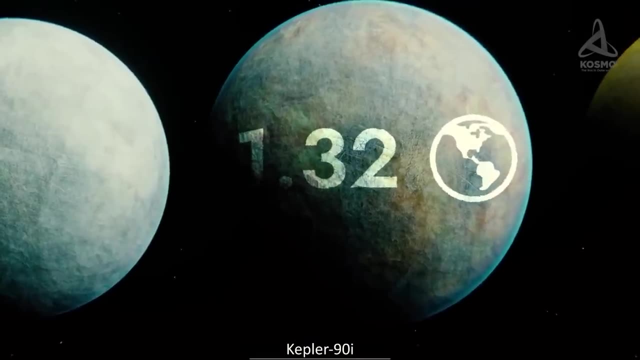 Located between Kepler-90c and Kepler-90d. this celestial object orbits its star within less than 15 days and its radius is 1.32 that of the Earth. Kepler-90i is three times closer to its star than Kepler-90d. 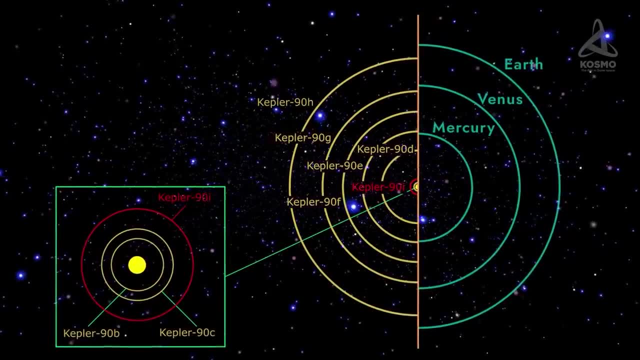 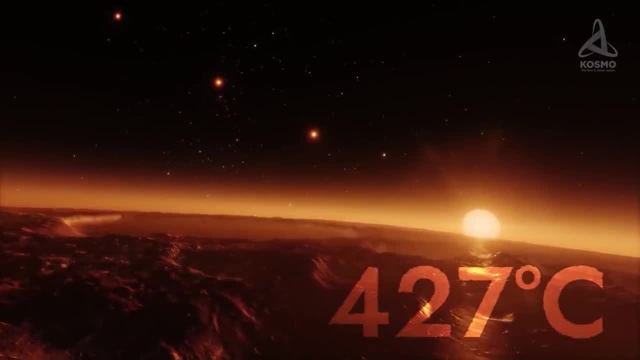 Kepler-90i is three times closer to its star than Kepler-90d. This is because the visual field that is shown in this image is not more than one percent closer to its star than Mercury is to the Sun. That is why its surface temperature is rather high, approximately 427 °C. 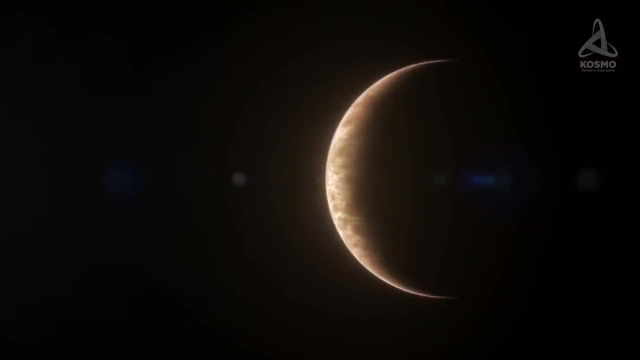 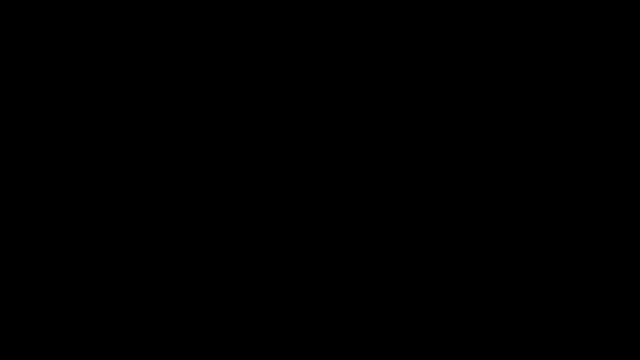 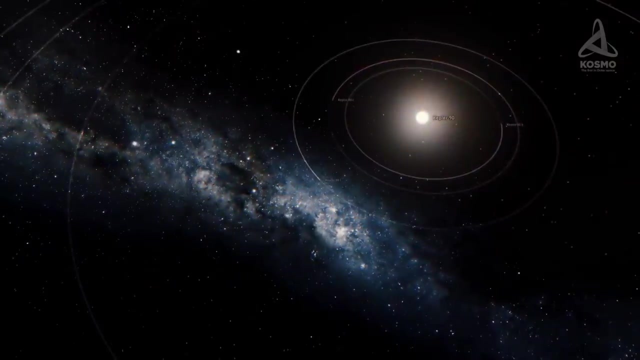 Just to compare, this value is quite close to the surface temperature of Venus, which is 477 °C. Kepler-90i resembles our Earth very much in terms of its chemical composition, size and mass. Its orbital period is 14.4 Earth days. 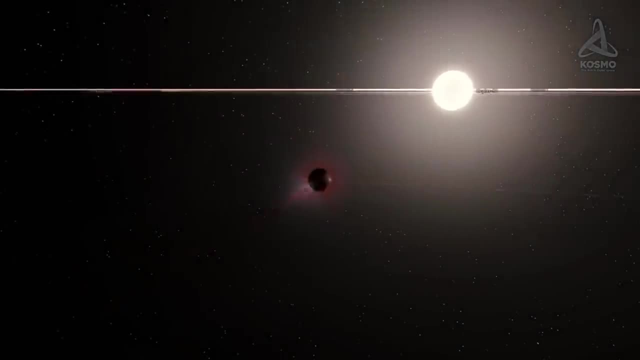 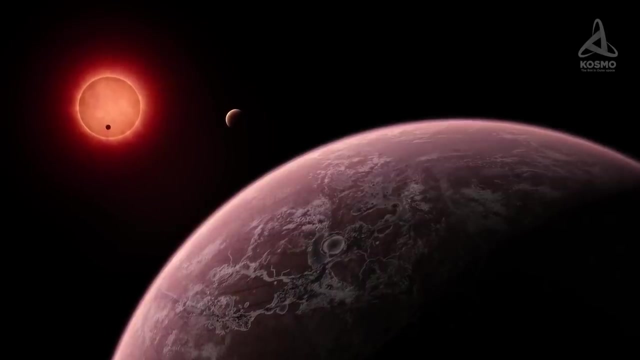 As the planet lies too close to its parent star, it cannot realistically support life. The discovery of this celestial object prompted a lot of questions on the part of the scientific community. It still remains to be found out how such a large and complex planetary system managed. 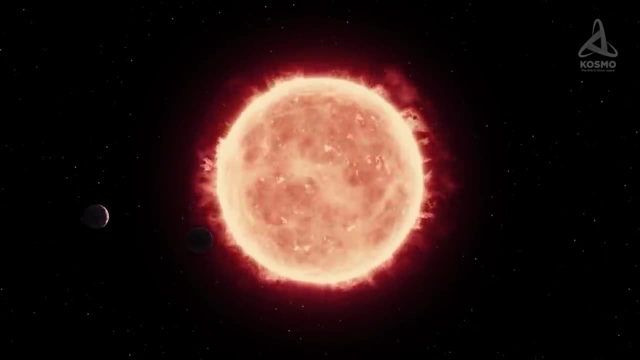 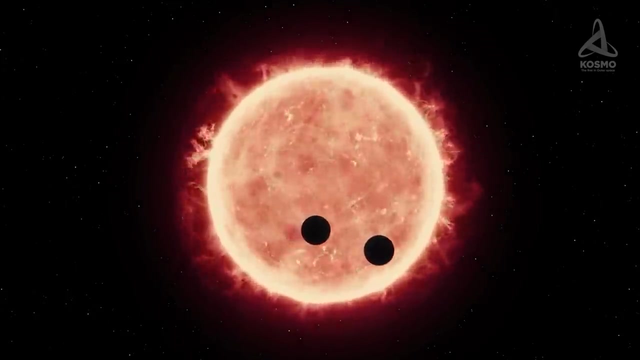 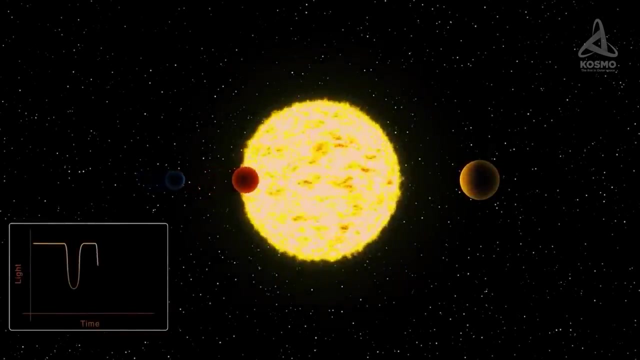 to remain so compact and stable at the same time. Also, astronomers assume there might be more planets out there orbiting Kepler-90, which still remain to be discovered. The search for other bodies in this system is still on. As for the other known planets in the system, the parameters of each are unique in their 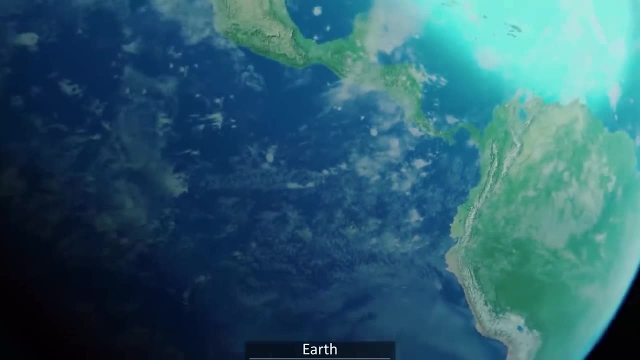 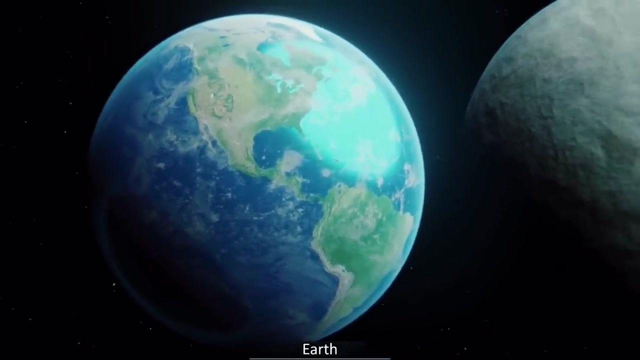 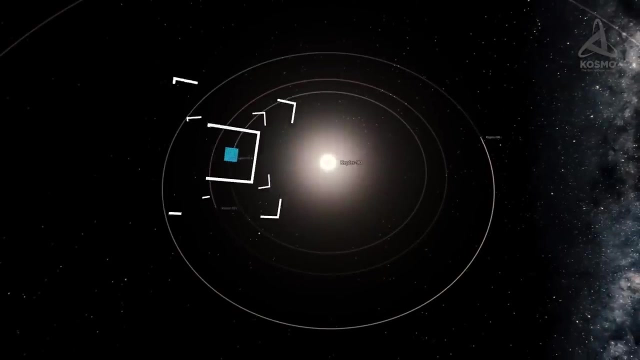 own way. Let's have a look at them, starting with the planet closest to its star. The radius of the one nearest to its parent star, Kepler-90b, measures about 1.3 times that of the Earth, And its orbital period lasts for 7 days. 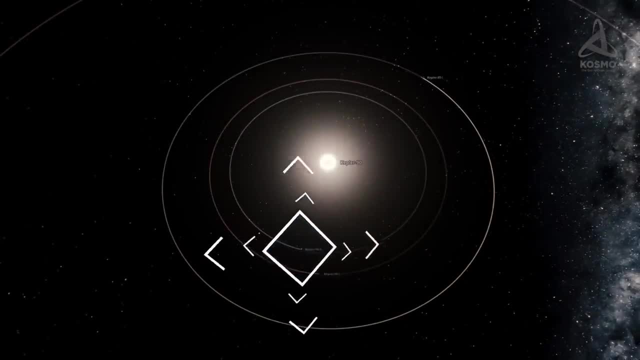 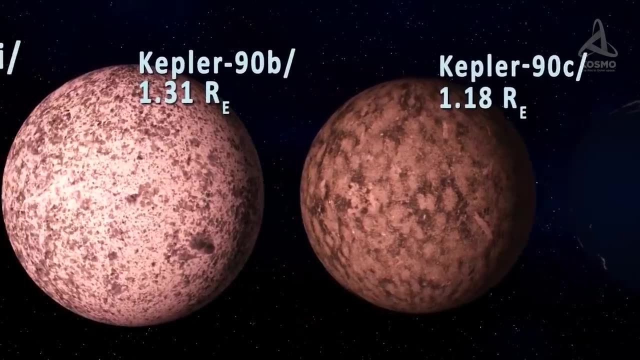 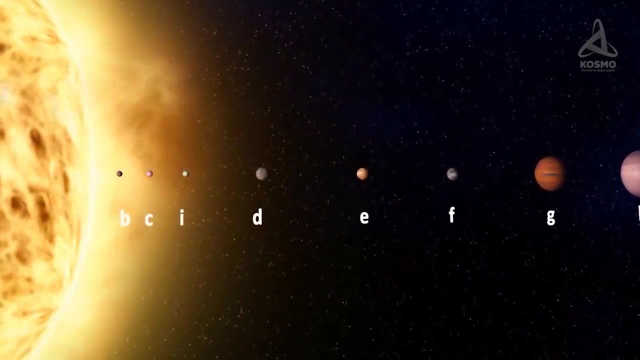 Just like all the other objects in the system, except Kepler-90i, it was detected back in 2013.. The planet coming next orbiting its parent star, slightly further away than Kepler-90b, is Kepler-90c. Its radius is slightly smaller, measuring 1.19 times that of the Earth. 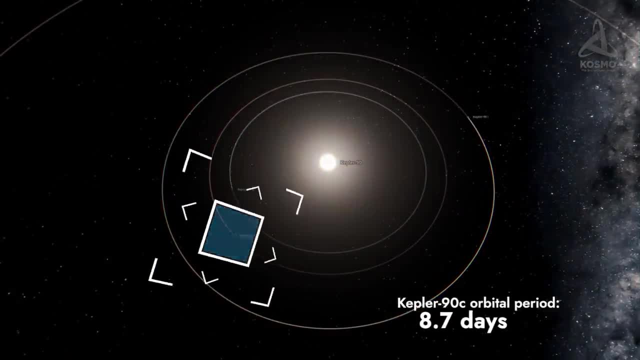 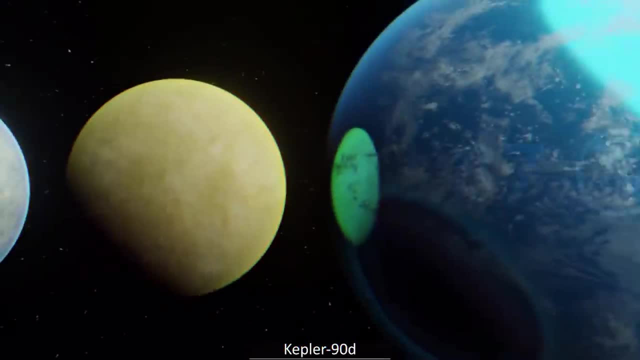 And as for its orbital period, it is 8.7 days. The fourth known object in terms of its closeness to its star is Kepler-90d. With its radius measuring 2.87 times that of the Earth, it orbits Kepler-90 within a 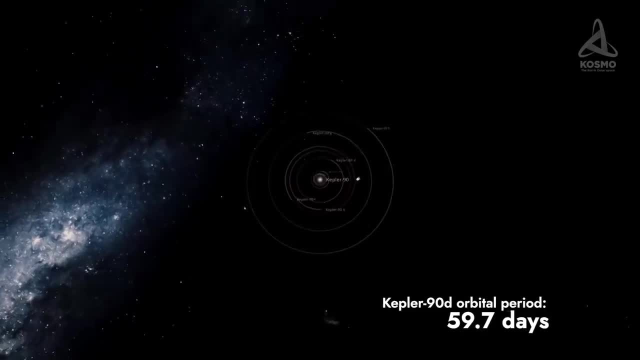 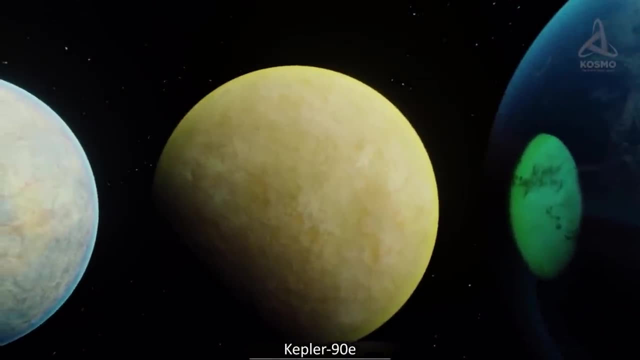 period of 59.7 Earth days. Kepler-90e holds the 5th place. Its radius is 2.66 that of our planet, and its orbital period may reach 91.9 days. Kepler-90e is the fifth place. 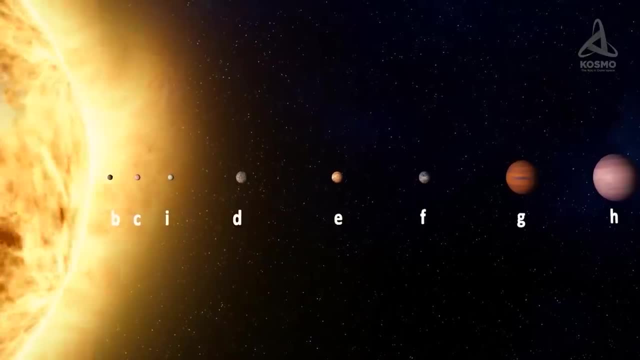 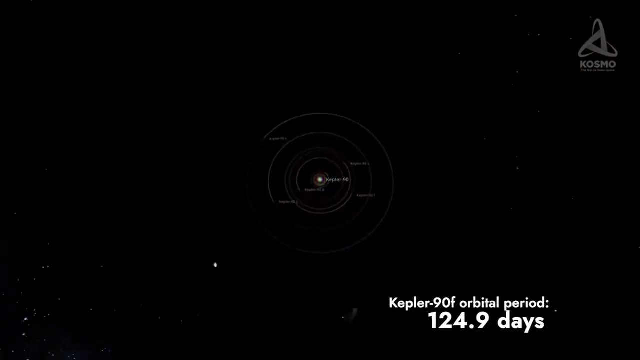 The radius of Kepler-90e is 2.66 that of the planet, And its orbital period may reach 91.9 days. Kepler-90f comes next. Its radius is 2.88 times that of the Earth and its orbital period is 124.9 Earth days. 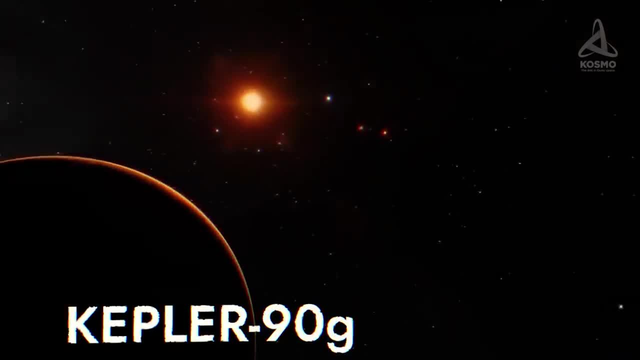 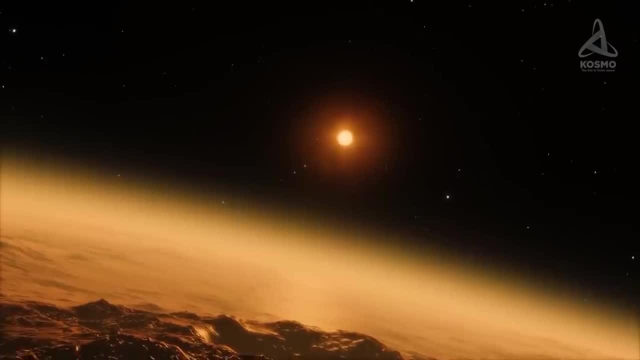 After Kepler-90f comes Kepler-90g, with a radius measuring 8.1 times that of the Earth, Its orbital period is 210.5 days and its mass is approximately 0.8 times that of Jupiter. Kepler-90f is the fifth place. 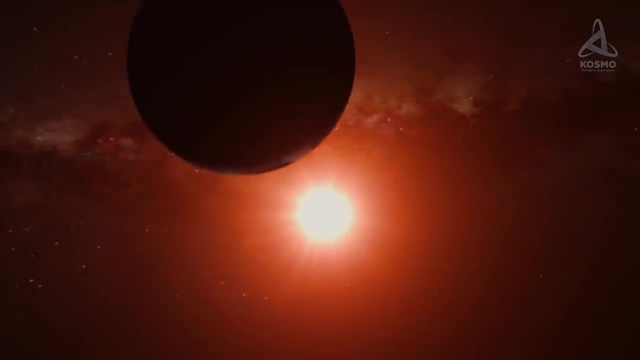 Kepler-90g is the sixth place. Kepler-90g is the seventh place. Kepler-90emo h has a radius measuring 11.38 times that of the Earth, Its orbital period is 331.6 Earth days and its mass is about 1.2 times that of Jupiter. This means that Kepler-90I is one of four stars in blijvig ح permanently счетан U overlooked to have a constant 8.8 ils-pound radius. at the time when Kepler-90g was discovered- The future of the earth, zucchini. the planet would measure 331.6 Earth days, as they were. 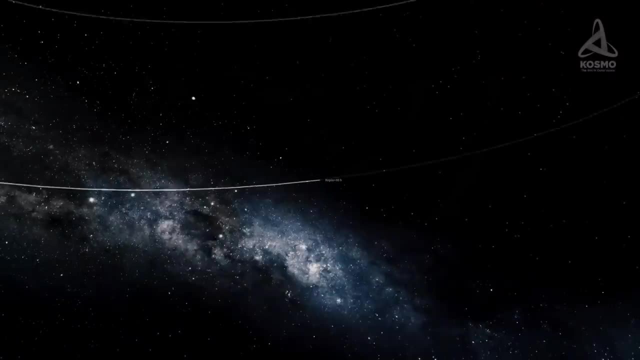 оз opens the 영상을 in the description below this video to answer your questions asked by Keplr-90f, This means that Kepler-90h is about 1.2 times that of Jupiter. From that quant Flip optimism is only decimal point 9.. 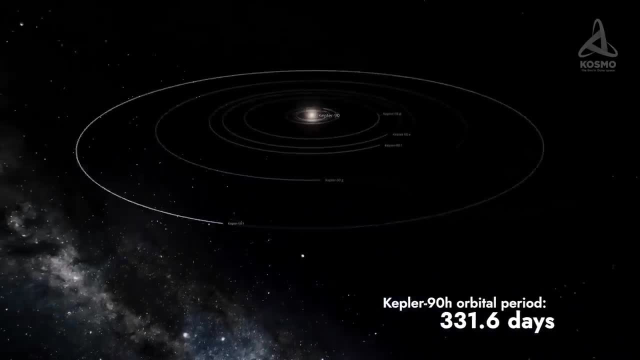 우리� olig스트� 150000mg du adaν, Without establishing the orbitof this suborbobe. er entonces astra개 cem sida, 6.0, six Earth days, and its mass is about 1.2 times that of Jupiter. 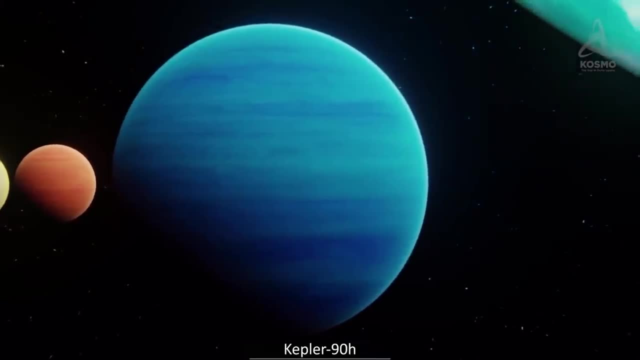 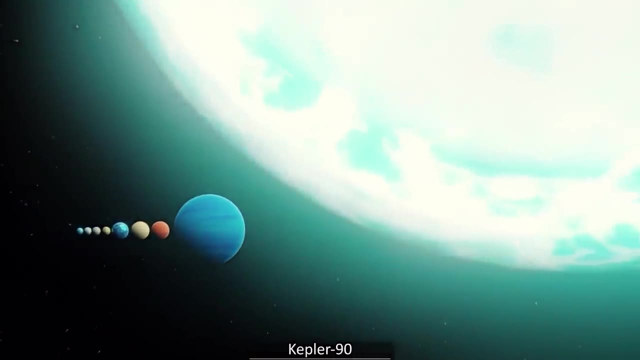 As this object's orbit lies approximately as far from its star as that of the Earth from the Sun, assumptions about the presence of hypothetical moons in its environs may prove to be true If there are any located close to Kepler-90h that are similar to Titan or Ganymede in their 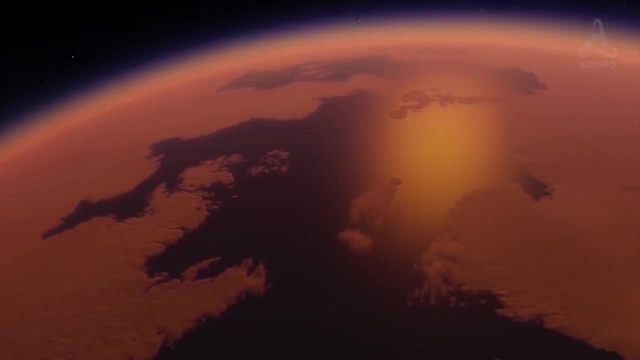 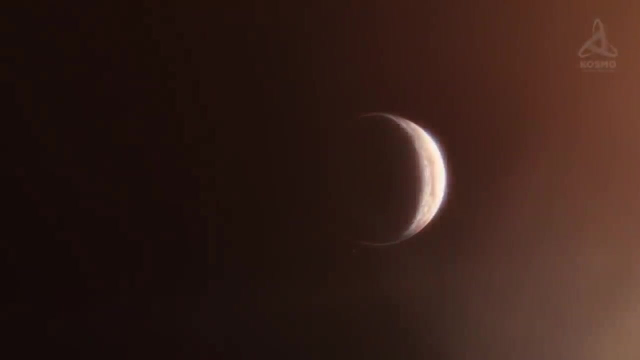 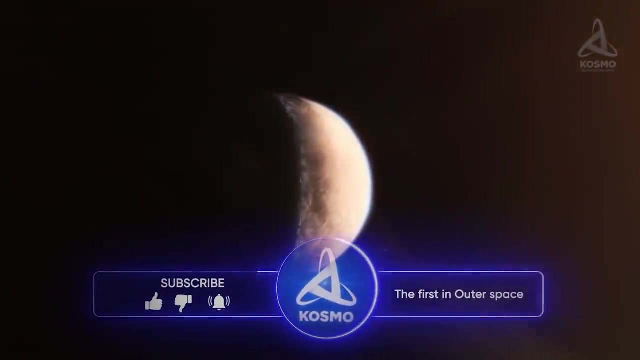 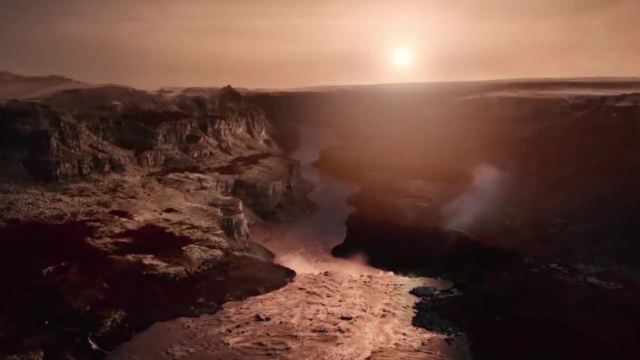 parameters, conditions on these moons may be realistically suitable for life. These hypothetical celestial objects might have some really incredible features. As their planet lies on the habitable zone of its star, some of these moons may well resemble our Earth For all we know. just as you are watching this video on the Cosmo Channel, a new life. 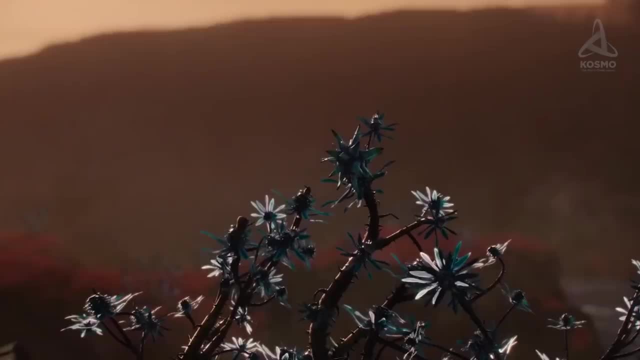 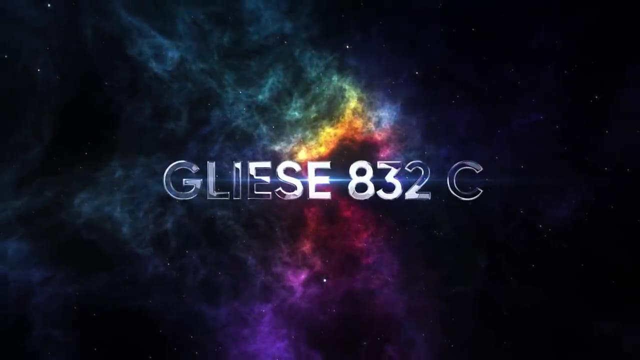 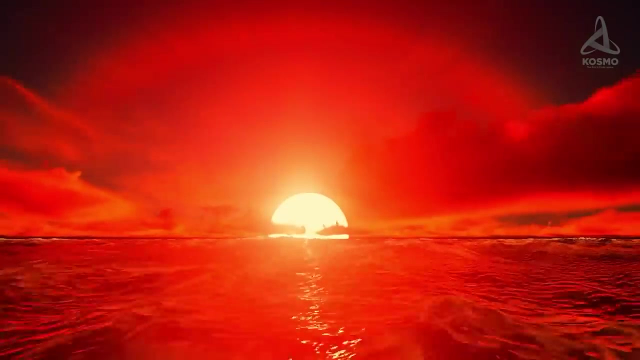 may be dawning on a moon of the faraway gas giant Kepler-90h. This is a kind of landscape one would see in the least harsh part of a planet dubbed by scientists as Super Earth and the closest potential candidate suitable for searching for alien life forms. 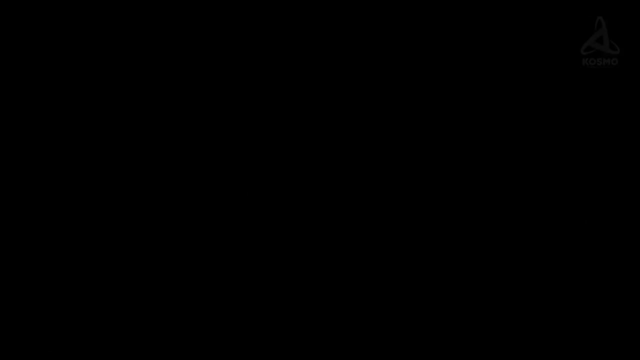 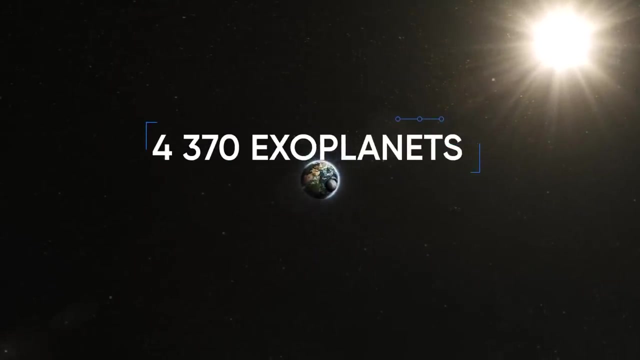 But let's be consecutive. The recent past heralded a boom in discovering exoplanets. There are 4,370 exoplanets discovered in over 3,000 planetary systems so far. In addition to these, more than 3,000 exoplanets have been discovered in the past. 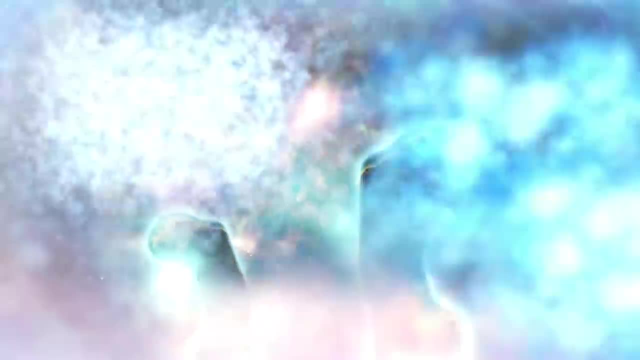 In addition to these, more than 3,000 exoplanets have been discovered in the past. In addition to these, more than 3,000 exoplanets have been discovered in the past. More than 3,000 objects are awaiting confirmation of their exoplanet status. 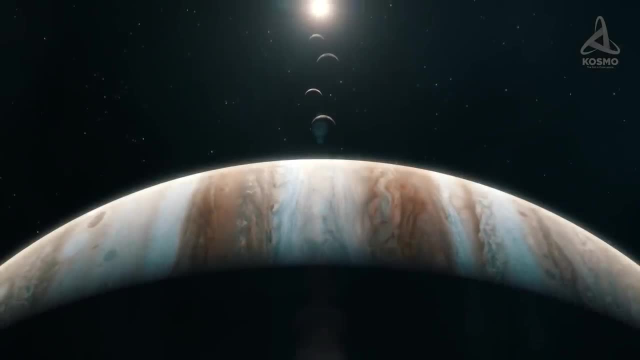 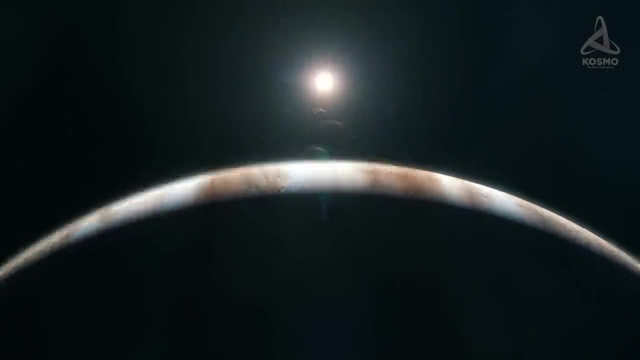 Most of them are large bodies – gas giants, super-Jupiters and super-Earths. This is accounted for by technical features of the technologies used for the purpose. It is easier to look for massive bodies with a short orbital period than to try to spot. 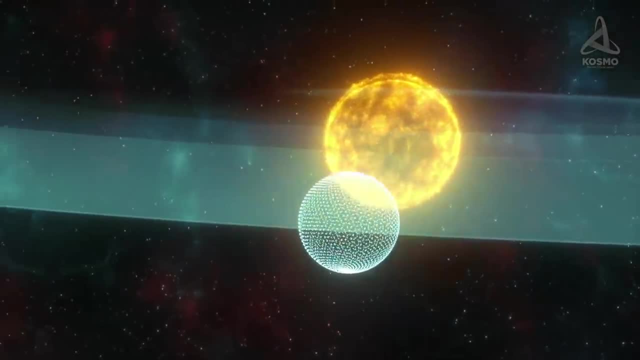 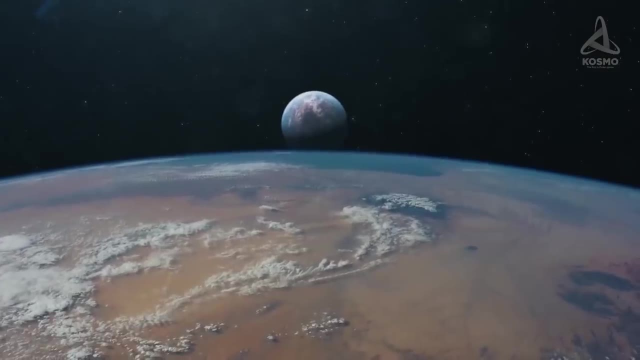 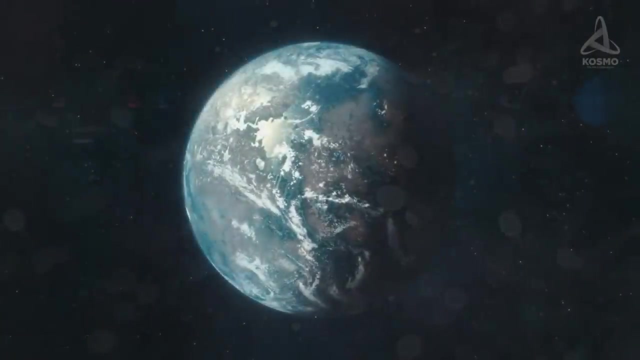 smaller planets similar to the Earth or Mars in terms of dimensions. There are among exoplanets those that may realistically harbour life. There are dozens of these objects scattered in space, and they understandably draw scientists' close attention. Today, we are going to look at one of these objects, which is an exoplanet dubbed Gliese. 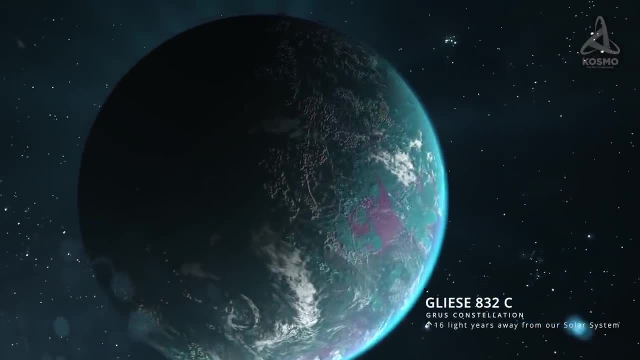 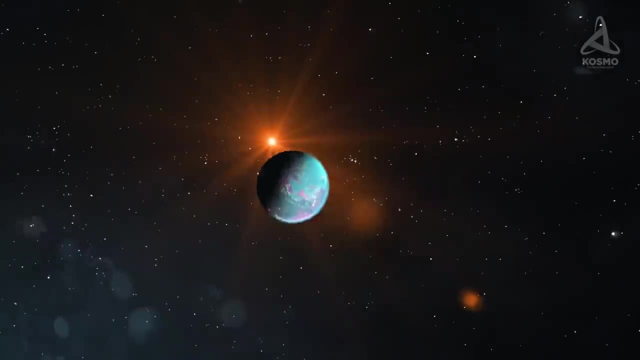 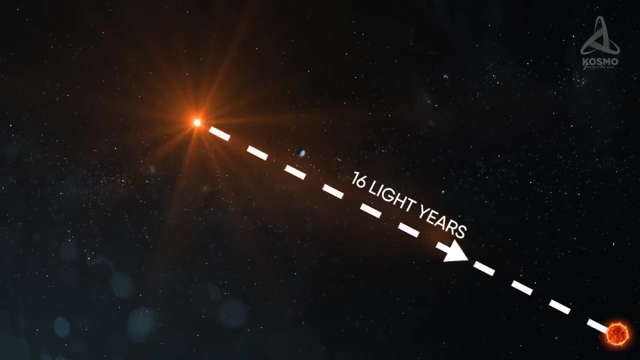 832c. In fact, this exoplanet is one of the most likely places where alien lifeforms will eventually be detected. This exoplanet orbits a star called Gliese 832,, which lies 16 light-years away from the Sun and is part of the Grus constellation. 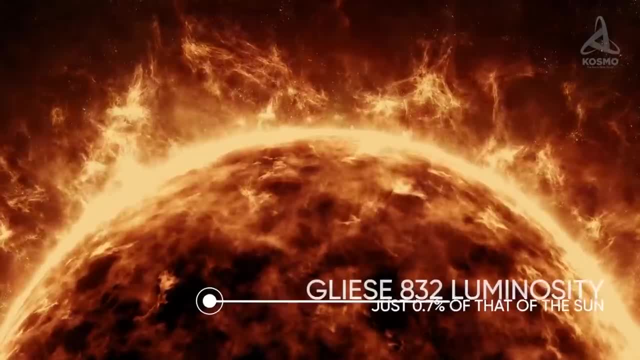 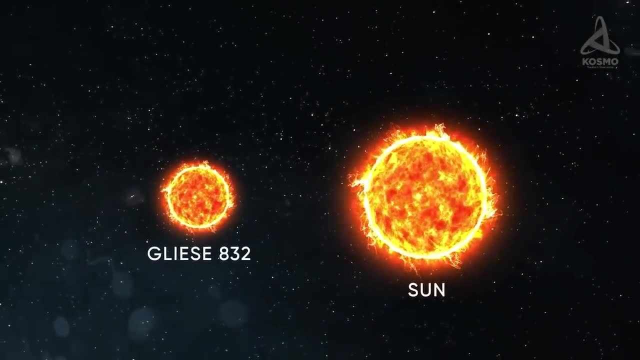 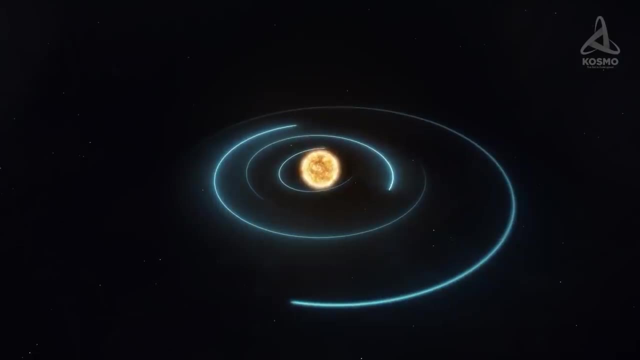 Gliese 832 is a dim red dwarf whose luminosity is just 0.7% of that of the Sun. Both its mass and diameter are approximately two times smaller than those of the Sun, and its temperature reaches about 3300 degrees Kelvin. 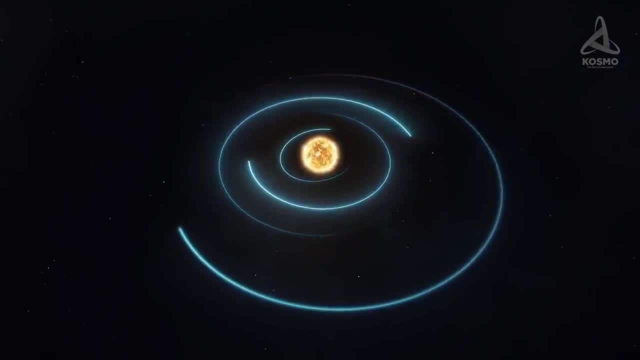 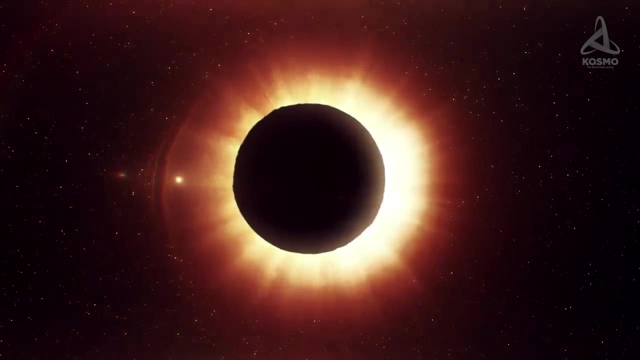 That is the reason why the habitable zone of this planet is within quite a short range from its star. Due to tidal forces, the planets lying in the habitable zone are not able to reach the star. The habitable zone of Gliese 832 will be tidally locked to their star, that is, will face the 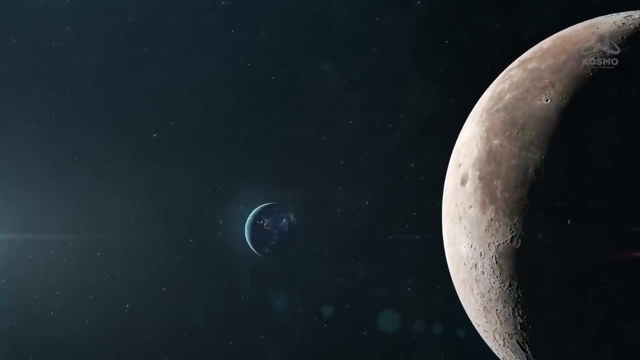 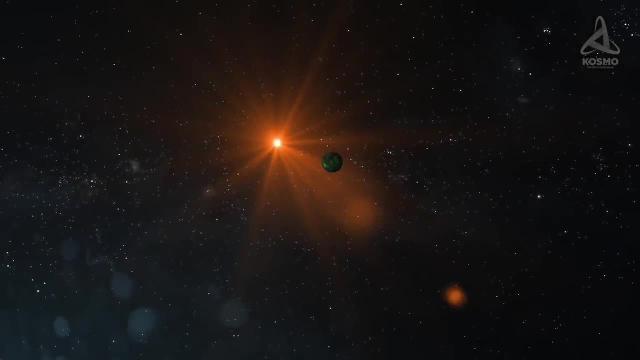 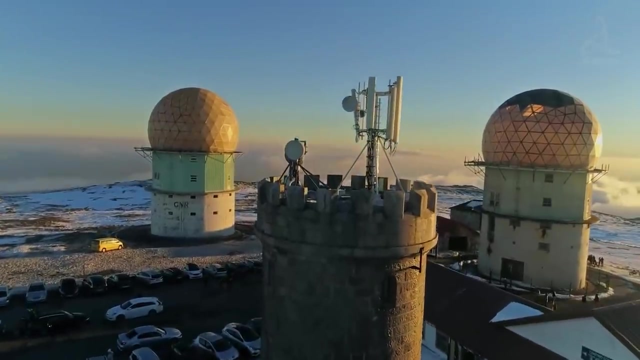 star with one side only, just as it is the case with the Moon and the Earth and Mercury and the Sun. There are two confirmed planets orbiting, Gliese 832.. The Jupiter-like planet Gliese 832b was discovered first. Astronomers announced the event in 2008.. 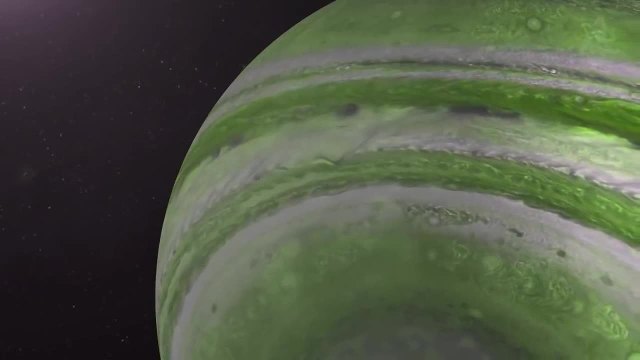 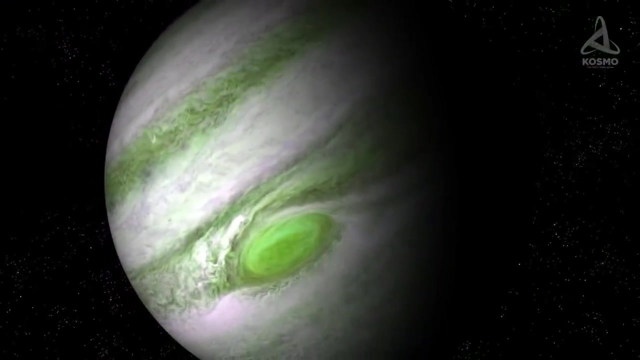 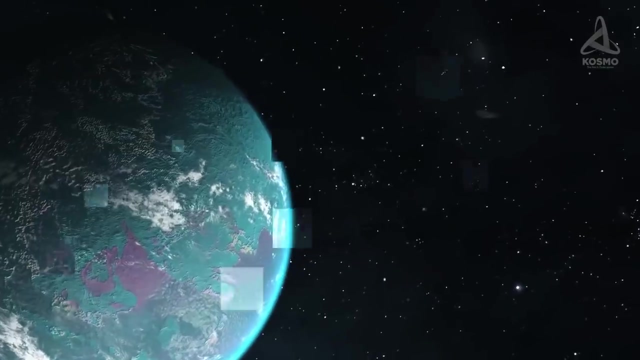 With the mass two-thirds that of Jupiter. the planet orbits its parent star at a distance of an average 3.4 astronomical units, completing a full orbit every 9.4 Earth years. The discovery of the other confirmed planet, Gliese 832c, was announced in 2015 by an international 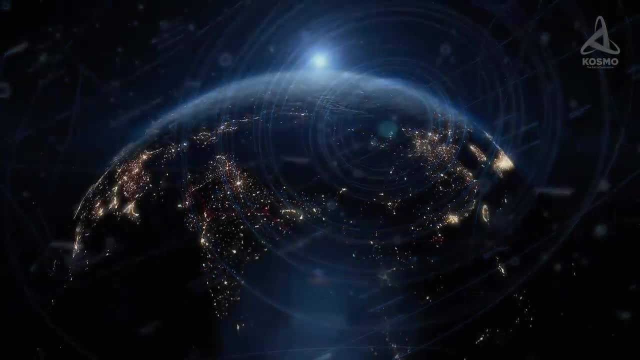 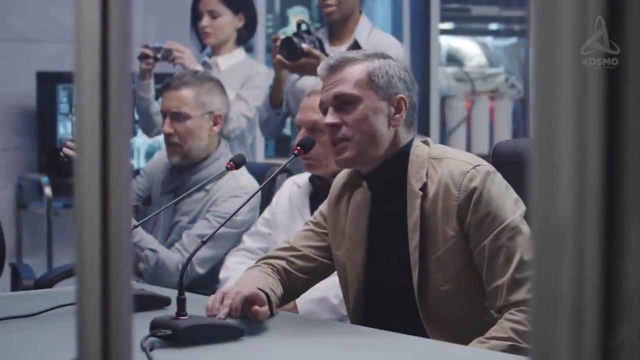 team of scientists headed by Robert Wittenmeyer. It got an exceptionally high rating for its similarity to the Earth- 0.81 to be more exact- which instantly attracted both scientists and reporters. It was also nicknamed as the Earth-like planet. It was also nicknamed as the Earth-like planet, Even though the two planets' parameters are rather different Either way, this is one of the planets closest to the Earth with such a high Earth similarity index. The mass of Gliese 832c is five and a half that of the Earth. 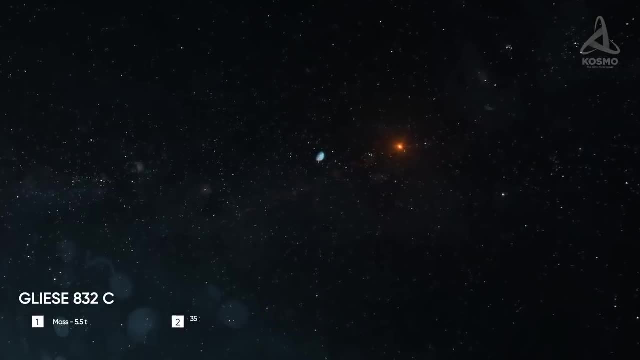 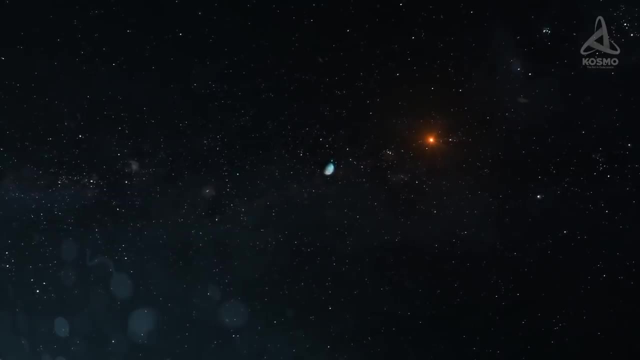 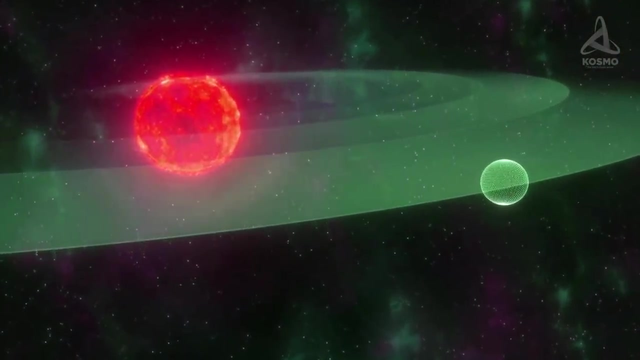 It takes the planet 35 Earth days to complete a full orbit around its parent star, moving at a distance of an average 0.16 astronomical units, less than the distance between our Earth and the Sun. Its orbit's eccentricity is rather high, with the planet regularly leaving the habitable. 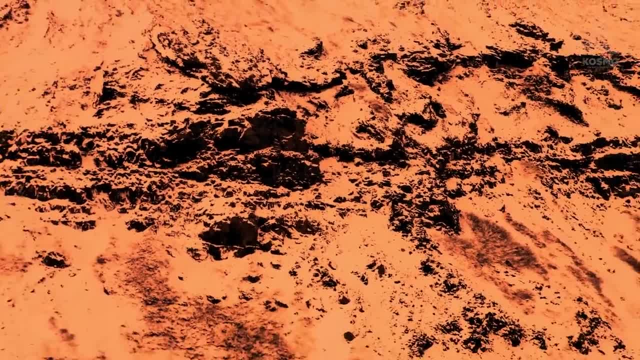 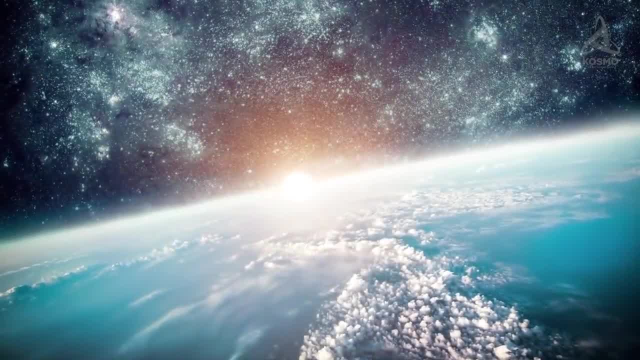 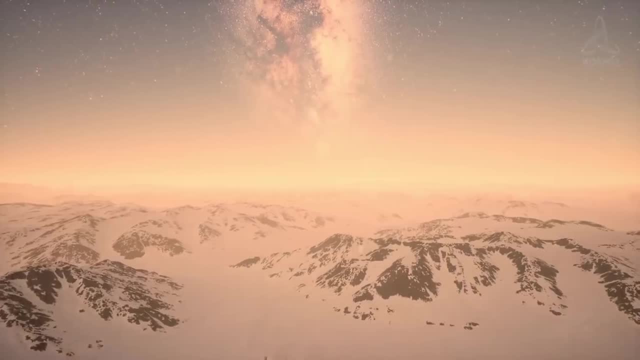 zone and then re-entering it. This must cause sharp temperature leaps and drops on its surface. Gliese 832c is estimated to receive approximately as much energy flux from its parent star as does the Earth from the Sun. The average surface temperature on the planet is 253 degrees Kelvin, or 20 degrees Celsius. 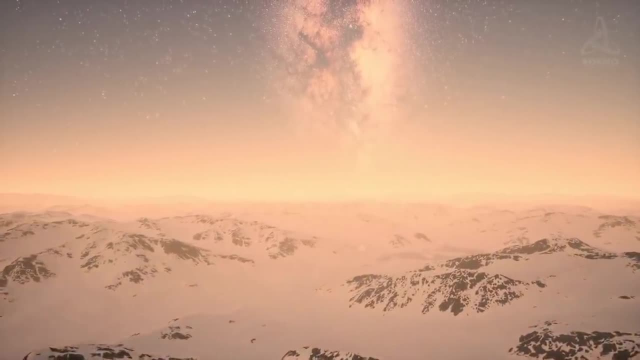 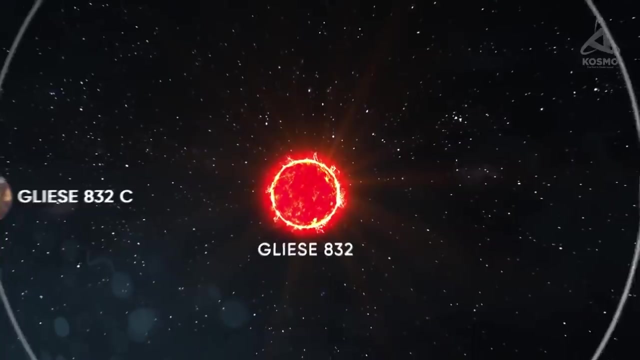 below zero. It is also suggested that, due to the atmosphere, which is likely to be quite dense, the temperature on the planet may be considerably higher. However, it is not easy to claim this with certainty, as Gliese 832c lies quite close. 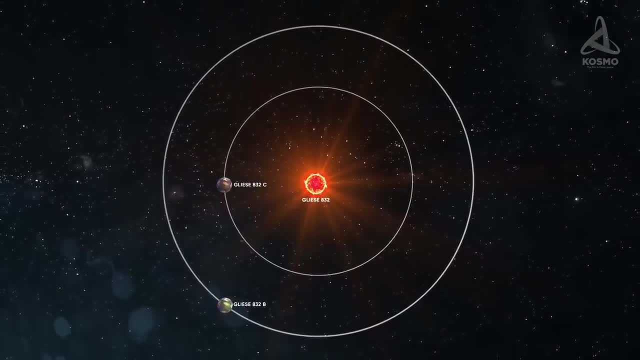 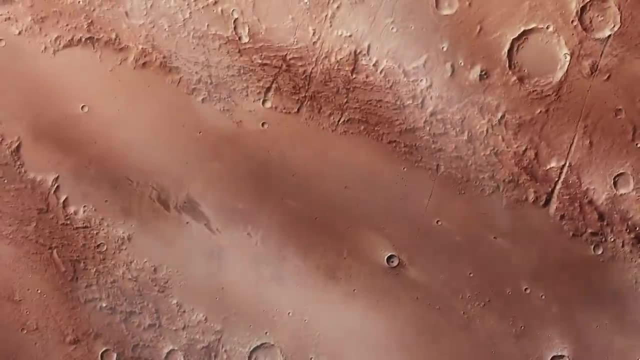 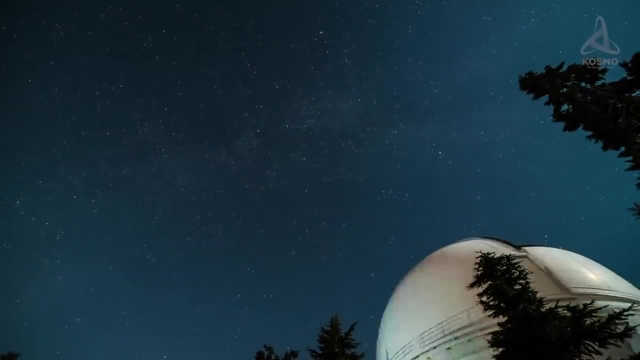 to its star, and so chances are it is firmly tidally locked to it. In this case, there should be a substantial temperature difference between its sunny side and shadow side, which should regularly cause hurricane winds if the atmosphere really is dense. It is worth mentioning that in 2017, following observations astrophysicists from the University 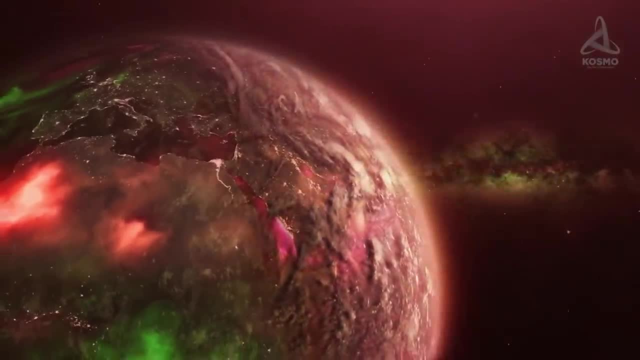 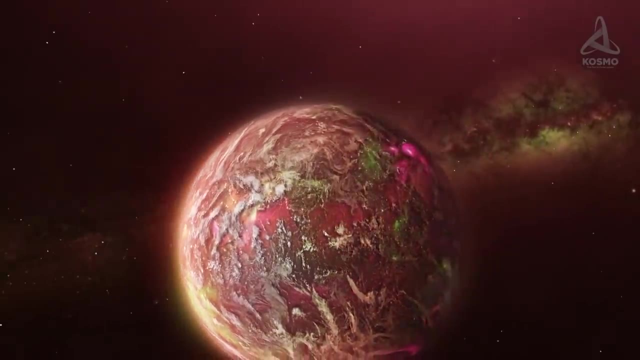 of Texas. at Arlington, the USA put forward the hypothesis that there may be a third planet in the Gliese 832 system. Its mass could be 1 to 15 Earth masses and it could follow a stable orbit around the center of the system, 0.25 to 2 astronomical units away from it. 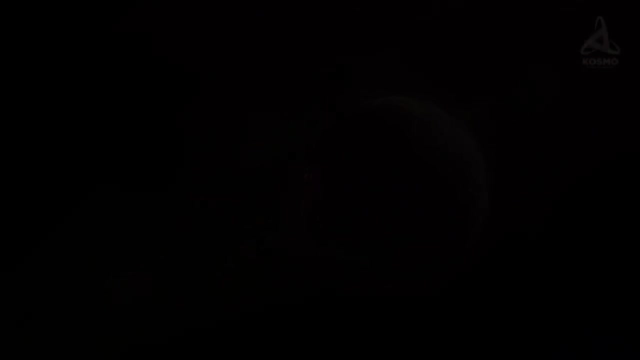 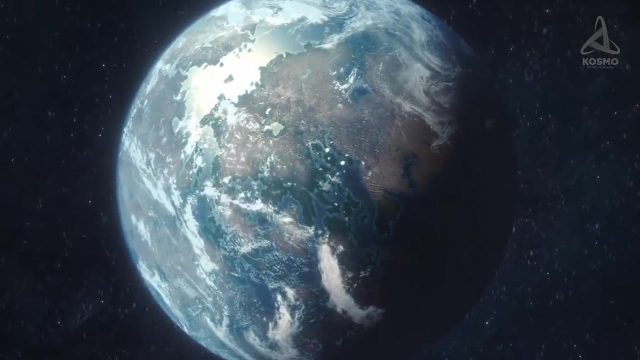 However, this is not the case At the moment the planet is being searched for. Let's imagine what Gliese 832c would look like, assuming life were possible on this planet. First of all, we wouldn't help noticing its gravity, which would be strikingly higher than that on our Earth. Since the planet's diameter is not yet known, the gravity force cannot be calculated exactly. Still, it would be a rocky planet, similar to our Earth and Earth-like planets in terms of its density, So its gravity force would be likely to reach 2 to 400% that of the Earth. 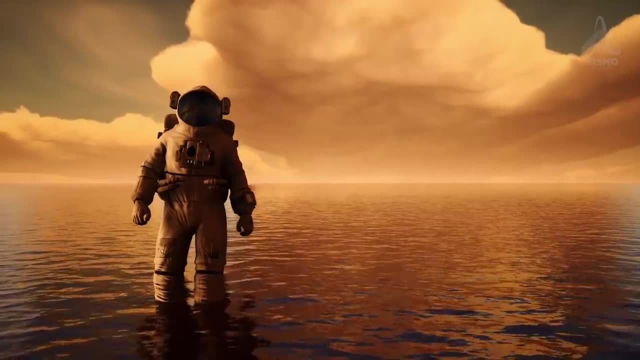 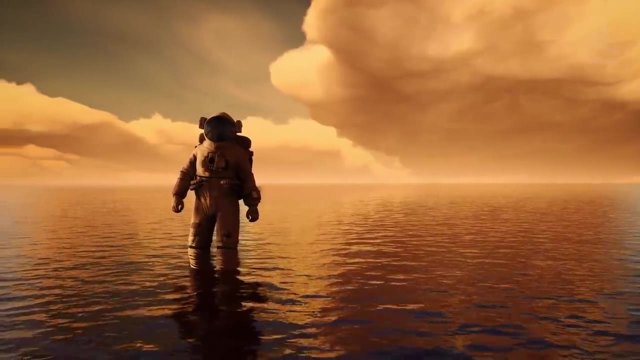 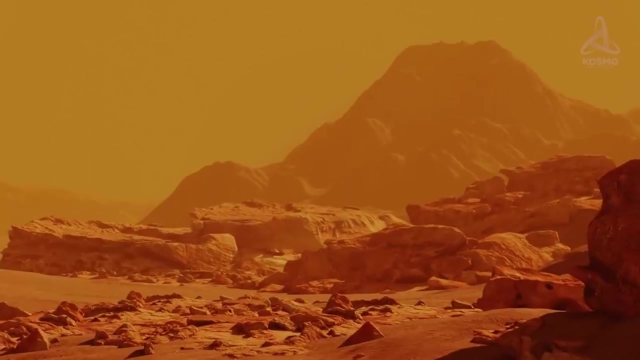 This would lead to the relief leveling out, meaning that the mountains would not be so high and the oceans not so deep. This, in its turn, would enhance the area of warm water, which is favourable for life. Due to a dense atmosphere and a comparatively dim sun, the landscape on Gliese 832c would 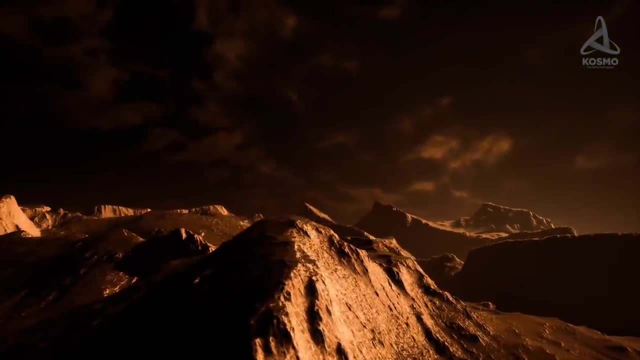 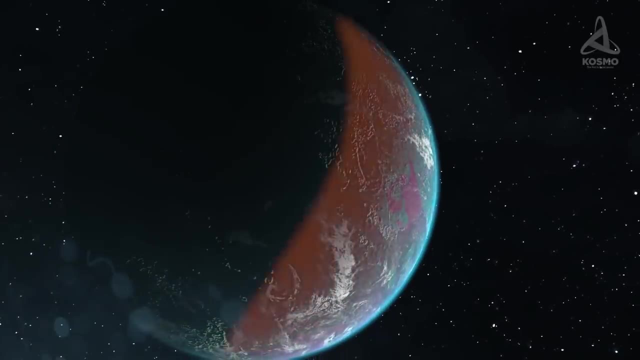 be of a reddish hue and, in general, the planet would be submerged in semi-darkness. Since the planet is likely to face its star with the same side at all times, the temperature on the sunny side should be high and the temperature on the shadow side quite low. 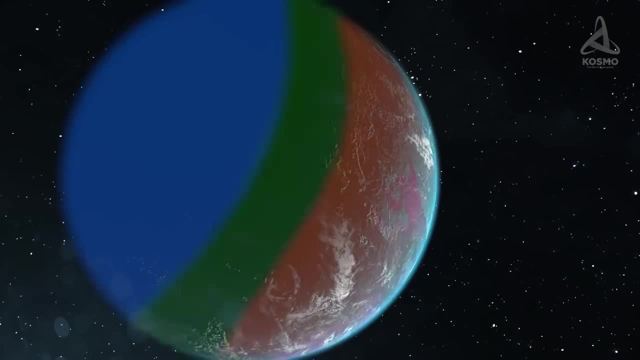 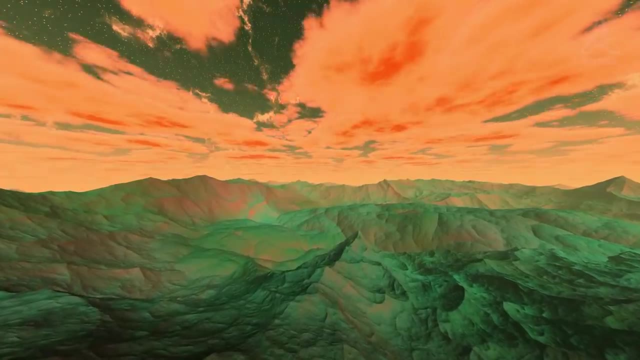 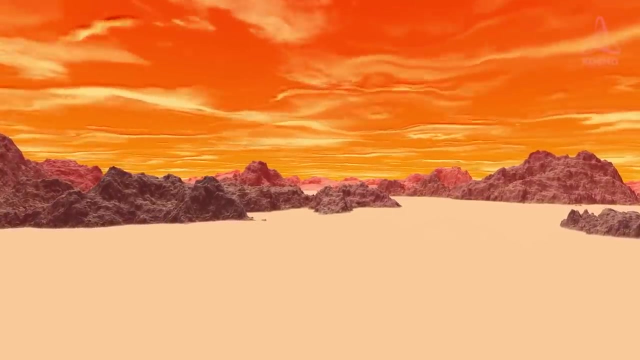 In the ring-like area at the border between them. the temperature should be moderately comfortable, although, due to irregular heating of the planet, the atmosphere would be constantly in turmoil, which should result in strong winds. In addition, high objects of relief potentially able to dissipate some of the force of hurricane-air. 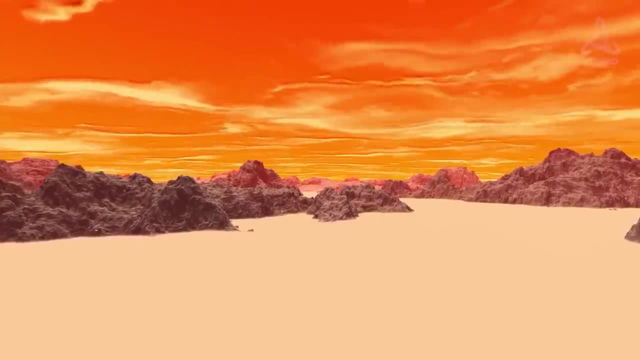 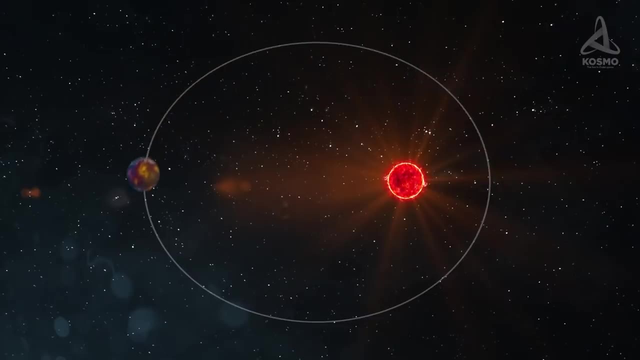 currents. This is due to the high gravity conditions. As the orbit of Gliese 832c is small and elongated, seasons on this planet should change every week. It will be winter on Gliese 832c at the furthest point from its parent star, and summer at the 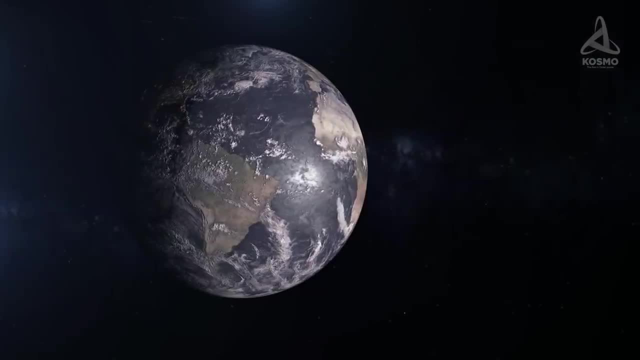 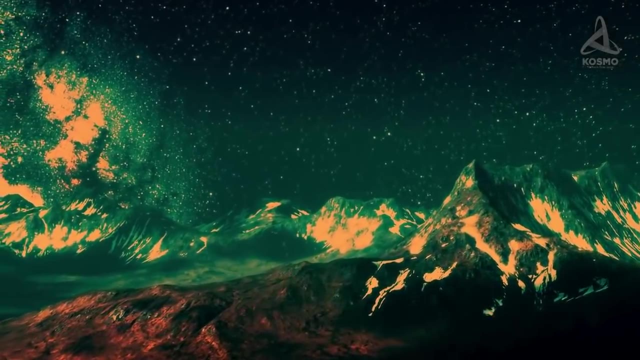 closest approach. The tilt of the rotational axis with respect to the ecliptic plane will not be of such importance as it is in the case of the Earth. The change of season will depend exclusively on the planets getting closer to or away from its parent star. 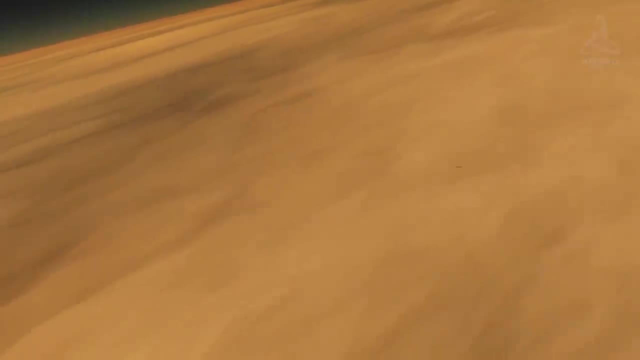 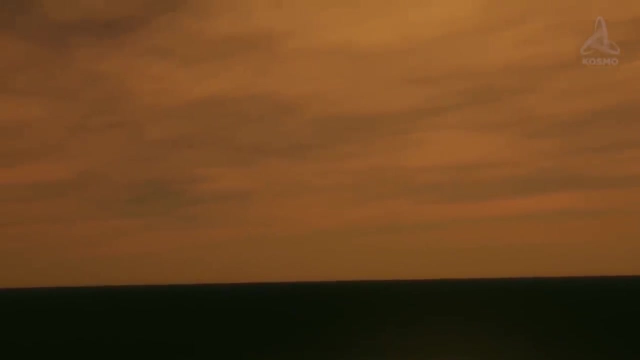 The most favourable conditions for life to develop on Gliese 832c are likely to be in the ring-like area at the border between the light and the dark sides of the planet. It is here that most liquid water will accumulate and rain down from clouds formed on the warm. 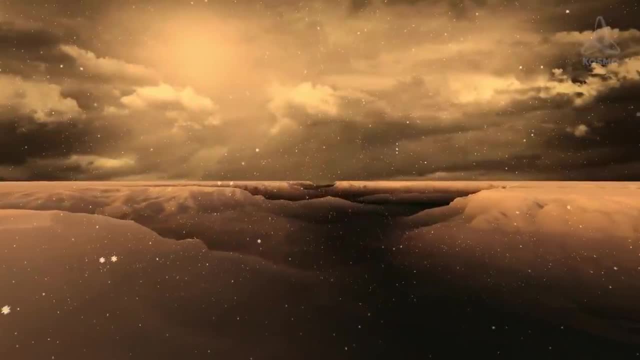 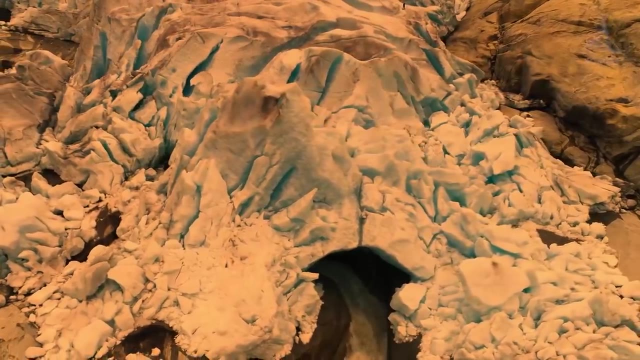 side. Ice caps on the dark side will also melt in the border zone, thus supplying still more water. It goes without saying that it is water that is key to developing life. The change in the temperature on Gliese 832c is likely to be in the ring-like area at the. 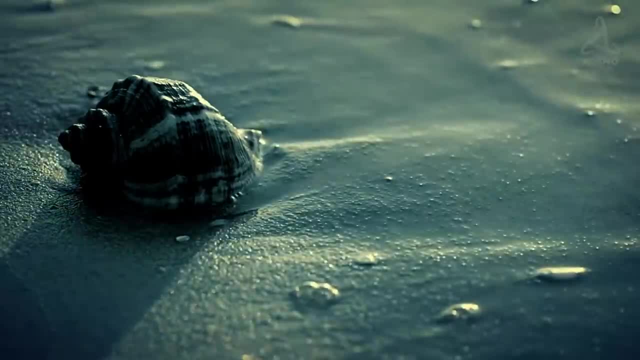 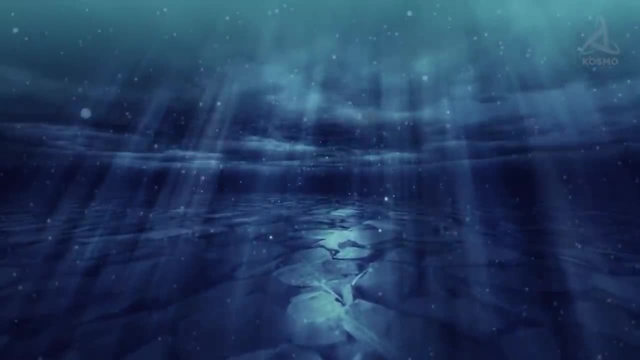 right hand side of the planet. The change of seasons will be likely to play the same role as lunar tides on our Earth, with areas alternately submerging and re-emerging. This process of water getting mixed with substances dissolved in it is a good prerequisite for 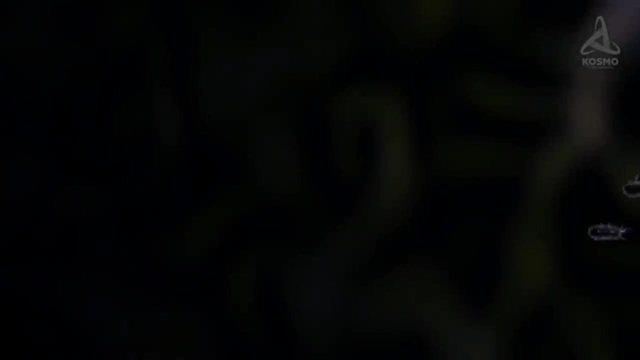 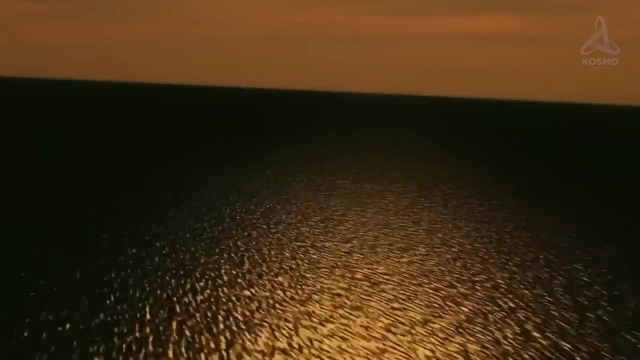 life to originate and develop. There is a good chance of life originating in water and probably staying in it, without later spreading to land. The ocean reduces the effect of gravity and protects its potential inhabitants from sharp temperature changes and hurricanes. The change of seasons will be likely to play the same role as lunar tides on our Earth. 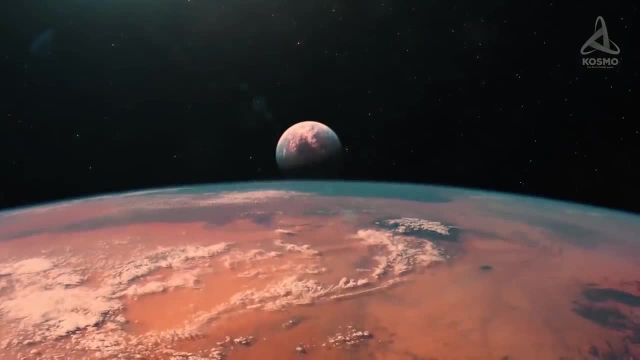 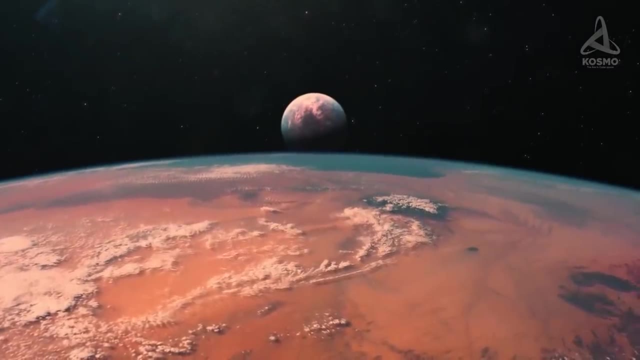 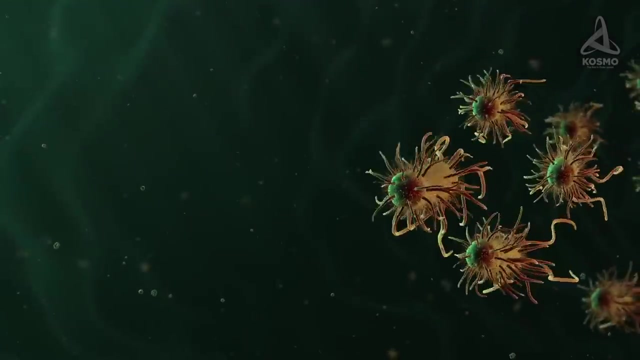 hurricane winds. As for frequent and sharp changes of seasons, hypothetical organisms on Gliese 832c may learn to lapse into a state of anabiosis in order to weather unpleasant, although short, periods of high and low temperatures. Alternatively, they may choose to emigrate to a comfortable temperature zone from the 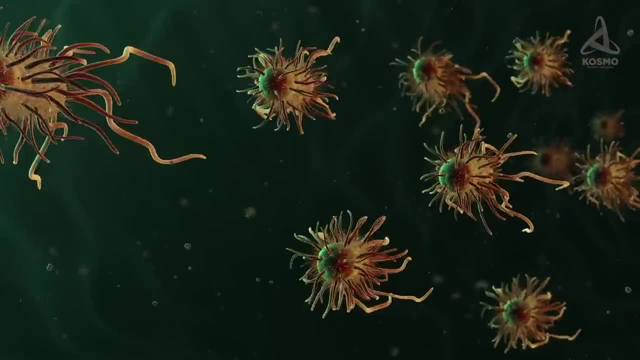 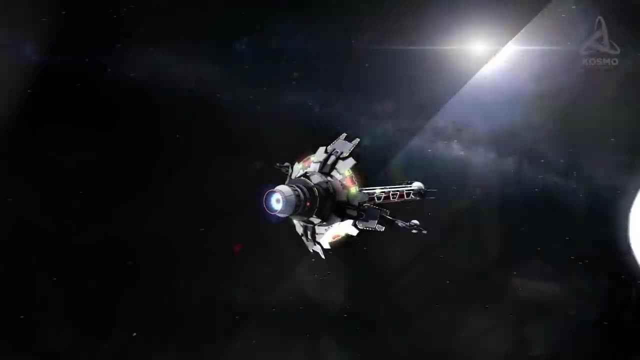 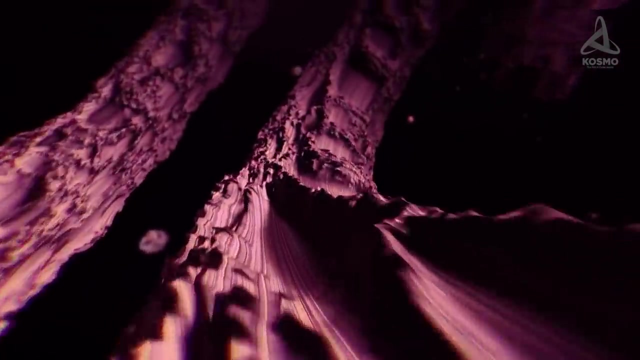 sunny side to the shadow side and back again. for example, If a space probe ever reaches the surface of Gliese 832c to investigate the area, what would it see there, Assuming life did originate on this planet, as the gravity forces are rather strong there? 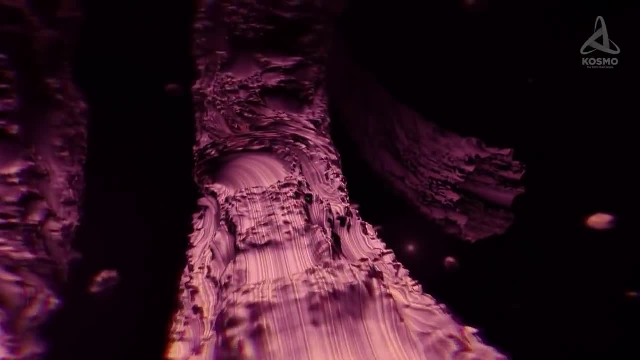 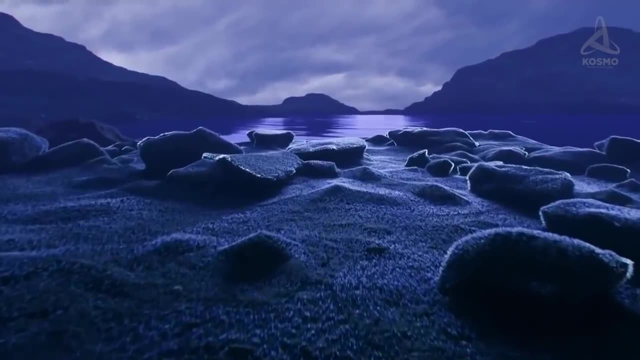 the potential inhabitant should be a thick-set, chunky figure boasting a robust skeleton and powerful muscles. Plants on Gliese 832c would be dark in order to attract as much light as possible. They should also be quite low and likely to fall. 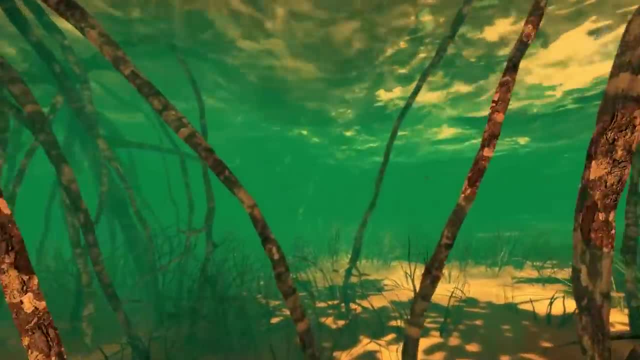 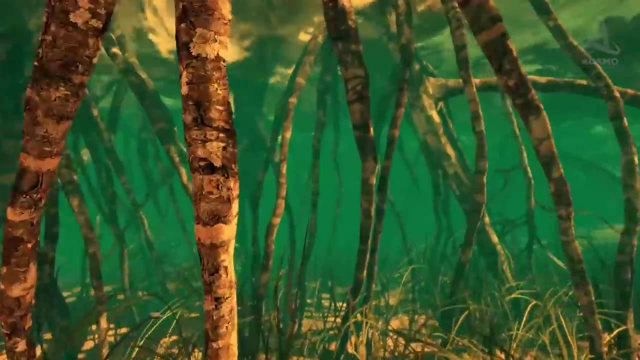 They are likely to be creeping or moss-like, with strong roots able to stand winds. It is highly likely that, rather than chlorophyll, some other molecules should be important for photosynthesis. The planet's dense atmosphere may become a habitat for bizarre life forms floating in. 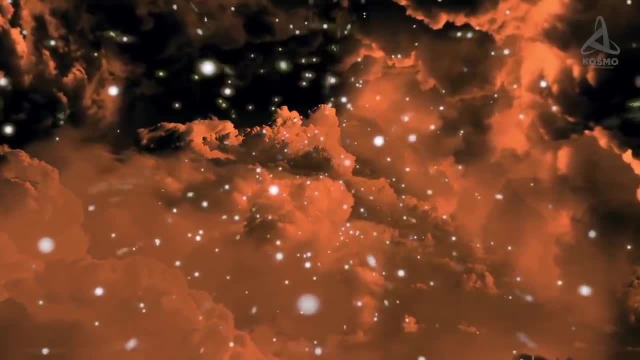 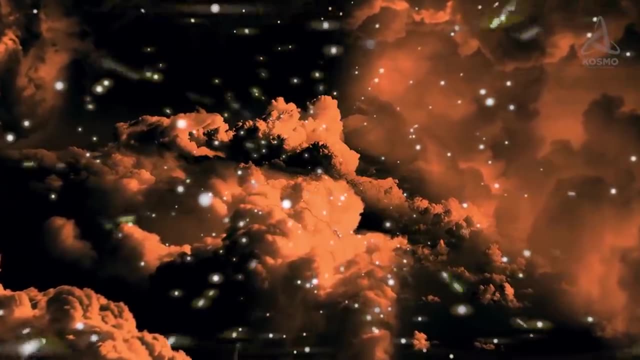 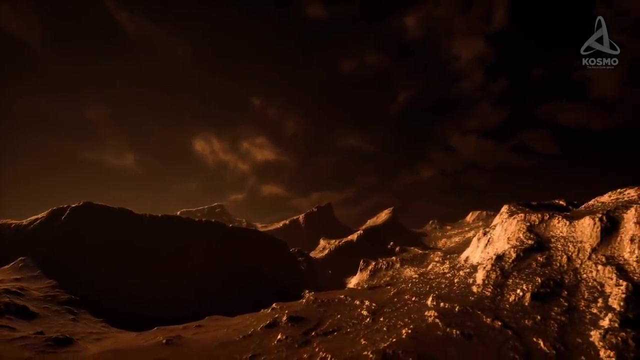 air currents. Single-celled microorganisms, for instance, may float in this dense atmosphere following air currents, while capturing light and nutrients dispersed in the air, Because of a dense atmosphere, they are likely to fall. They are likely to fall High clouds and a dim sun. the surface of Gliese 832c would be a rather dark place. 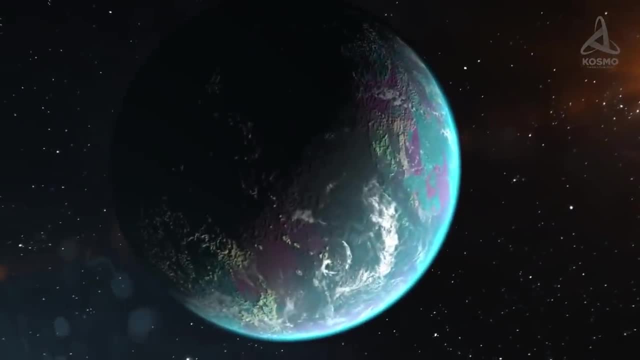 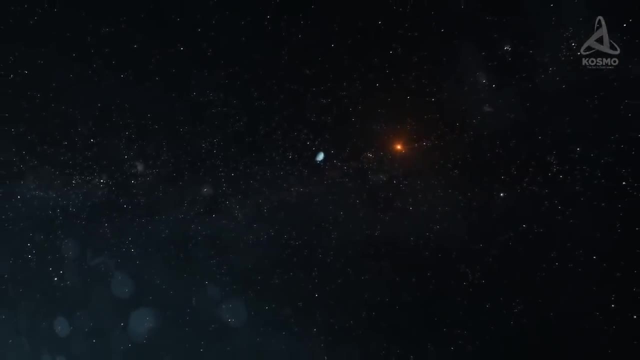 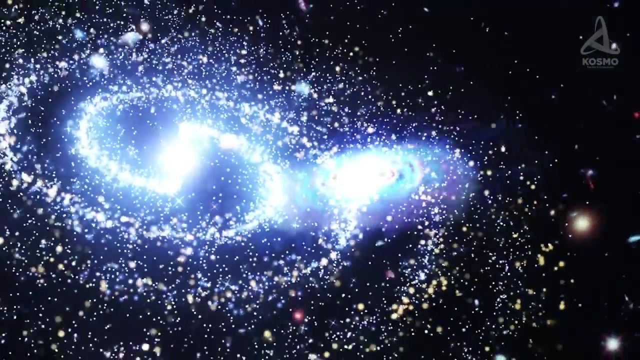 Life forms would have to adapt to these conditions. Vision would probably not play the decisive role in their existence, if it evolved at all. Alternatively, its spectrum may be limited to the infrared range. Be it as it may, all these speculations remain conjectures and ideas, even though they are. 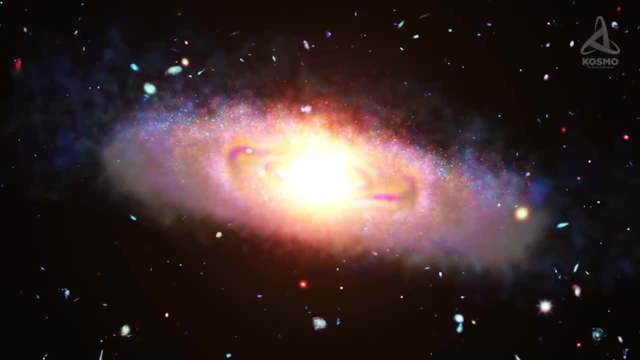 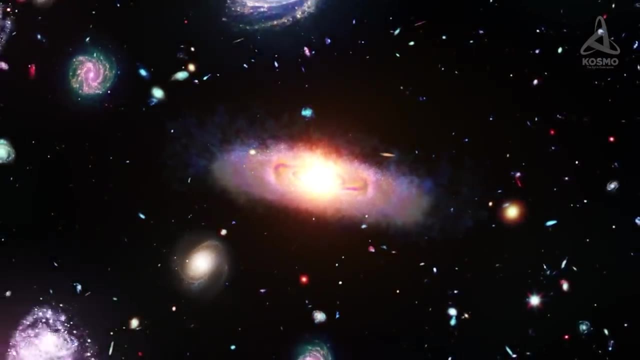 based on good physical laws and assumptions. I wonder Which of these suggestions you would call realistic and which of them bordering on fantasy. Or perhaps Gliese 832c is not habitable at all. Let us know in the comments and let's keep in touch. 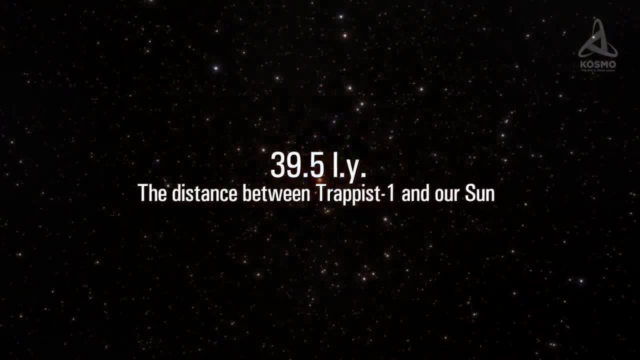 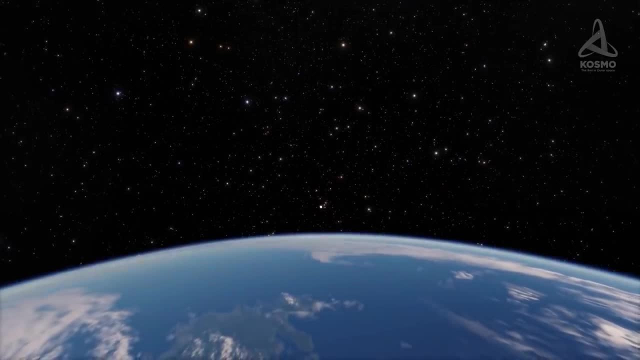 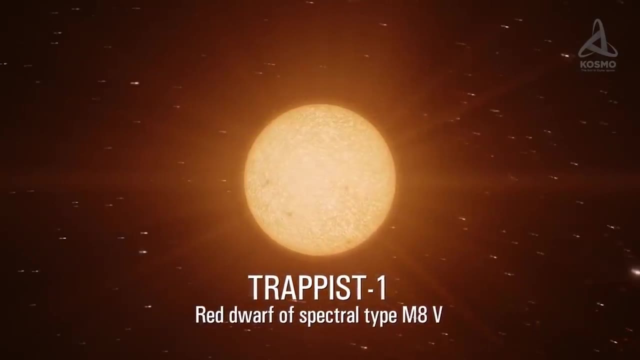 For more detail. the distance between TRAPPIST-1 and our Sun is 39.5 light-years. The object was discovered in the period from 2016 to 2017.. This single star is a red dwarf of spectral type M8V. 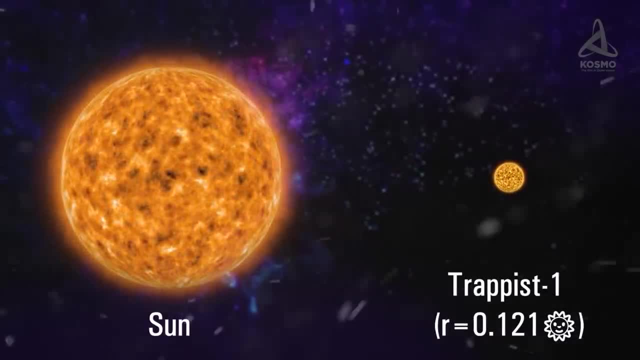 As for its dimensions, it is only 12.1% of our Sun's radius. Just to compare, it isn't, in fact, much larger than Jupiter. The mass of the star is only 12.1% of our Sun's radius. 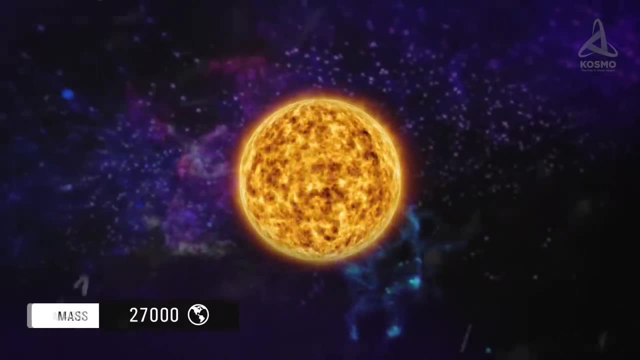 Just to compare, it isn't in fact much larger than Jupiter. Just to compare, it isn't in fact much larger than Jupiter. The mass of TRAPPIST-1 is 27,000 times that of our Earth, but at the same time is 0.08. 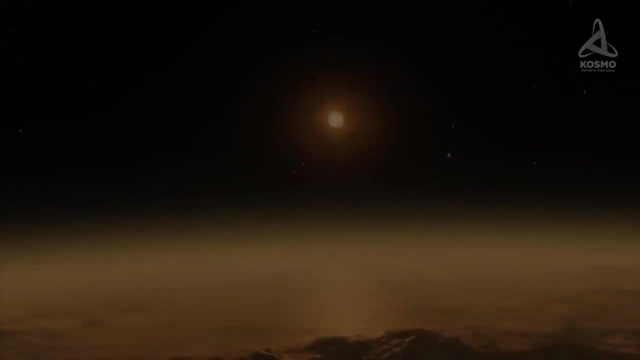 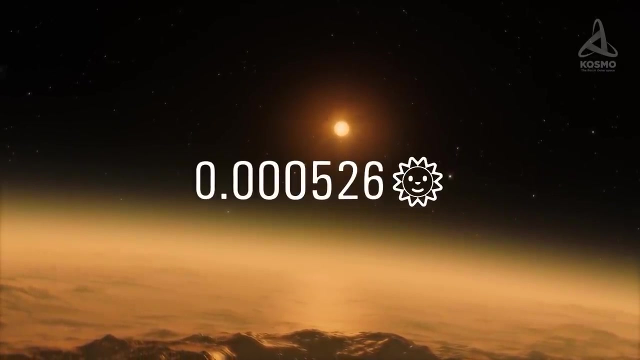 the mass of our Sun, With the average temperature reaching 2500K. its luminosity is 1900 times weaker in comparison with that of the main star of our system. The orbital period of TRAPPIST-1 is 3.3 days. 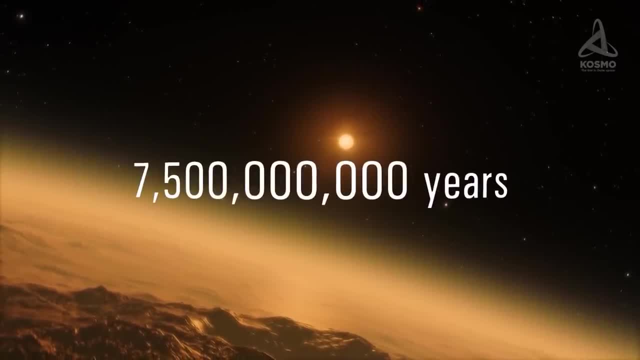 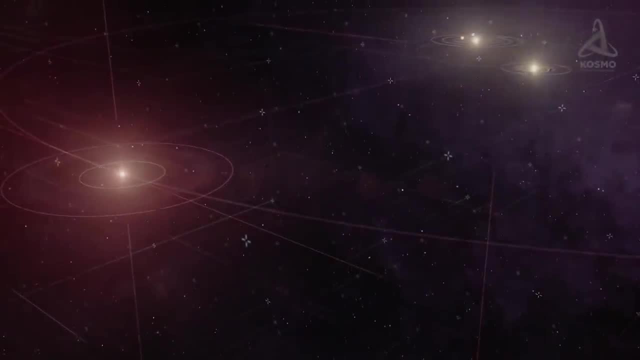 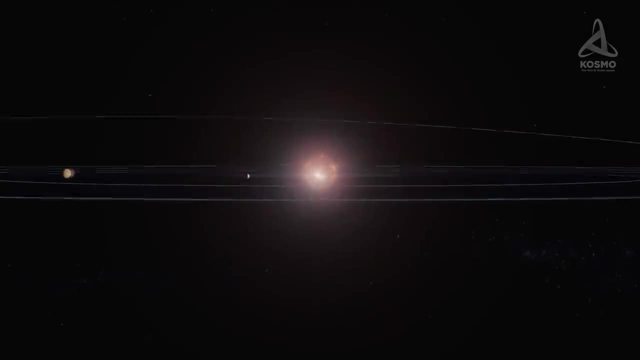 As for its age, it is 7.5 billion years, which makes it almost 3 billion years older than the Sun. The distance between this star and us is diminishing, as it is slowly but surely drifting towards our system. This object aroused interest largely following the discovery of its planetary system back. 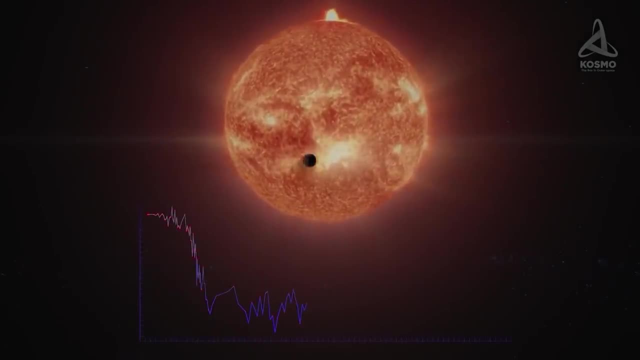 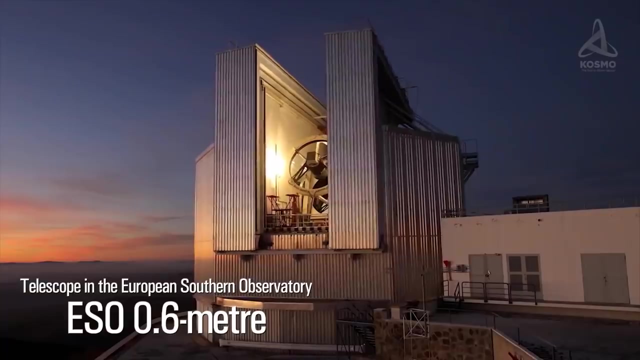 in 2016,, whose three components were spotted by a transit method with the help of an automated 0.6-metre telescope in the European Southern Observatory or the ESO in Chile. The planets were initially seen in the solar system, but they were not seen in the solar 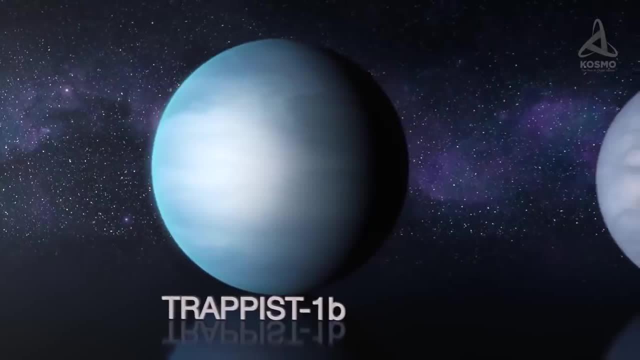 system. The planets were initially seen in the solar system, but they were not seen in the solar system. Now the earth has three planets and they are called TRAPPIST-1B, TRAPPIST-1C and TRAPPIST-1D. 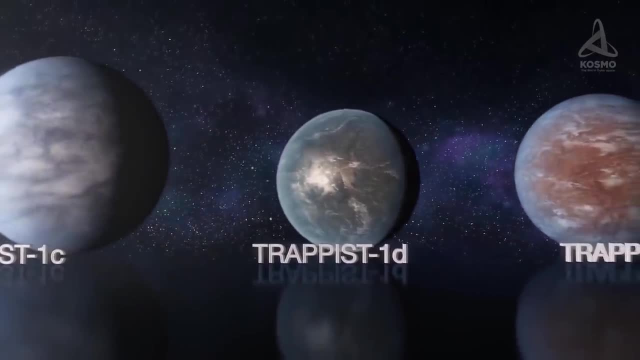 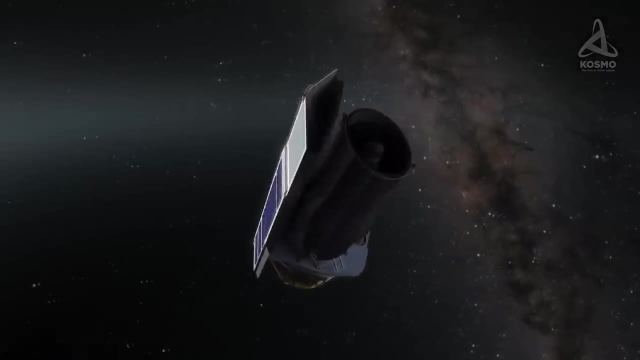 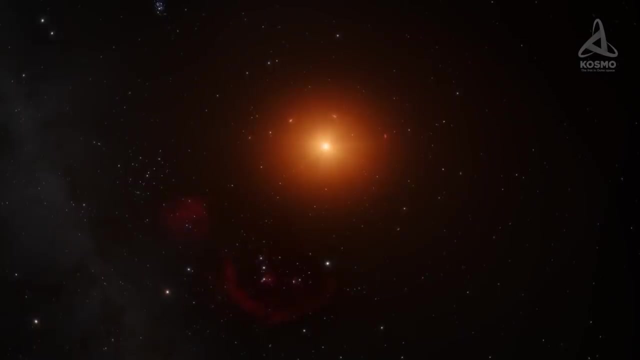 However, further investigations revealed that the presumed location of TRAPPIST-1D was described incorrectly, Following that, four more earth-like objects were discovered by astronomers with the help of the Spitzer Space Telescope. These were dubbed TRAPPIST-E, F, G and H. 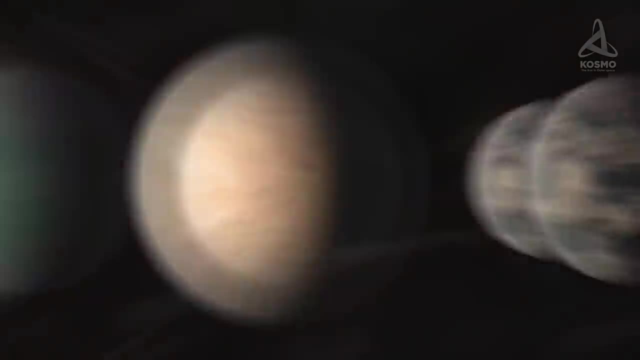 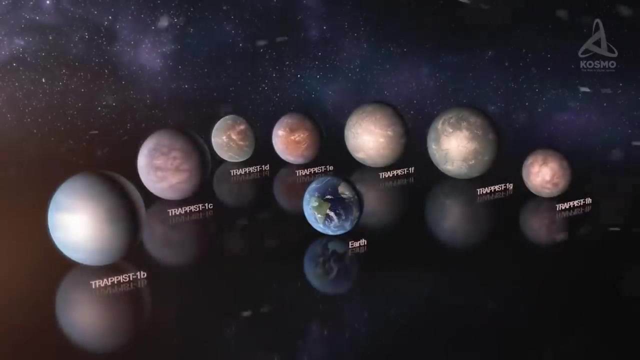 Thus, the total number of planets in the system reached seven and on the 13th of April 2016, seen, the parameters of these celestial objects were defined in more detail. All the seven exoplanets are identical to our Earth in terms of their dimensions, with. 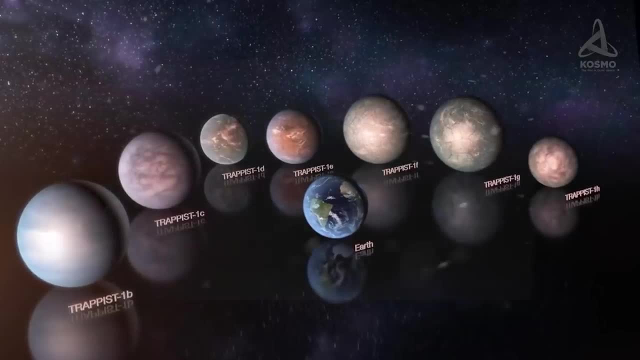 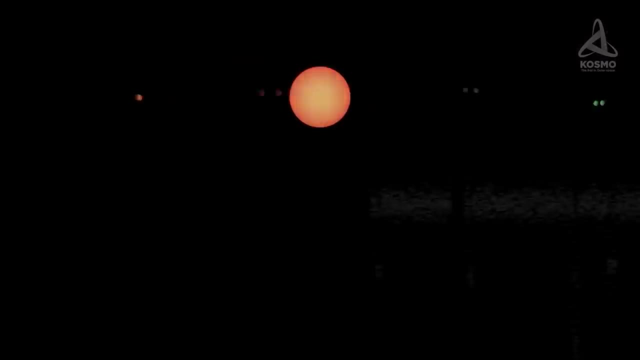 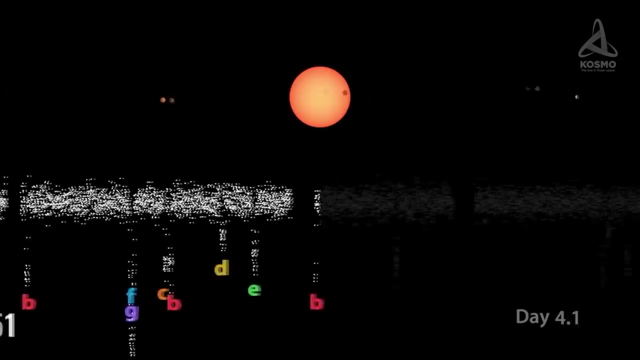 their radii ranging from 0.71 to 1.13 that of our planet. Planets B and C orbit their parent star in the periods of 1.51 and 2.42 days respectively. Initially, according to astrophysicists, both of these planets were comparable to Venus. 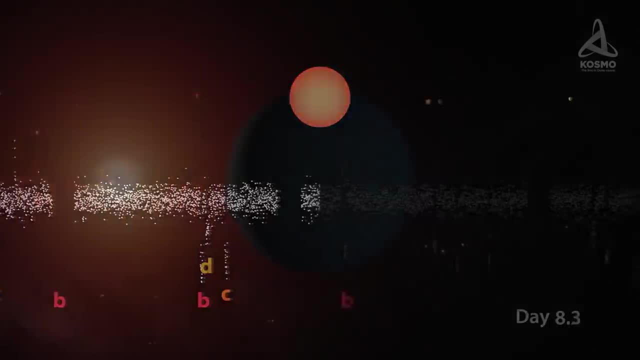 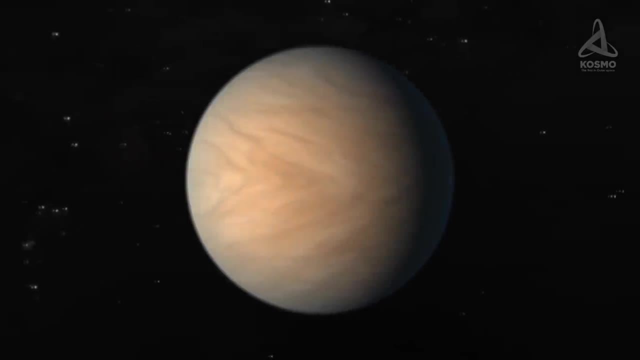 in all but exceptionally high temperatures. However, after their mass and density had been measured, it was TRAPPIST-1 that could be called Venus' analogue. TRAPPIST-1b, the second closest planet to its star, is likely to contain a large amount. 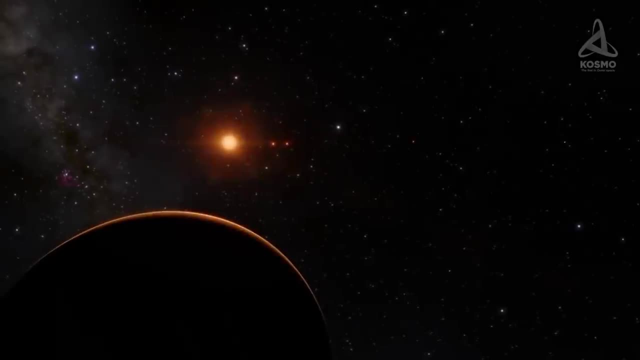 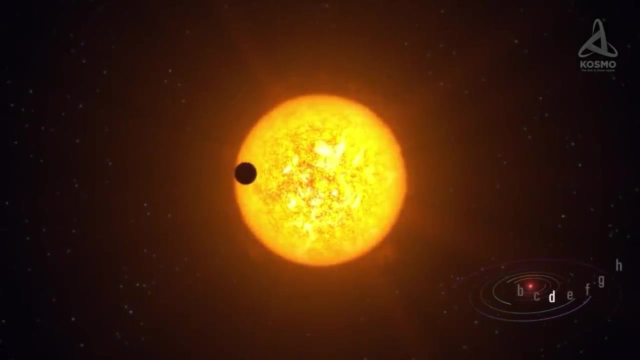 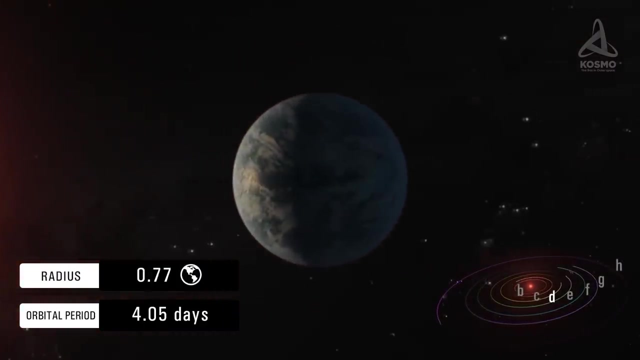 of water and other volatile elements. The new data enabled scientists to find out more about the other discovered planets too. It takes TRAPPIST-1d 4.05 days to orbit its star. Its radius is 0.77 that of the Earth. 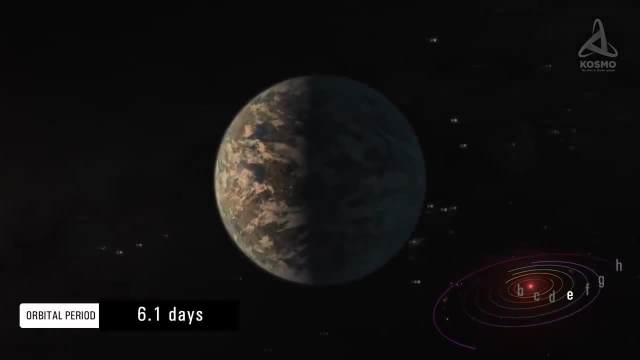 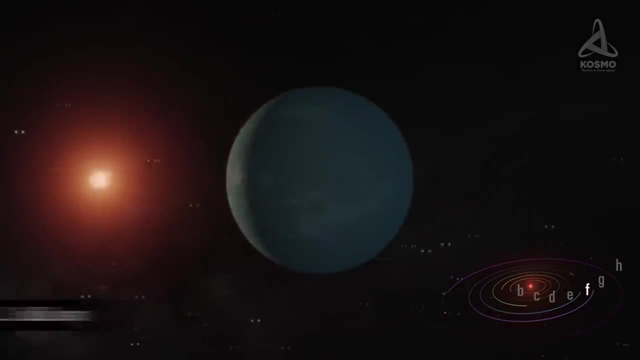 The orbital period of TRAPPIST-1e is 6.1 days. Its radius is 0.92 that of the Earth. The orbital period of TRAPPIST-1f may last up to 9.2 Earth days. 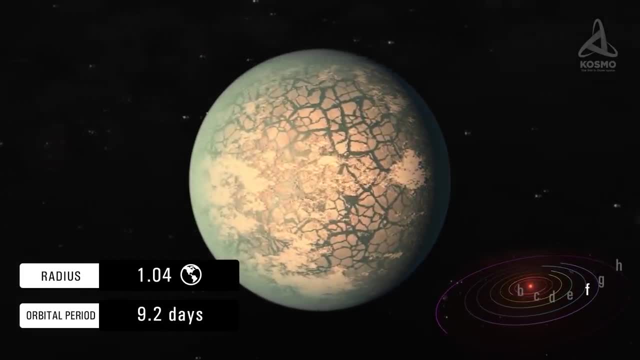 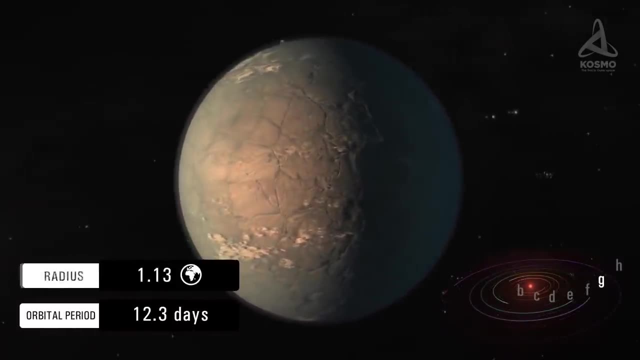 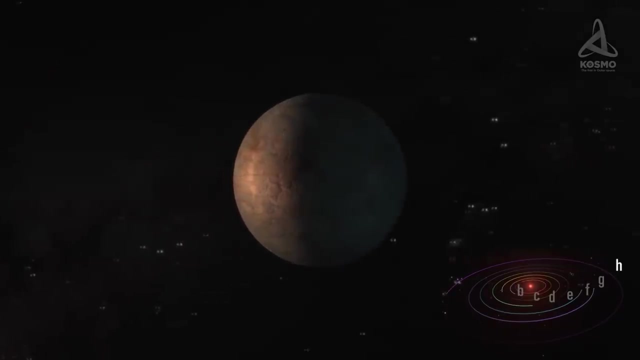 Its radius is 1.04 that of the Earth. The orbital period of TRAPPIST-1g is 12.3 days and its radius is 1.13 that of the Earth. Last but not least, TRAPPIST-1h is the seventh object and is the furthest from its star, with 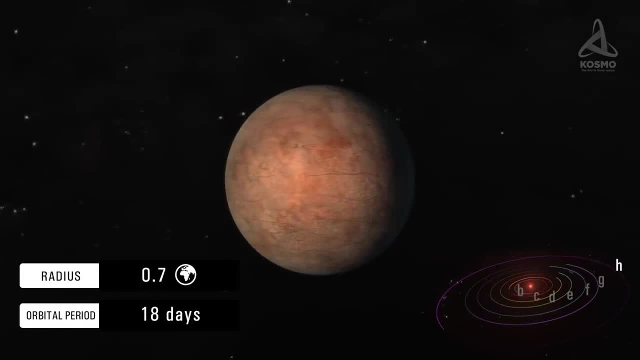 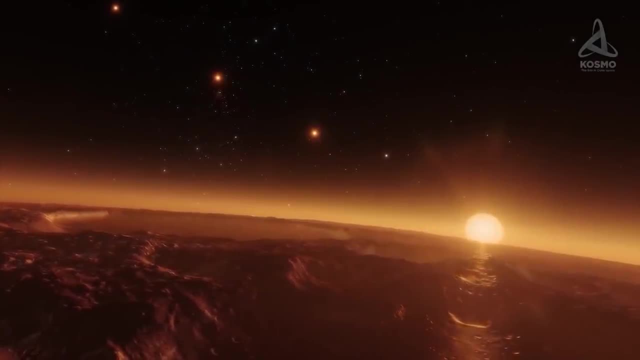 a rotation period of 18 days and a radius of 0.7 that of our planet. It should be mentioned that the initial estimates of the object's masses were likely to be rather conservative, Due to the analysis of the density of the first six planets. it was later ascertained. 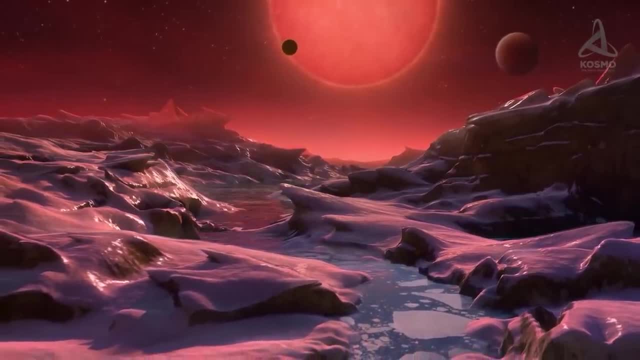 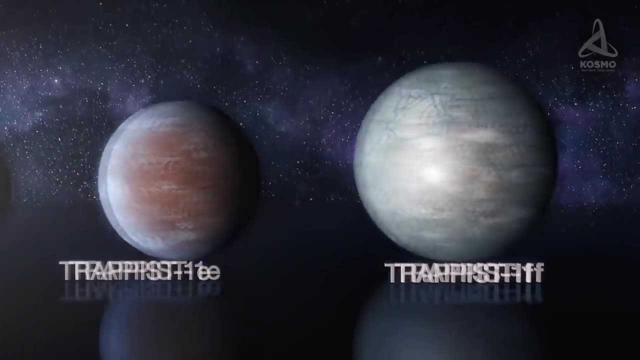 that they contain a big amount of water and other volatile elements, which makes them considerably lighter than thought previously. As for the furthest of them- E, F, G and H- for all we know they may consist entirely of water. 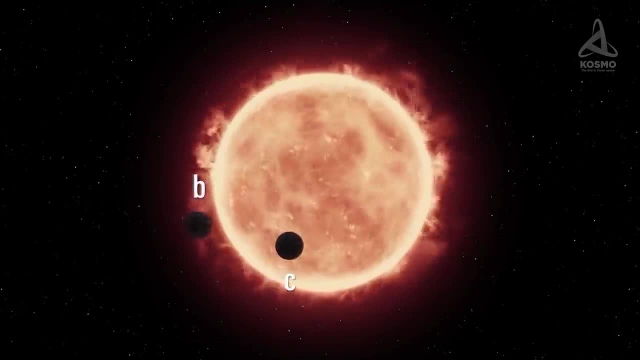 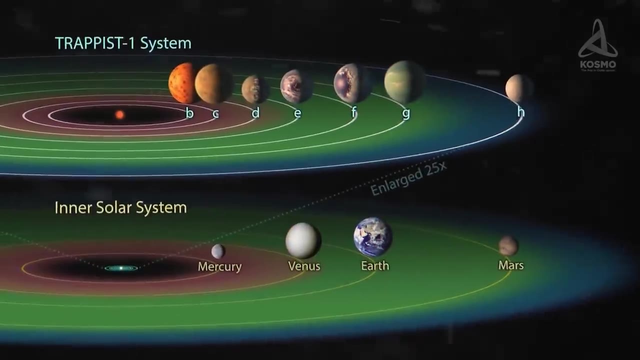 Only TRAPPIST-1c boasts a mass bigger than initially estimated, which may be indicative of over 50% of iron in its composition. Of the seven planets known to be located in the TRAPPIST-1 system, three of them find: 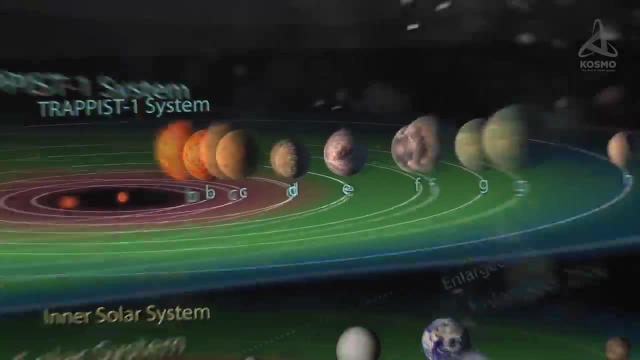 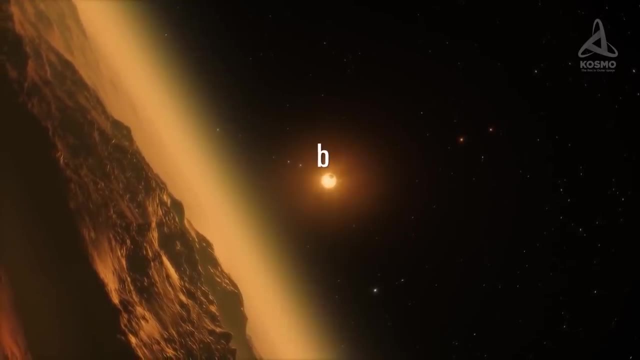 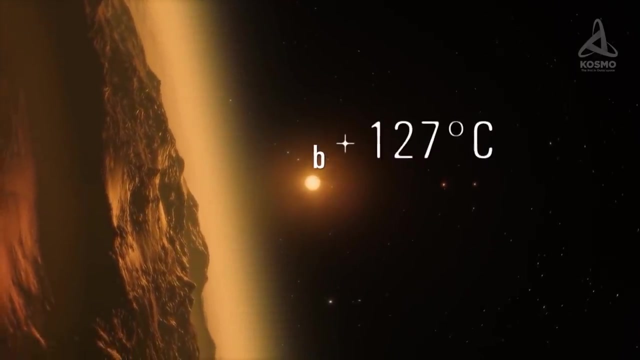 themselves within the habitable zone, namely D, E and F. Speaking about the rest of them, following the estimates of its density, planet B is thought to contain either a small nucleus or else a considerable amount of volatile elements Due to high temperatures of 127.69°C above zero on the surfaces of planets B and C respectively. 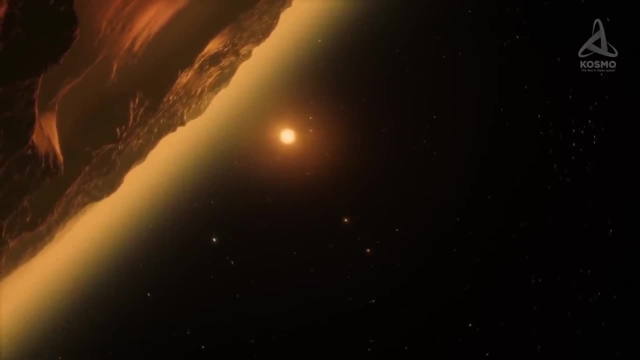 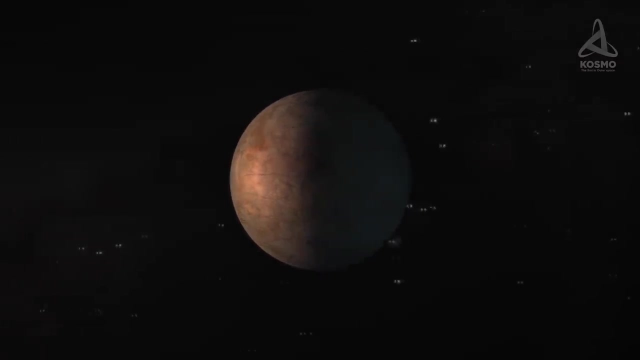 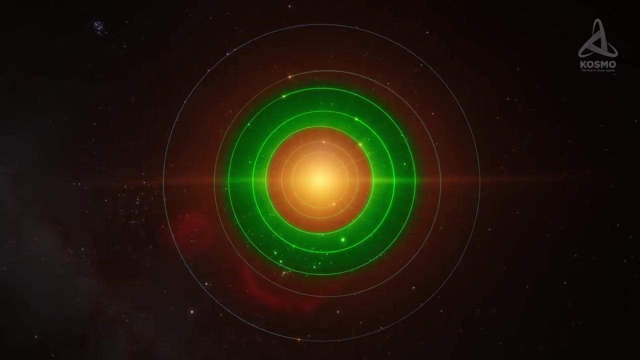 water is not likely to remain in its liquid state there and is bound to float about as vapor. As for planets G and H, they are too remote from their central star to be potentially habitable. However, according to models suggested at Cornell University, the habitable zone of 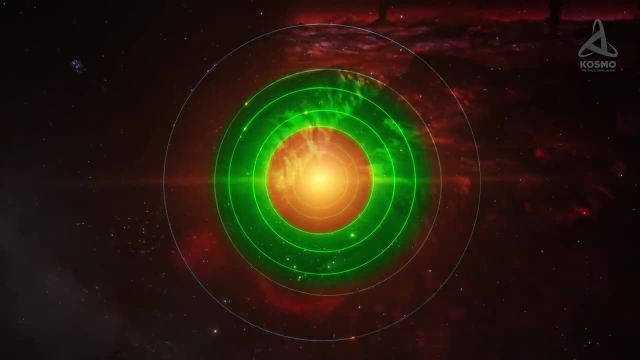 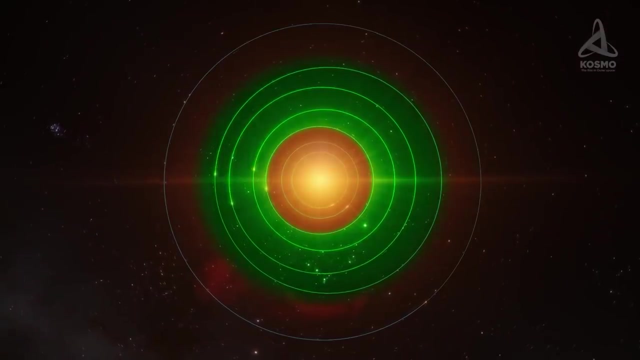 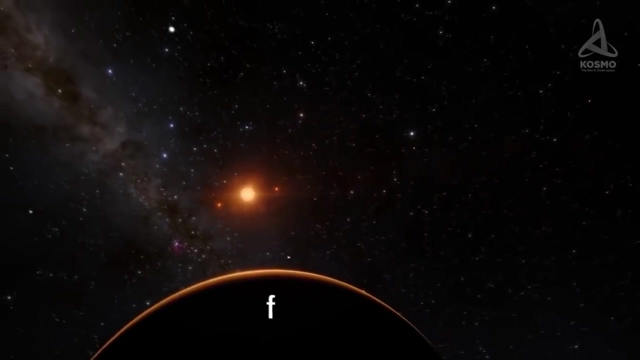 TRAPPIST-1 may well be wider and, allowing for volcanic hydrogen potentially acting as a greenhouse gas, there may be four planets within the habitable zone rather than three. The density of TRAPPIST-1f is rather low too, and so it may well turn out to be an all-ocean. 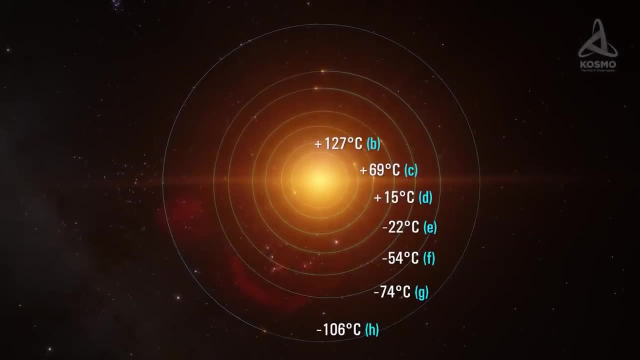 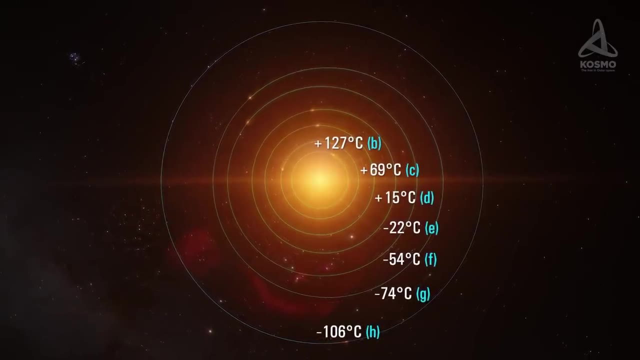 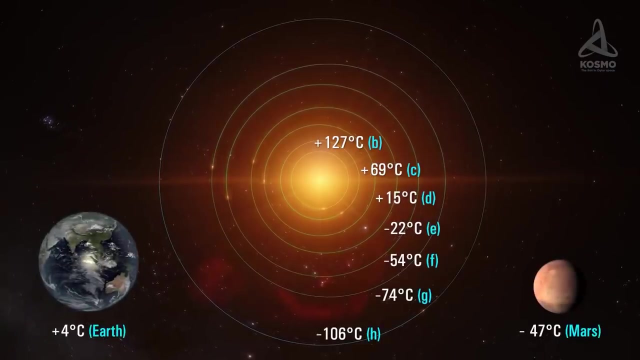 planet. Here are the temperatures for all the planets in the system. The steady state temperatures are given without including incident light dispersion and greenhouse effects. Just to compare, the steady state temperature on our planet in the same conditions would measure 4 degrees above zero and on Mars 47 degrees below zero. 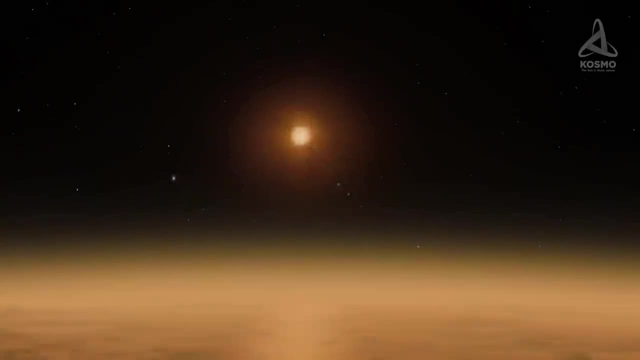 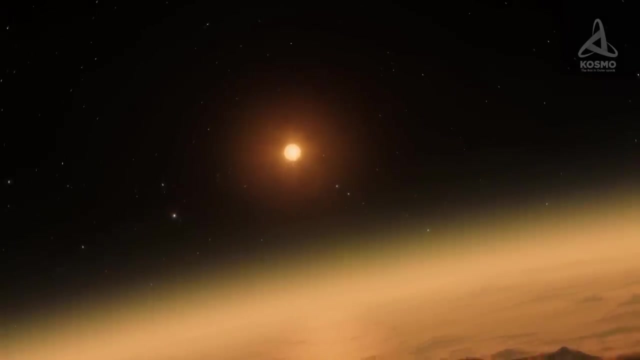 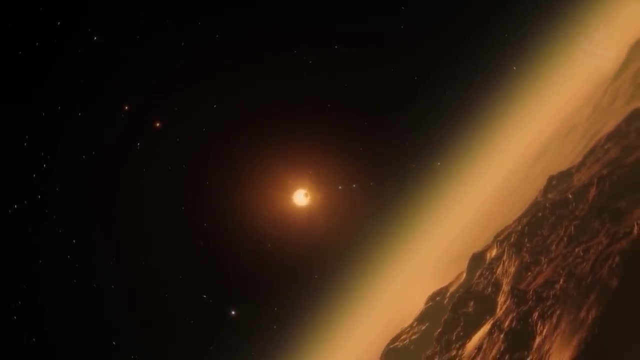 In November 2017, it was posited that the activity of this star didn't allow its planets to form and maintain their own atmosphere. It is accounted for by the fact that TRAPPIST-1 goes through periods of active flares which may negatively affect the nearby celestial bodies and thus render them uninhabitable for living organisms as we know them. Interestingly, the planets are located much closer to each other in comparison to our system's planets. The planet Mercury, which is the closest one to the Sun, is located 0.39 astronomical units from it, while the distance between TRAPPIST-1b and its parent star is just 0.01 astronomical units. 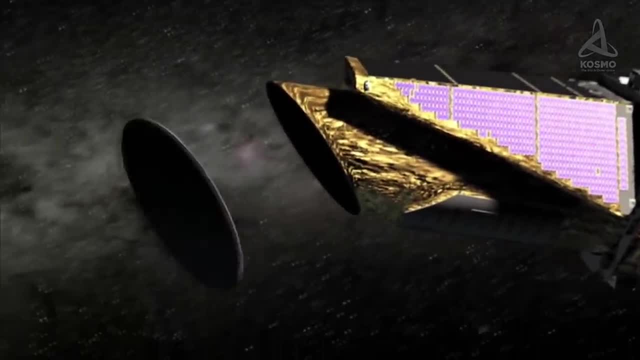 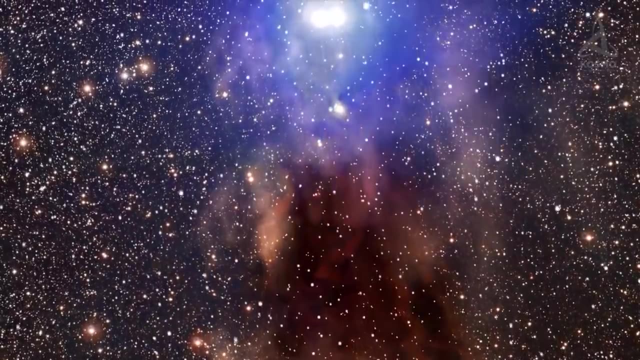 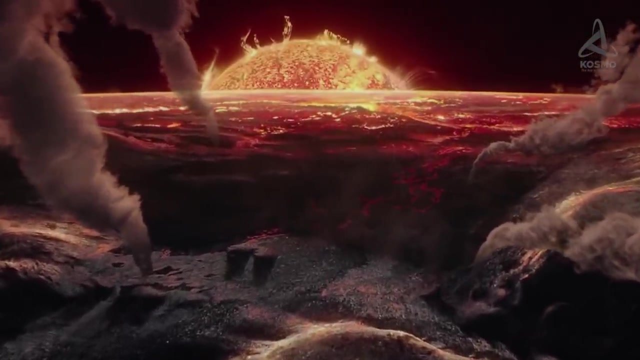 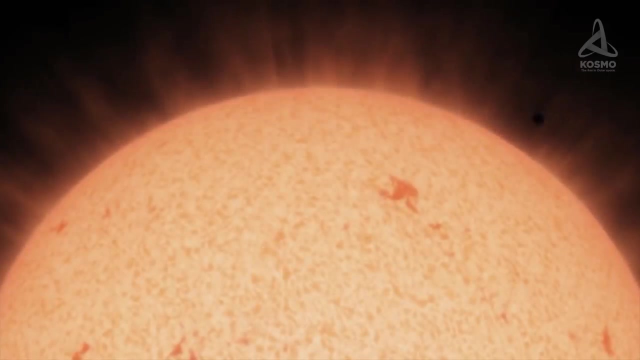 As TRAPPIST-1 is a rather dim star, it is no easy matter to explore it. Red dwarfs like that are quite widespread across the Universe, accounting for most of the galaxy's stellar matter. Plasma ejections on these stars are a rare occasion, although astronomers believe that there may be giant cold areas and compact hot areas with temperatures upwards of 4000 K on the surface of TRAPPIST-1. 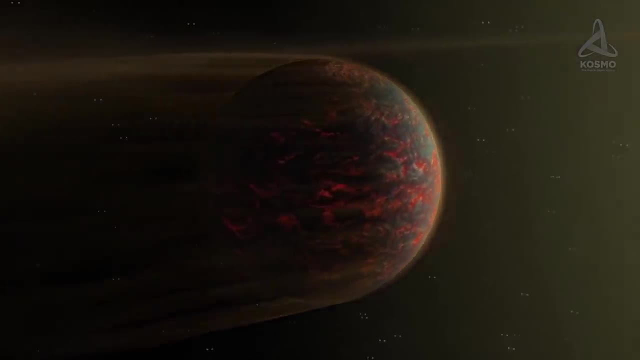 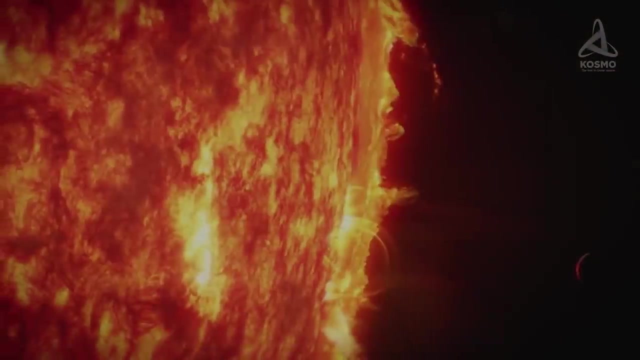 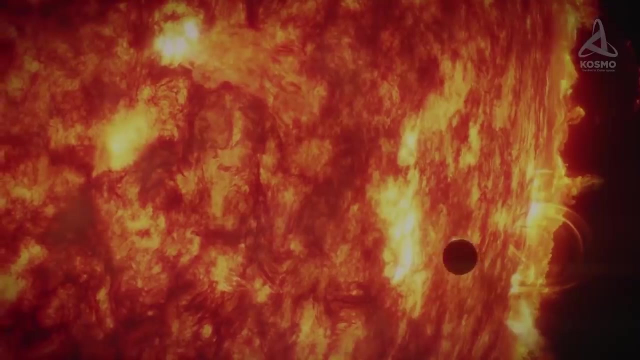 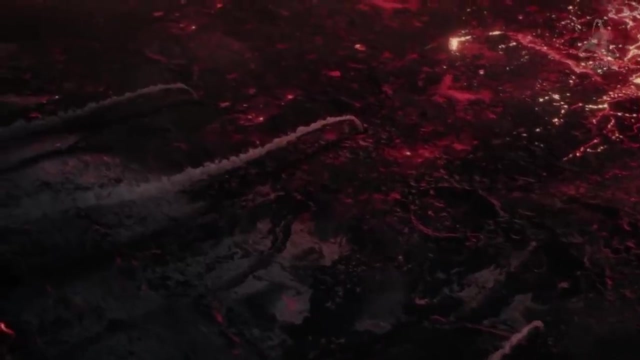 If this conjecture proves to be true, scientists will proceed to confirm that the system's planets are constantly bombarded by powerful ultraviolet and X-ray radiation, which is able to destroy their atmospheres and render their surface completely sterile. The reason for that lies in the fact that none of the microorganisms known on the Earth are able to withstand intensive radiation emanating from flares of this kind, including the most radiation-resistant bacteria, Deinococcus radiodurans. 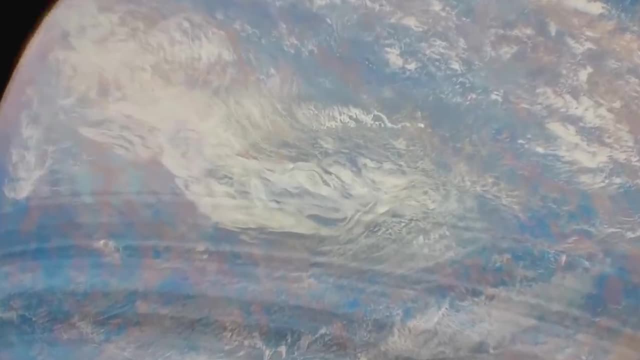 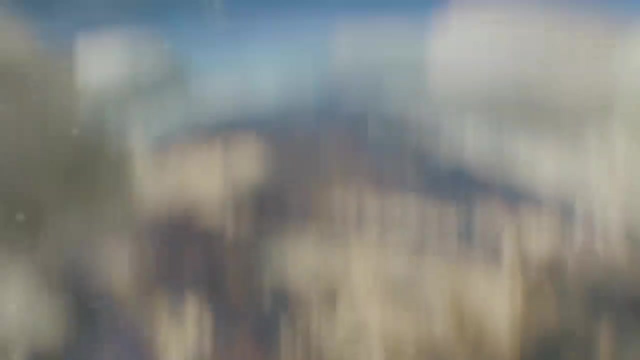 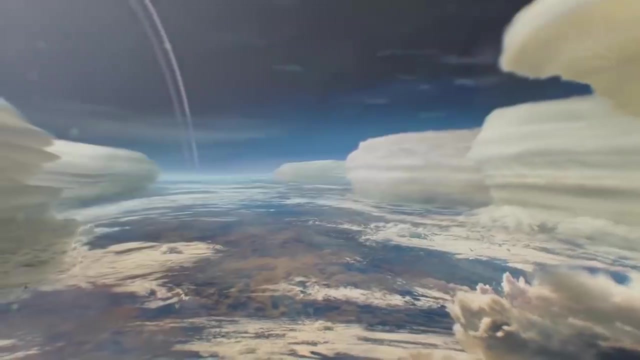 Nevertheless, in December 2017, atmosphere was proven to persist even in periods of high activity of stars, which implies that planets G and H may potentially have their own atmospheres. At the moment, astrophysicists' idea is to use more up-to-date telescopes for studying the matter. 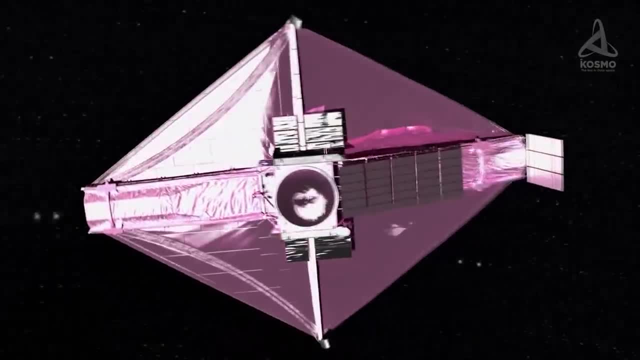 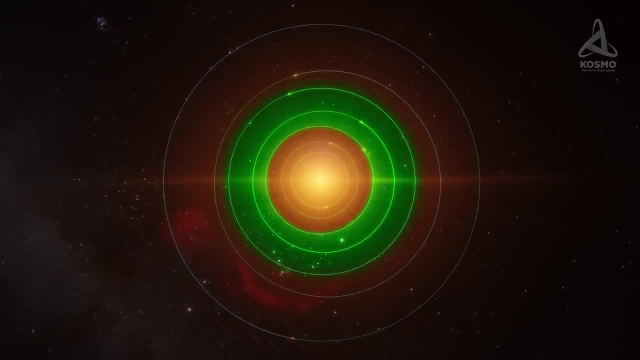 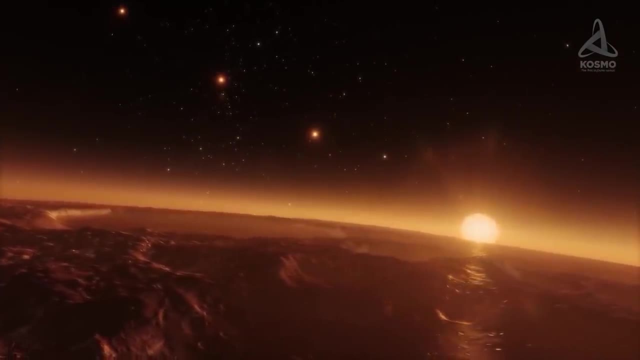 For example, the James Webb Space Telescope, whose launch is planned for March 2021.. Today, the TRAPPIST system presents a great interest for the global scientific community, And, even though it is highly unlikely that any advanced civilization will be discovered on its planets, we cannot ignore the fact that life forms in the Universe may be extremely diverse. 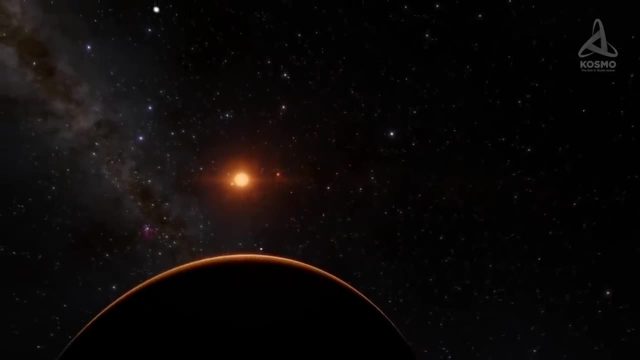 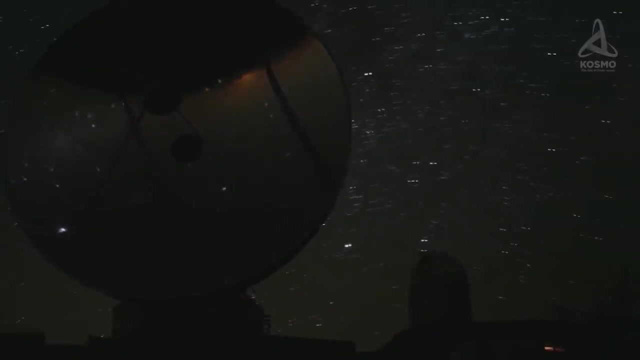 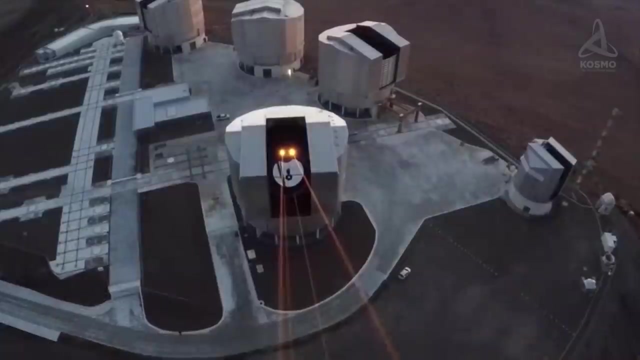 and may differ from our perceptions of life as we know it, which implies that not all intelligent organisms are supposed to follow the scenario of our planet. If science manages to find out more details about this system in the nearest decades, many conjectures and doubts we have today about TRAPPIST-1 will most likely be cleared. 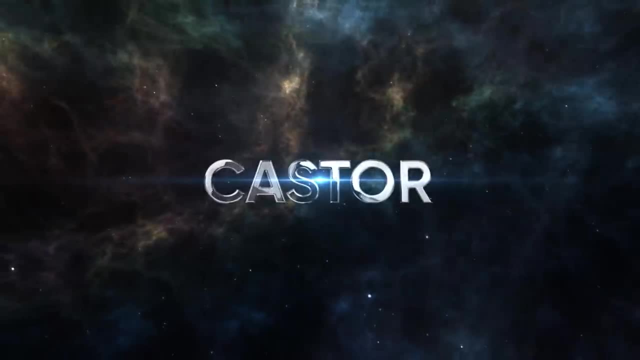 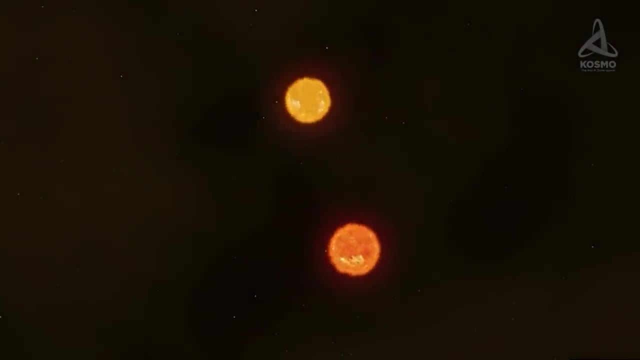 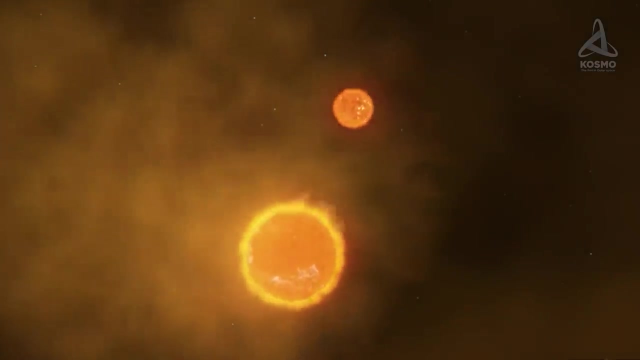 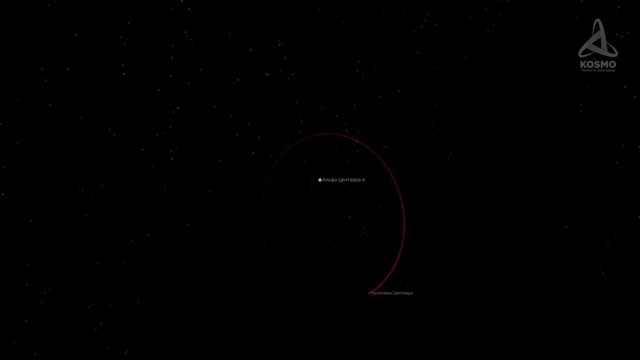 Systems with this number of stars are rather rare. What we see while observing the stars are generally binary systems, that is, systems consisting of two objects. As for multiple systems, that is, those made up of three or more stars, they are by far rarer. 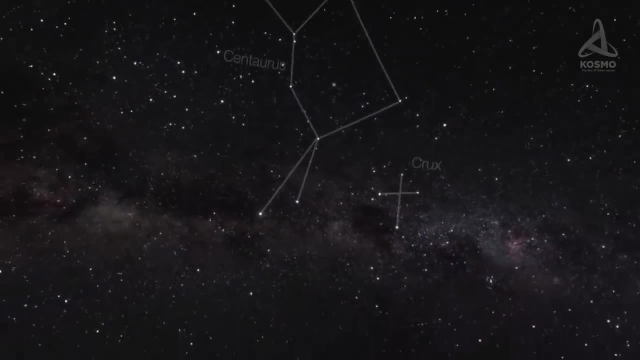 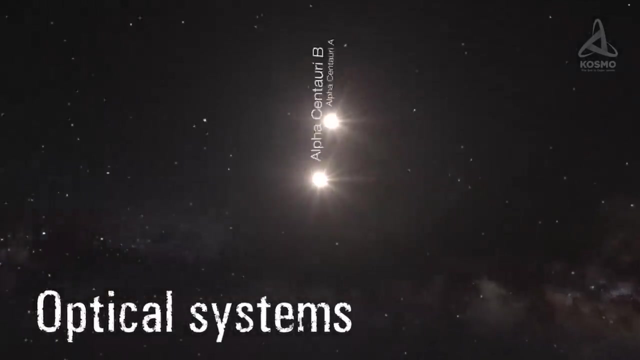 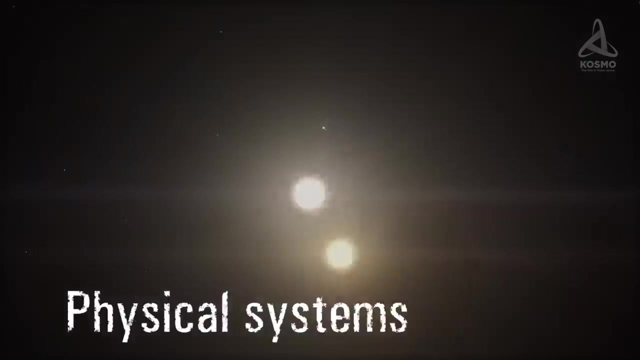 There are two varieties of multiple systems, namely optical and physical Objects, and optical systems are located far from each other, While seen from the Earth they appear to be just one star. Objects and physical systems, meanwhile, are actually close together and are bound by gravity. 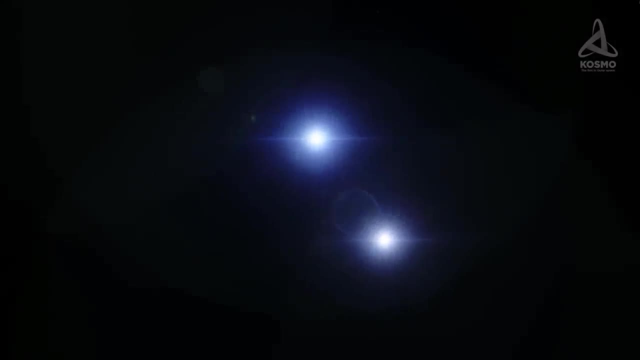 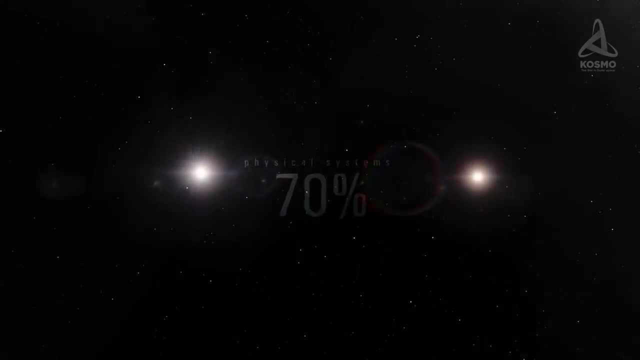 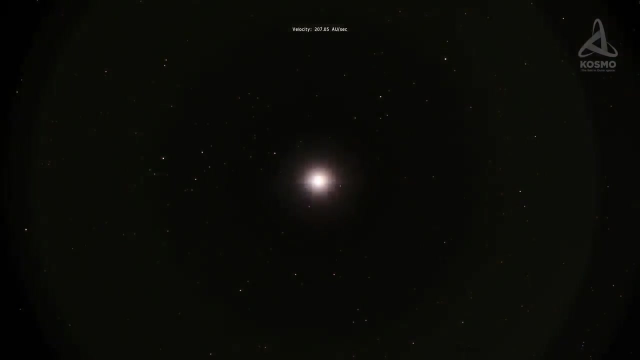 Most physical multiple systems consist of just three objects. It is triple systems that account for about 70% of all systems of this kind known to us today. The Castor system, however, is noticeably different from the majority. Each of the three main stars in this system is a binary star. 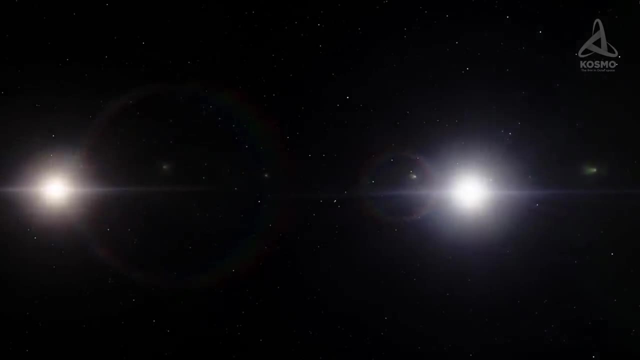 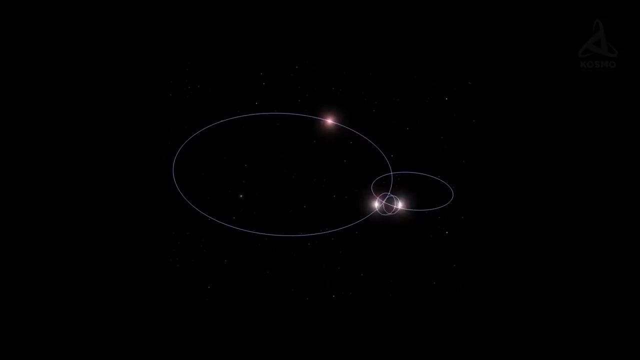 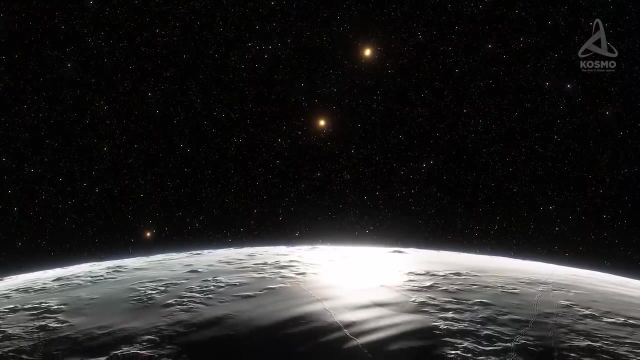 Thus, the total number of stars in Castor is six. It is also highly unlikely that there are stars in areas unobservable to us in Castor's vicinity which are gravitationally bound to this sextuple system. The more components a multiple system contains, the fewer such systems there are in space. 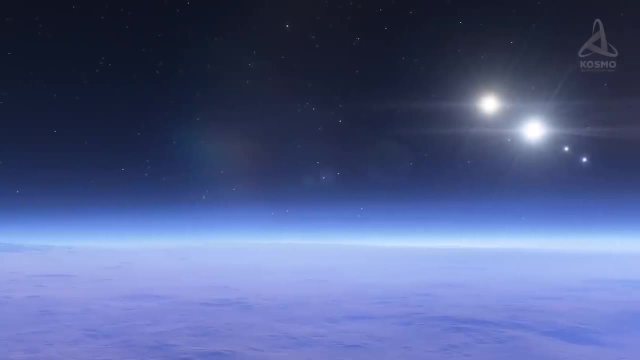 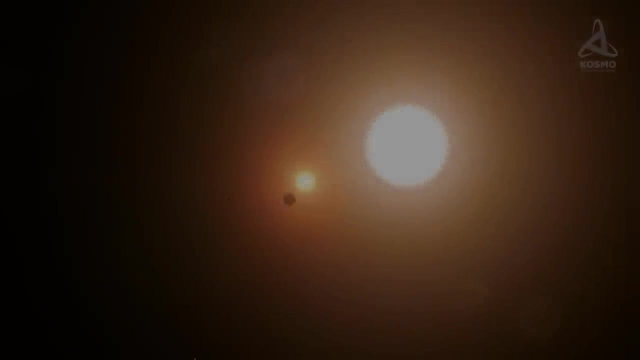 This means that systems consisting of three and more stars must be extremely rare in the Universe. It goes without saying that we are far from possessing all data about multiple systems. That is why we can't but admit that, in theory, there may be systems with still more components somewhere in deep space. 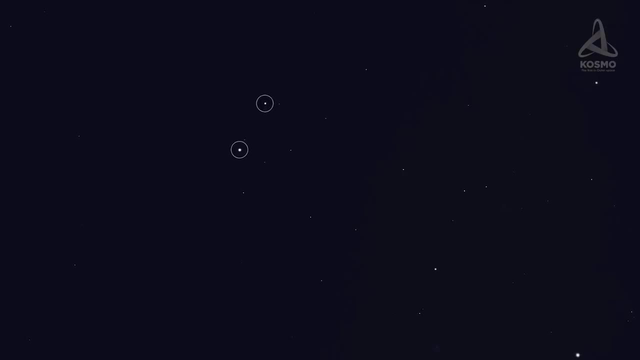 Getting back to the Castor system, this is the second brightest object in the constellation Gemini. It is beaten only by Pollux, an orange-hued giant star. In terms of luminosity in our sky, Castor holds the 23rd place. 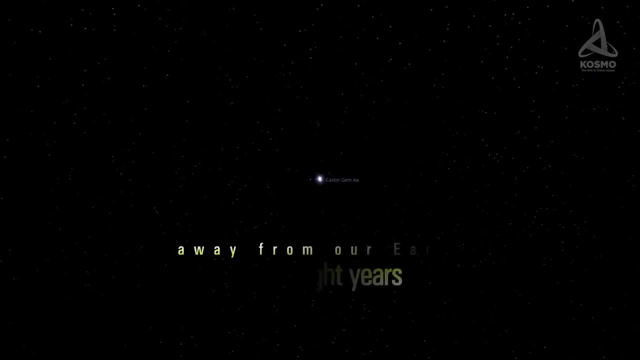 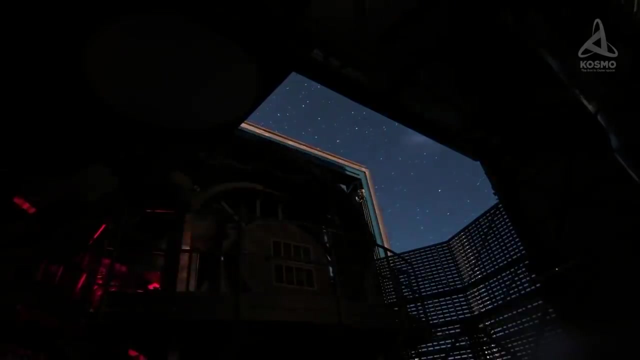 The system is 50.88 light-years away from our Earth and its age is estimated at approximately 200 million years. It was discovered back in the 17th century and even then it was classified as a binary system, And later astronomers managed to spot several other objects physically bound to it. 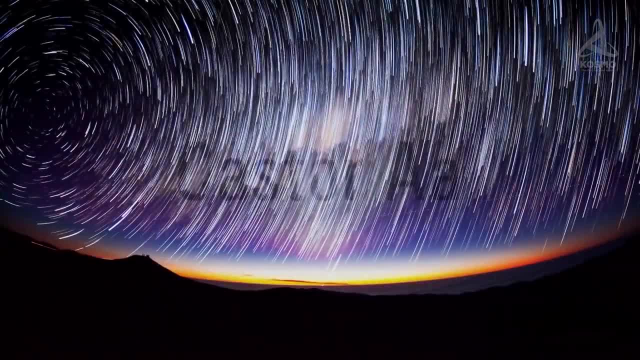 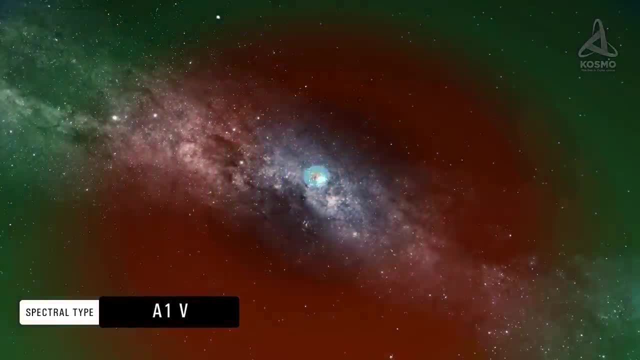 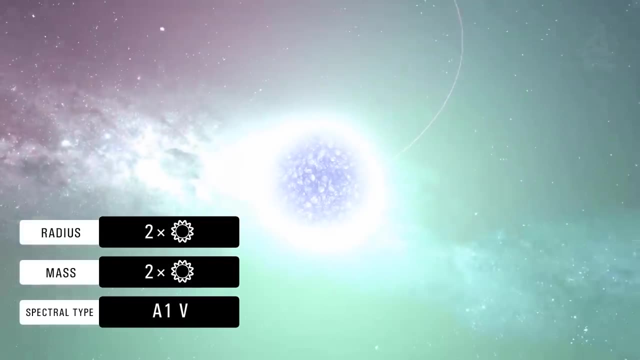 The first and the main component of the system was dubbed Castor AA. This is a main-sequence star of spectral type A15.. It is about twice as heavy as our Sun and its radius is also two Sun's radii. The surface temperature on Castor reaches approximately 9,140 degrees Kelvin. 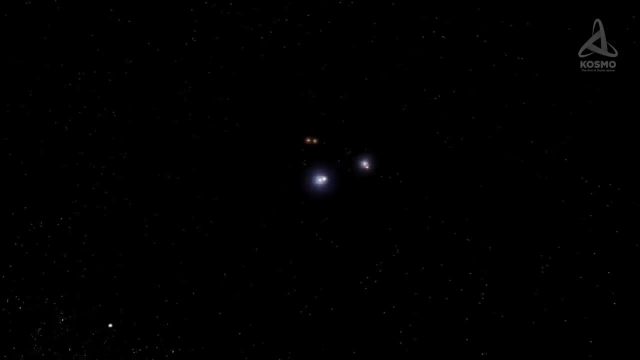 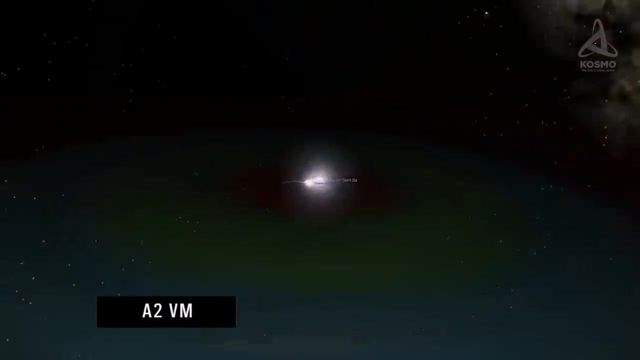 At the same time, the object's luminosity is 30 times that of our Sun. The second component's designation is Castor BA. It is of spectral type A25M and its mass is 1.7 times that of the Sun. 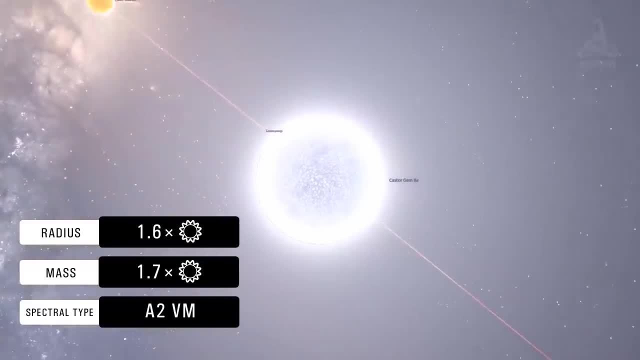 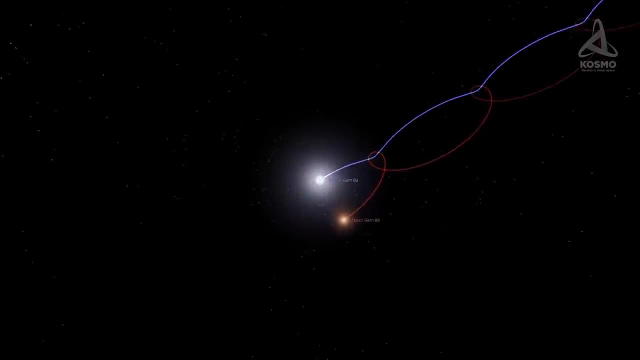 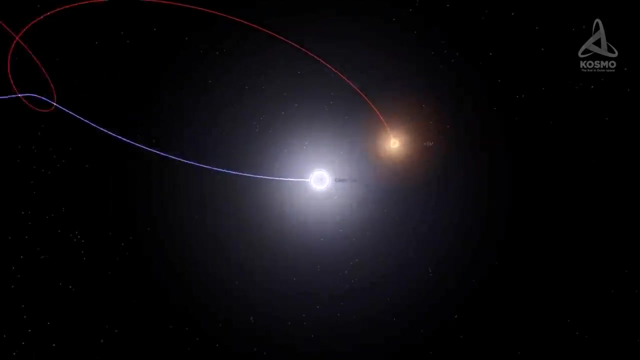 and its radius, measuring 1.6 that of the Sun. Castor BA orbits its companion star, Castor AA. It takes the two objects about 350 years to complete a full orbit around each other. It was later found that the eclipsing variable star YY Geminorum is also physically bound to Castor. 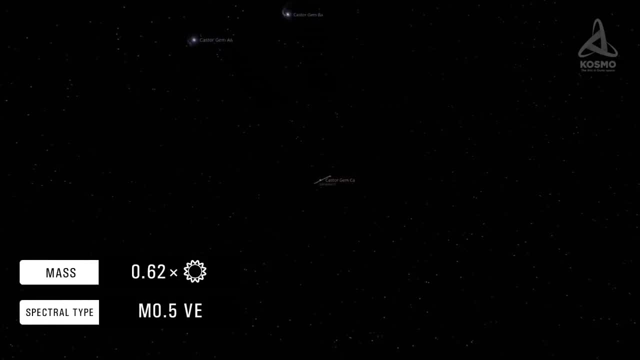 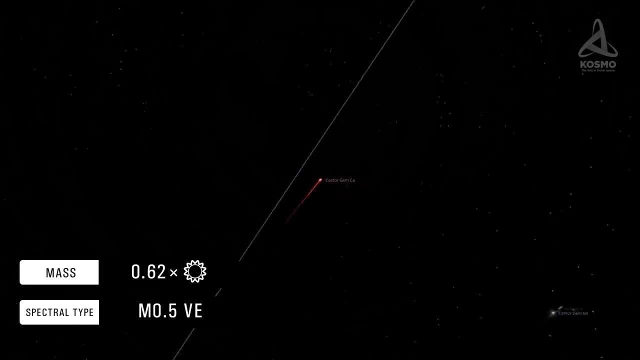 It is a star of spectral type M.55E. Its mass is 0.62 that of the Sun and its radius is 0.76 that of the Sun. That made it the third component in the system, so it was rightfully designated Castor CA. 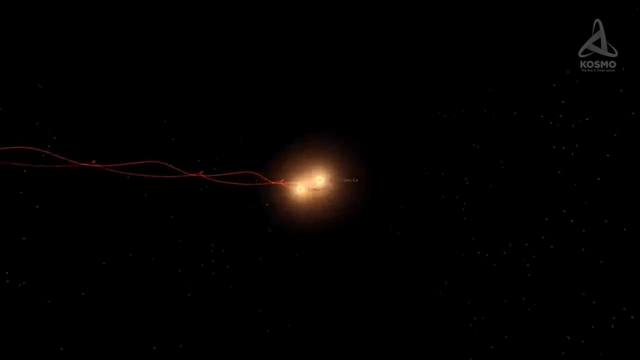 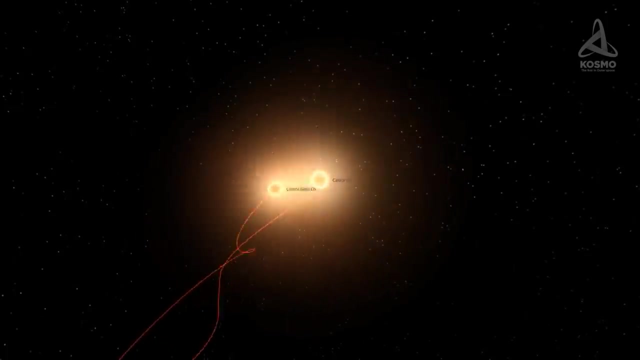 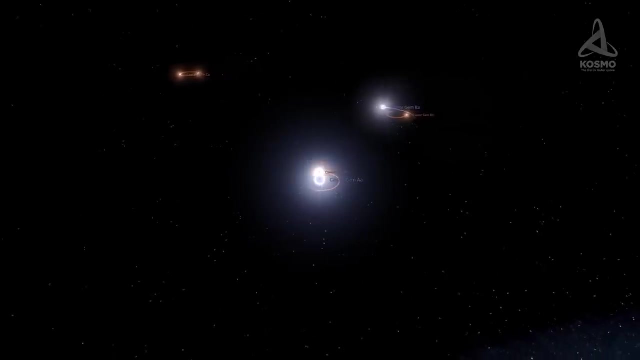 This star follows an elongated elliptical orbit around the system's barycenter. Scientists estimate its orbital period at 14,000 years. As for its location, it is approximately 1,100 astronomical units away from its two companions. Each of these stars is binary, which means that each of them has a secondary companion of its own. 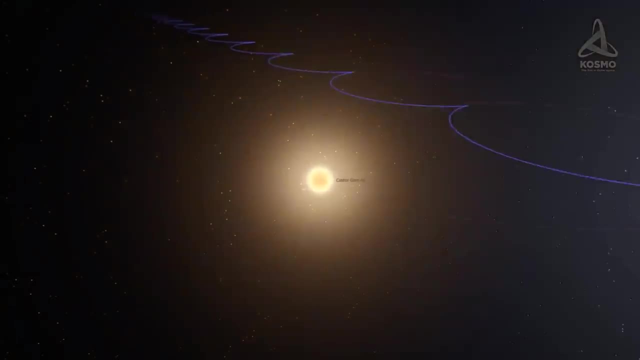 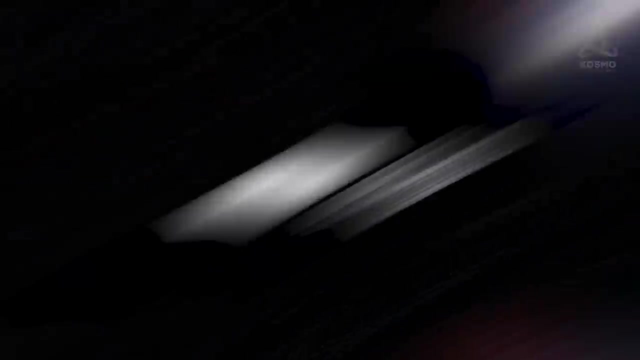 Let's look at them. Castor AB is strongly bound to Castor A, and its mass is about half that of the Sun. Castor BB is a star of spectral type M.25, and its mass is also about half that of the Sun. 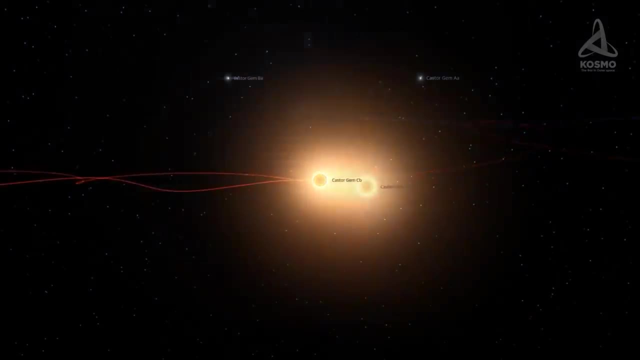 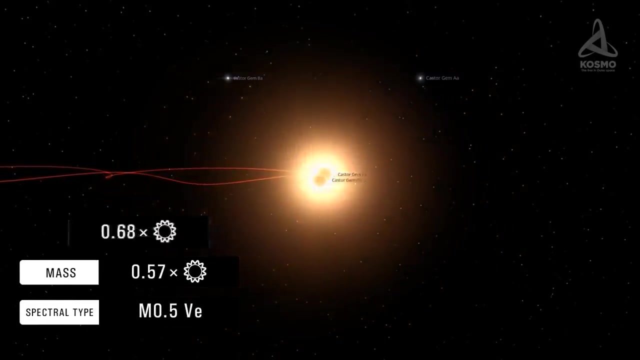 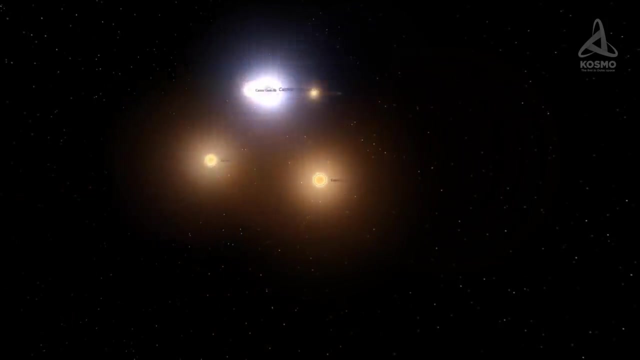 Castor CB is a star of spectral type M.55E and is slightly heavier, at 0.57 Sun's mass and with a radius of 0.68 that of the Sun. Castor CB is almost identical with Castor CA in its properties. 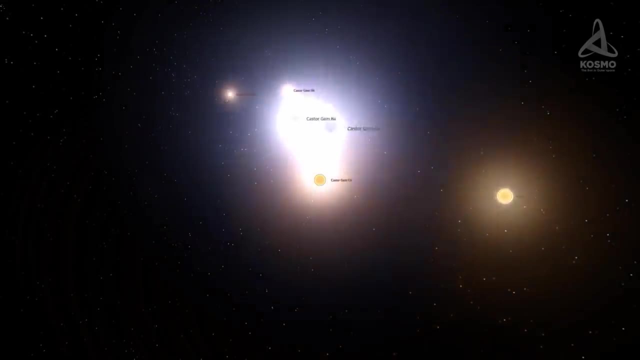 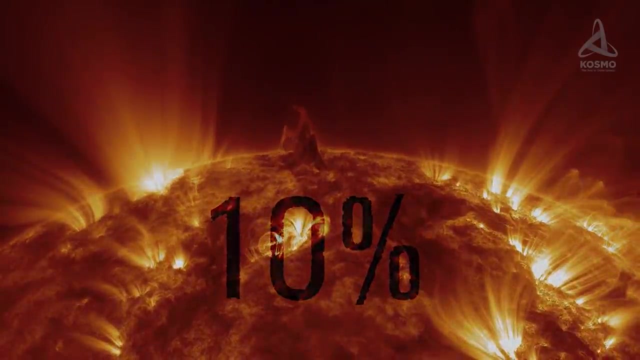 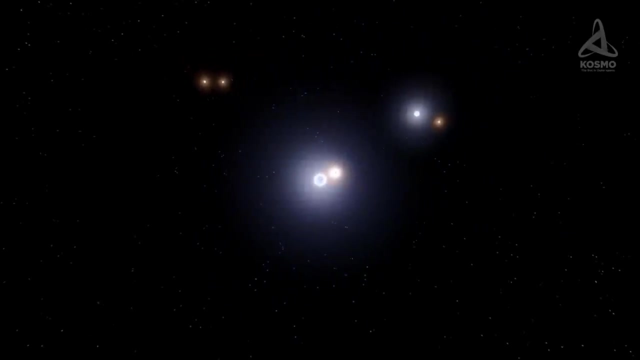 as the surface temperature of both is approximately 3,820 degrees Kelvin and their luminosity is less than 10% that of the Sun. All the six stars orbit around a common center of mass, or barycenter, and their overall luminosity is 52.4 times that of the Sun. 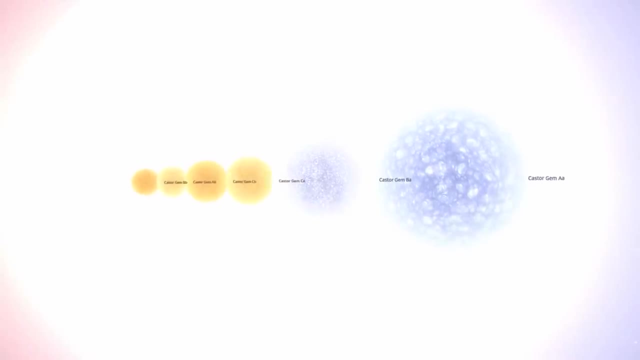 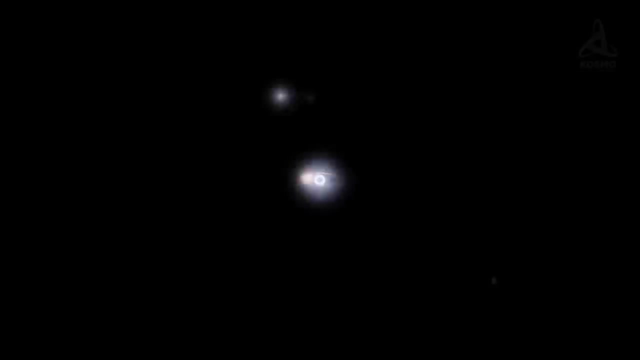 Castor AA and Castor BA are white stars. Interestingly, the former is 30 times and the latter 14 times brighter than the Sun. By contrast, Castor CA and Castor CB are typical red dwarfs. According to scientists, Castor AA and Castor BA are supposed to remain in the main sequence stage. 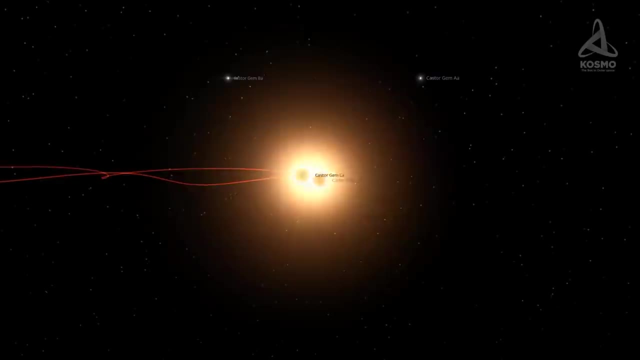 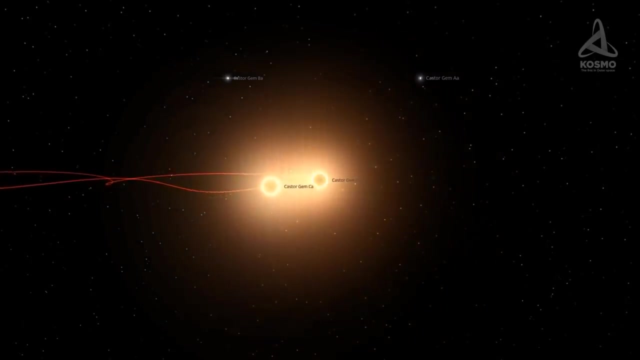 for at least several hundred million years. The red dwarfs, meanwhile, like Castor, CA and CB, have a much longer expected lifespan. This is due to the slow process of thermonuclear fusion of hydrogen, and so they may last from several billion to tens of trillions of years. 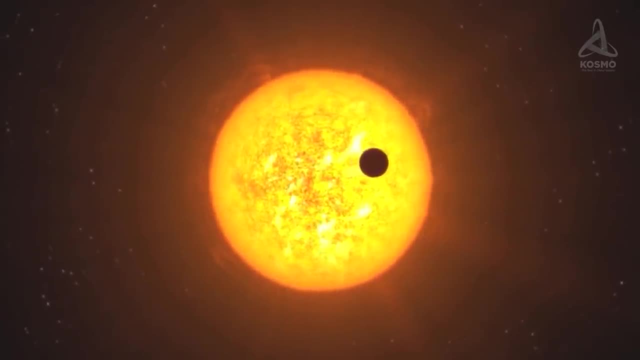 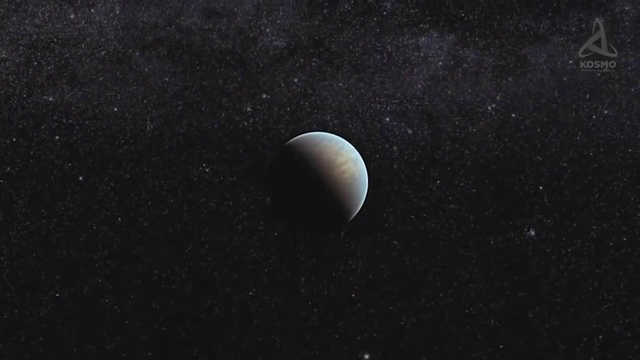 Scientists are currently busy looking for exoplanets in the Castor system. However, so far they have not been able to discover as much as a hint of exoplanets in the system. Perhaps the system is too young to have produced any, or else more advanced methods of detection are called for. 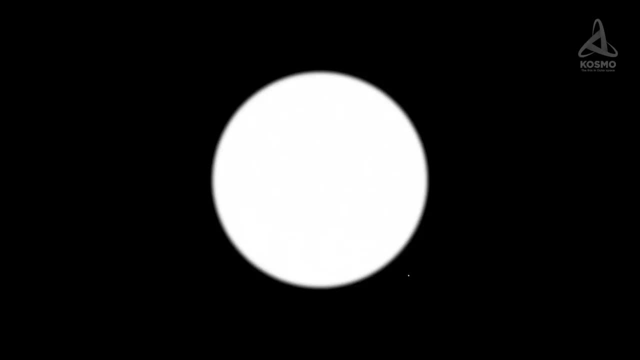 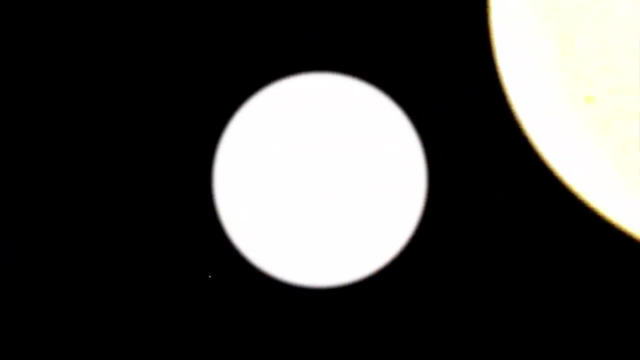 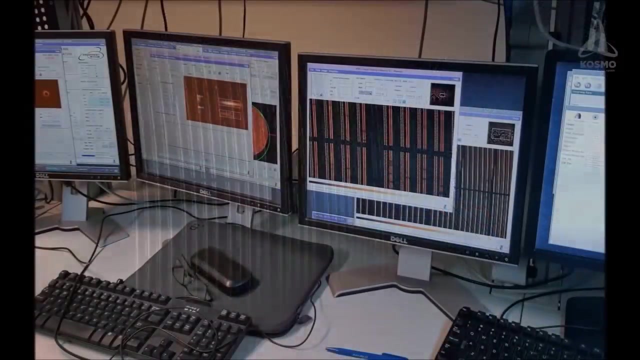 It is too early to speak about other physical properties of these stars. It is quite difficult to study them because they are optical doubles and, seen from the Earth, only seem to be close, whereas it is an illusion. That is why special spectrometers are necessary to take care of accurate measurements. 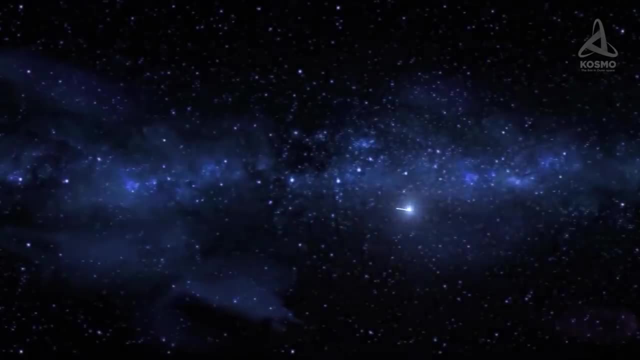 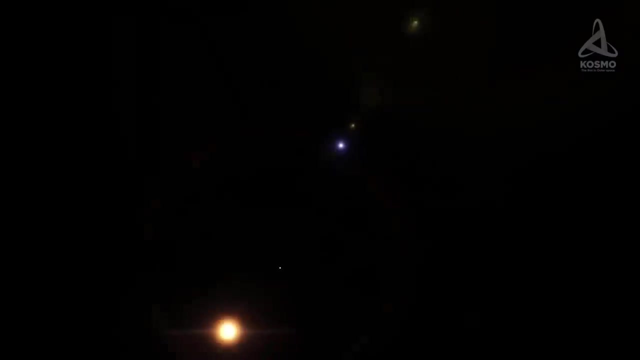 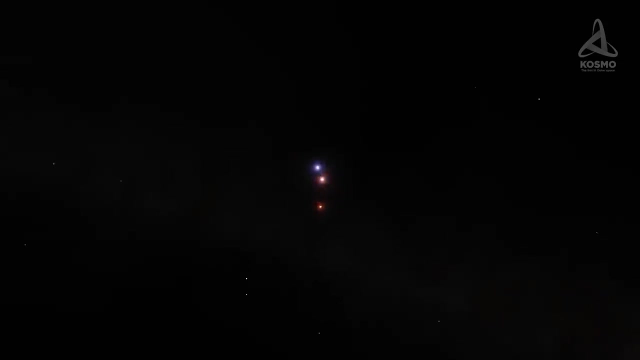 We can see all the six stars from our Earth as a single object, and it is located in the northern hemisphere in the constellation Gemini. The best time to observe them is in winter and spring. It is easy to locate Castor in the sky, as it is bright enough. 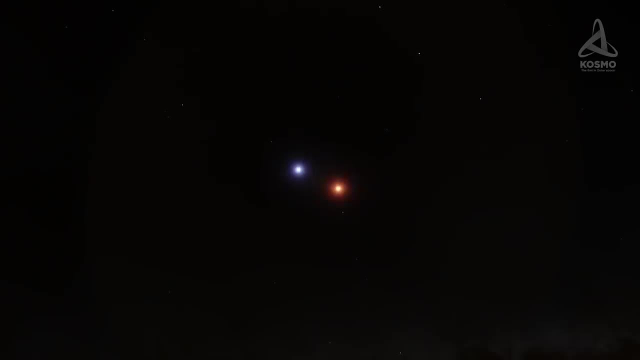 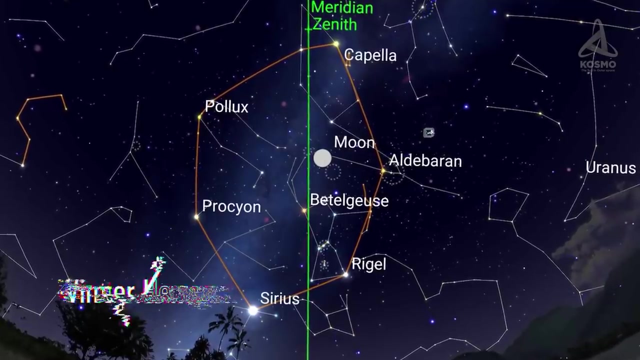 and can be found near a well-known asterism called the Winter Circle or the Winter Hexagon. This asterism is made up of Pollux, Capella, Aldebaran, Rigel, Sirius and Procyon. It is best seen in the night sky in northern latitudes in the winter time. 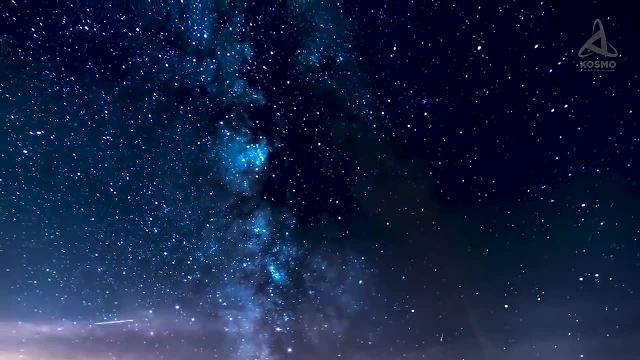 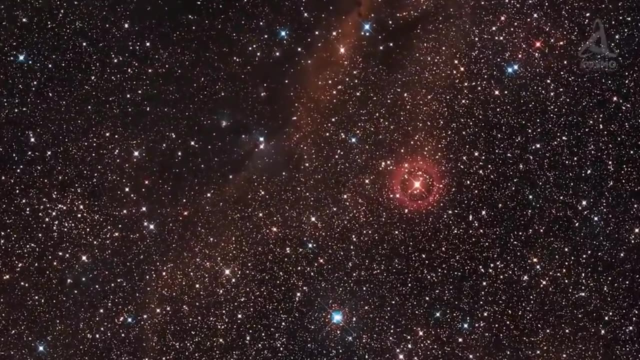 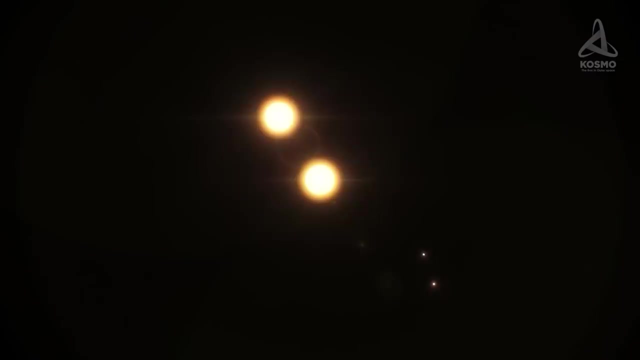 February is the best month to observe Castor and Pollux. It is worth mentioning that Castor is a star system that leads a group of at least 16 celestial bodies. The point is that these stars move together and have similar velocities, and their range is similar. 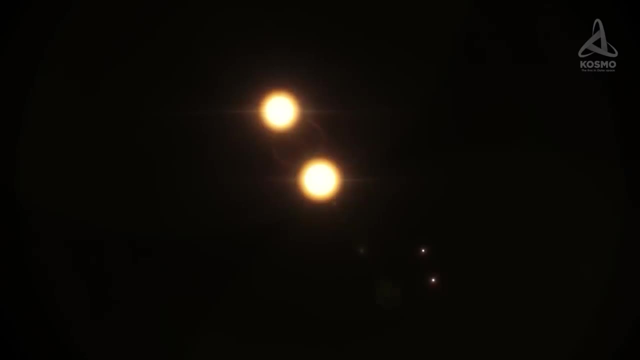 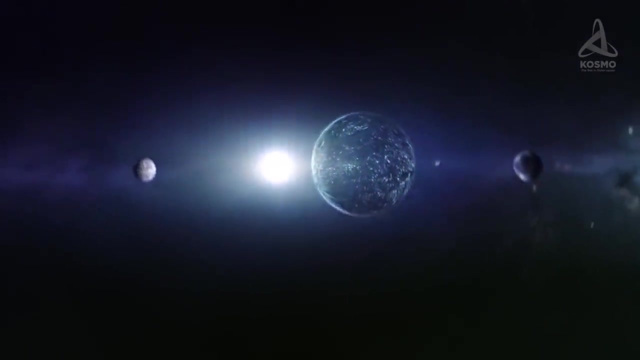 That is why they have been dubbed by scientists as the Castor Moving Group or Castor Stream. It includes such well-known asteroids, astronomical objects as Fomalhaut, Vega, Alderamin, Alpha Libri and others. The question of Castor's stellar evolution still remains open. 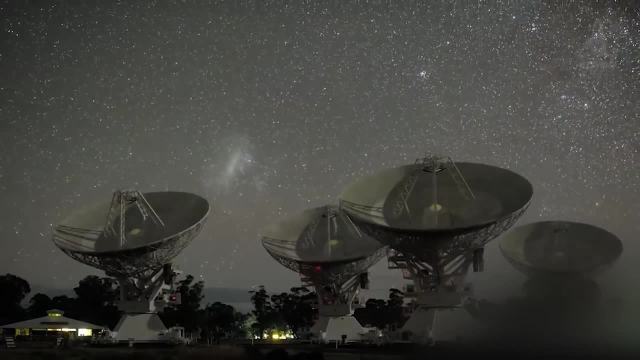 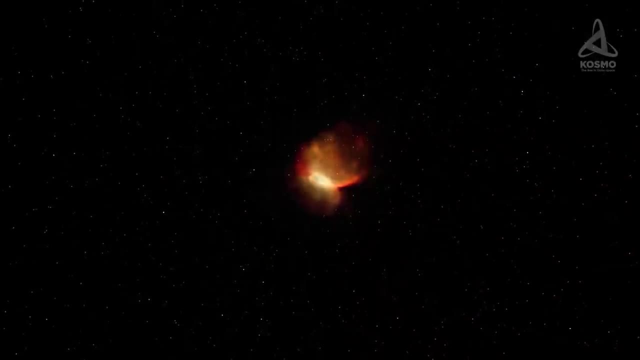 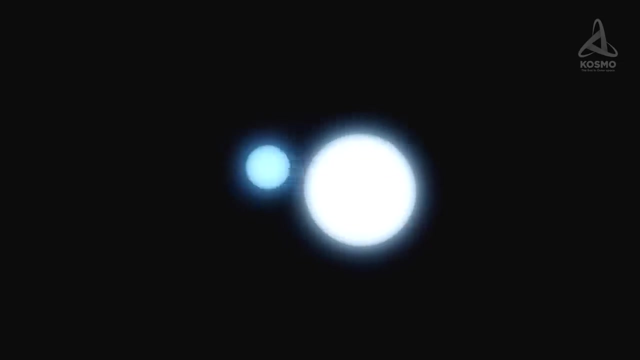 As I have mentioned before, most telescopes are incapable of revealing finer details of these stars as they are too close together as seen from the Earth. According to some scientists, systems of this kind are formed as a result of a big star split into two components by centrifugal force. 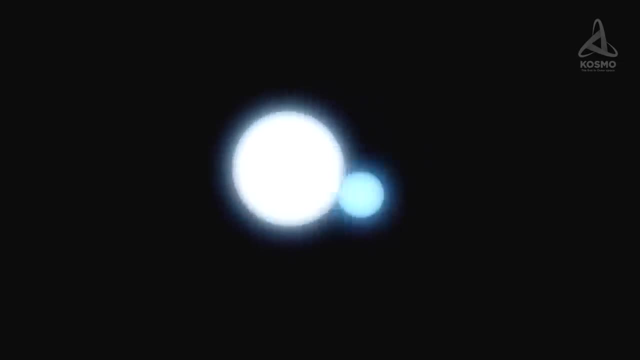 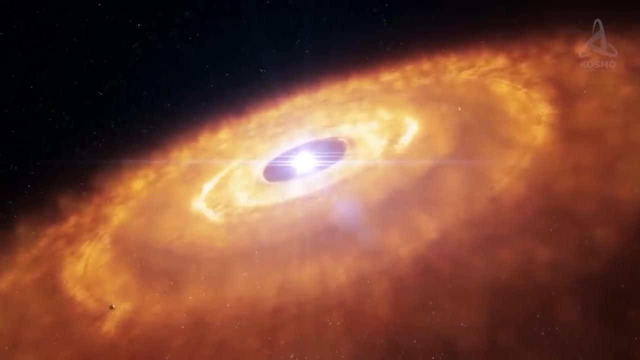 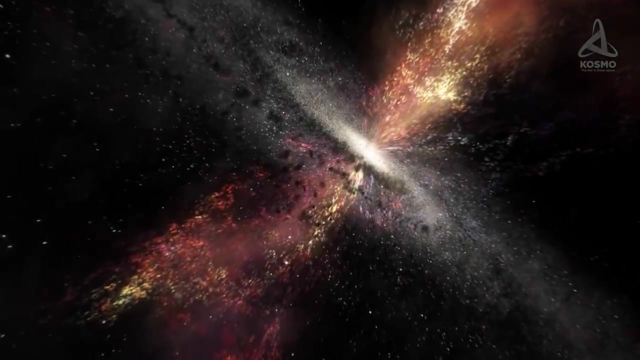 Others claim that they originate when one star gravitationally captures the other. There is also a theory of compound nucleus formation that suggests a molecular cloud's fragmentation, with stars forming as a result. Then there is a theory involving protostellar disks that suggests sudden cooling of gas in a massive protostellar disk. 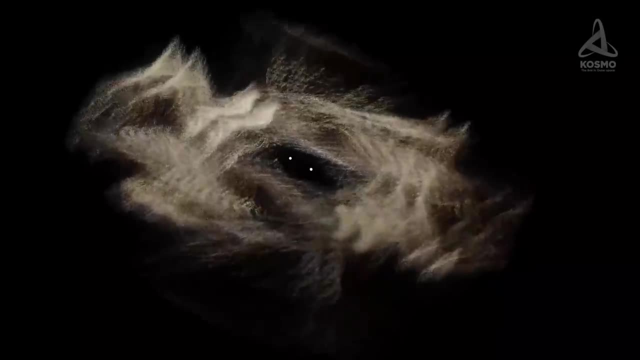 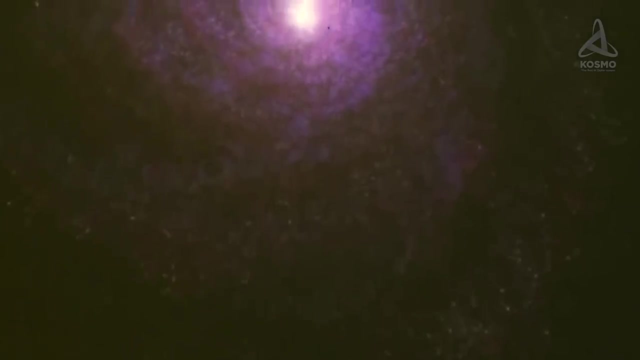 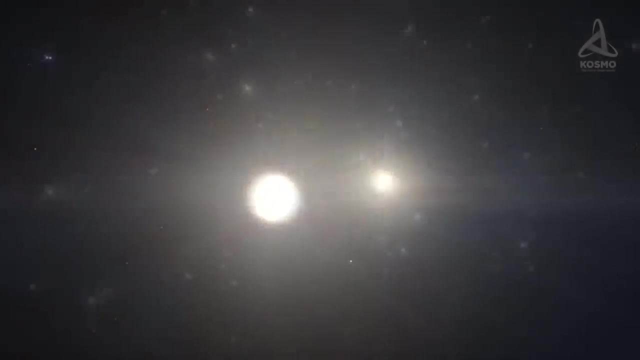 so several stellar companions may simultaneously originate in one and the same plane following the disk's fragmentation. Be it as it may, most facts indicate that multiple systems originate in one place, rather than from scattered sources. In the case of the Castor system, its components are believed to have been formed out of one molecular cloud in the same period. 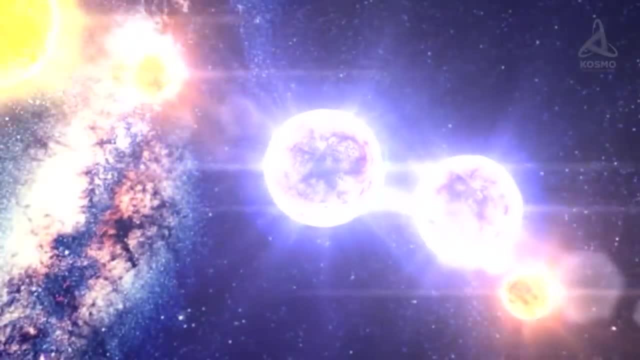 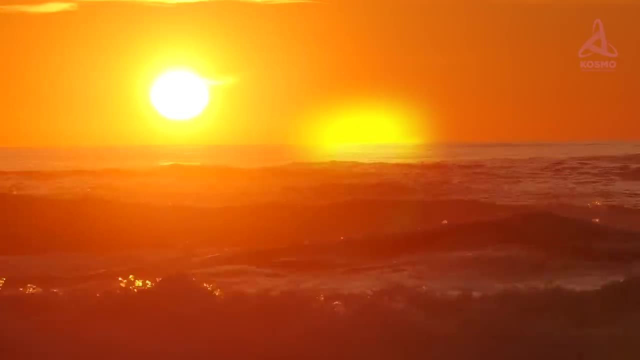 Were a hypothetical exoplanet to find itself in the Castor system, its inhabitants would have enjoyed rather bizarre natural phenomena. For example, the planet would receive light from several stars at the same time, so there would be several suns and sunsets a day. 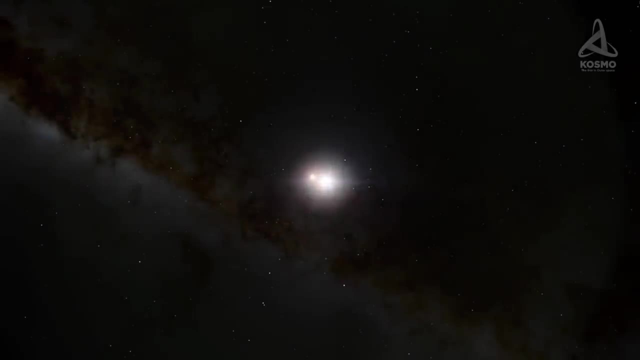 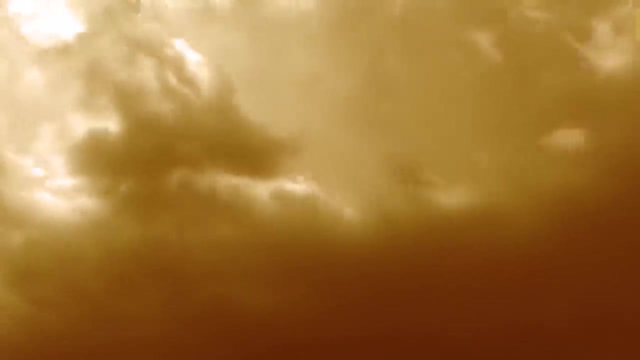 At least it seems bizarre and exotic to us, as we live in the light of only one star. If the Sun had a companion with similar parameters, the Earth would get twice as much heat and light, with all that it implies, and the sky above us would have a totally different aspect. 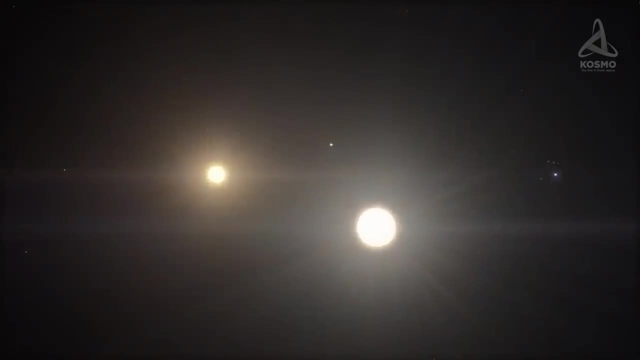 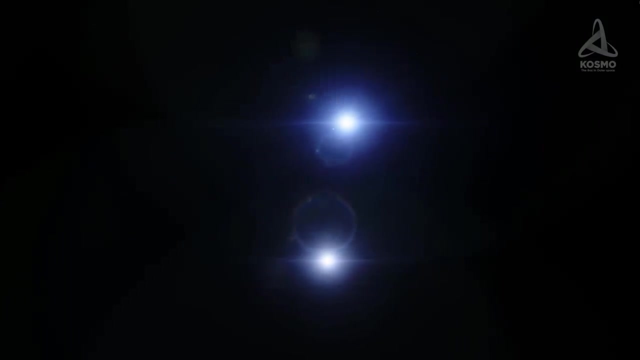 And it is hard to imagine what a sky with several stars, like our Sun, would look like. This mind-boggling sight is straight from a world of fantasy, But that's what we would see if we were to find ourselves in the Castor system. 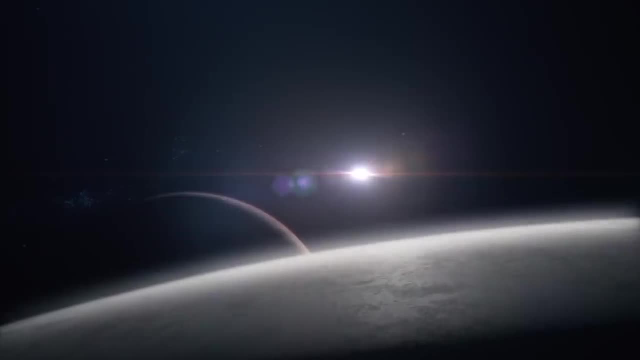 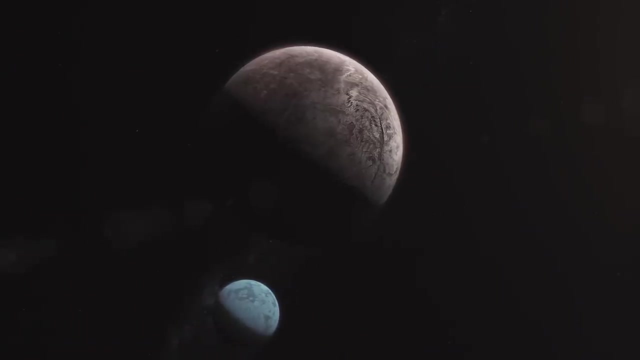 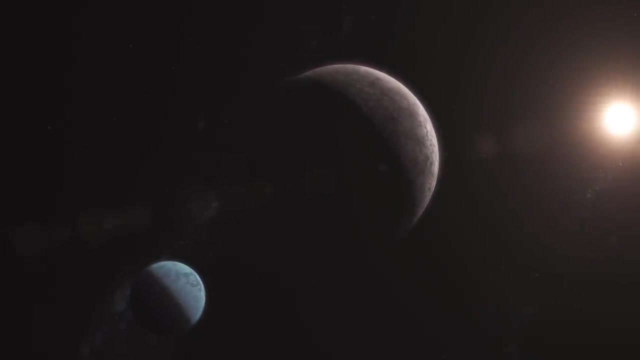 In this film, I have told you about many notable exoplanets. Still, our trip was admittedly quite brief. To cover all the fascinating worlds mankind is now aware of would literally take infinite time. Even as we speak about them, the rate at which we get information about them grows incrementally. 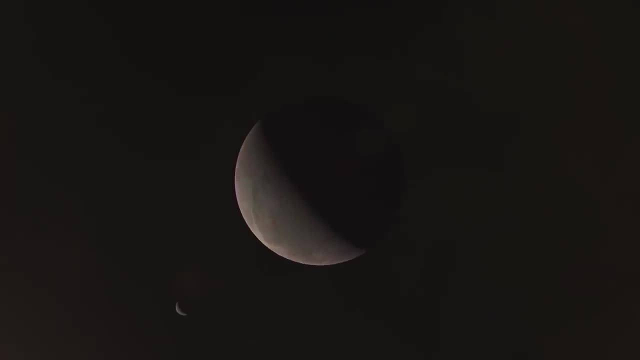 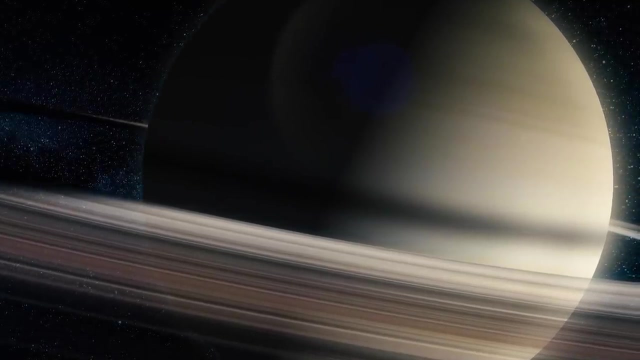 It is these unusual exoplanets that draw the attention of the entire scientific community, And it is these celestial bodies that will become new objects of more detailed investigations and research, And so we'll definitely be getting back to them in our new videos to bring you the latest updates.